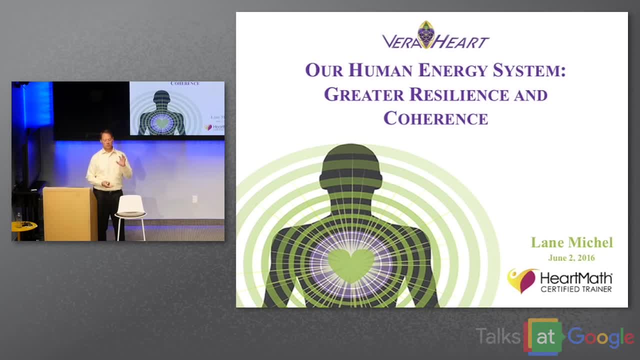 When I started VeraHeart a couple of years ago, it was really with the idea that this was the time to advance mindfulness and what I was calling heartfulness in business, but in our personal lives as well, And that led to building or searching for best materials. 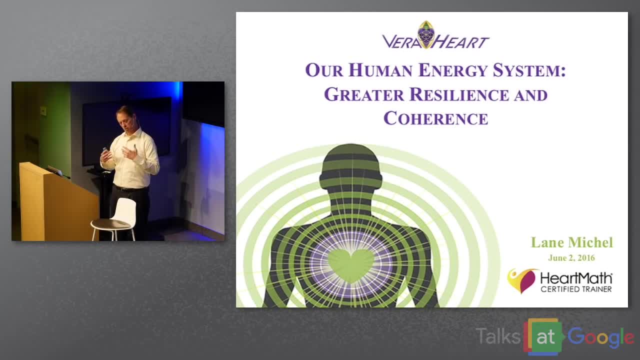 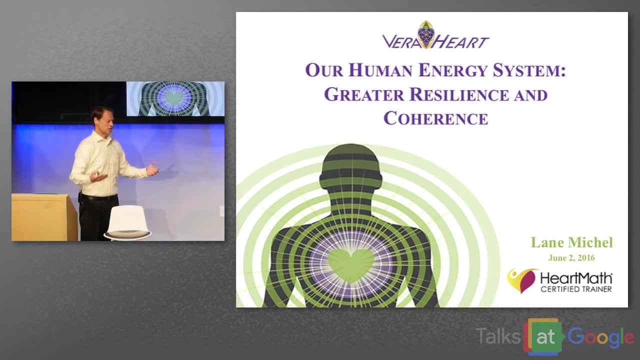 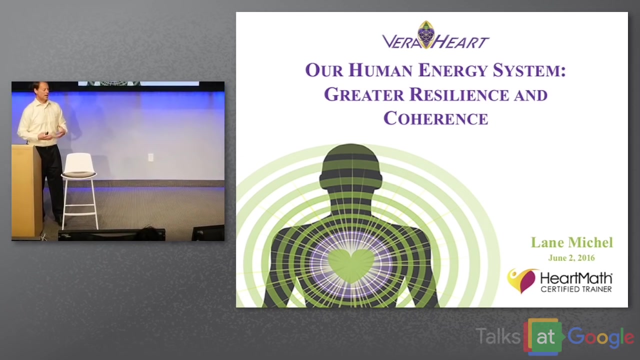 for empowerment, for supporting choice And for supporting being more in our own energy And extending that to organizations so that organizations could become energized- And VeraHeart's tagline is about developing energized people and companies- This whole idea of opening up the energy that we have. 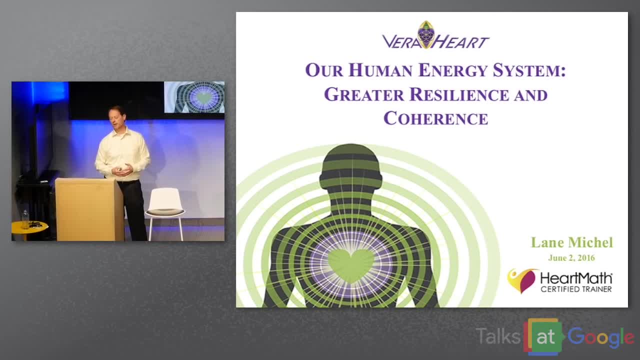 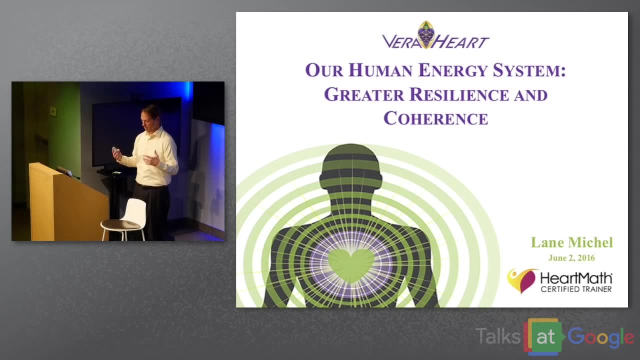 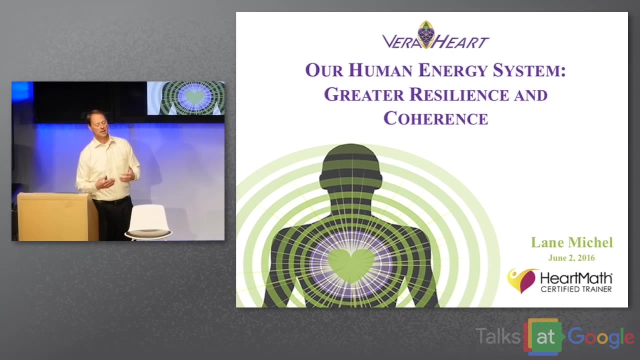 unleashing new potentials- a very exciting time right now. The part I want to share with you in this, I believe, is that this segment is about human energy, our system and how some biofeedback tools, the research and science behind those, is helping to improve. 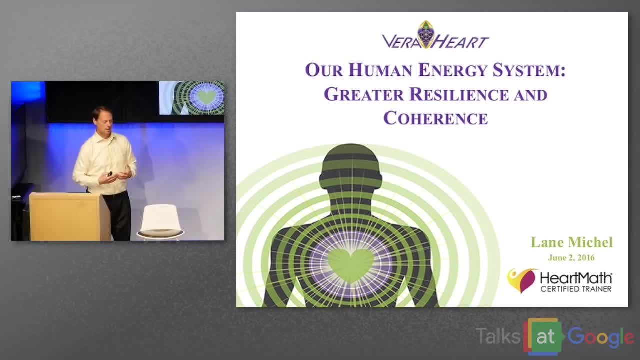 how we can access more of our energy, build more of our energy and, frankly, achieve more as well, both personally and as organizations, come together, using these practices as a team. So that's where we're going to focus on those elements today. 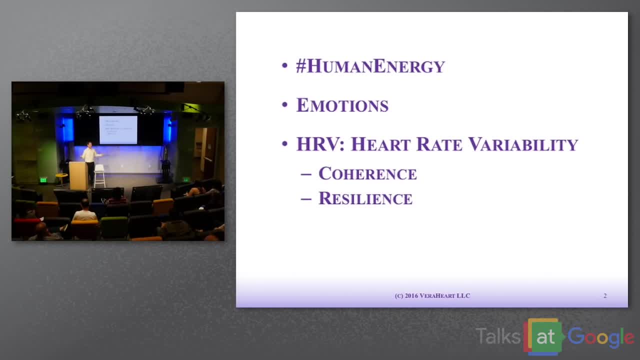 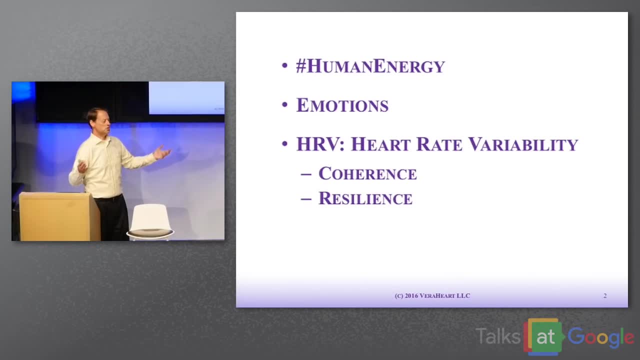 First of all, so hashtags. I go out and search for anything to do with energy and people And what do you imagine that I find? It's oil, petroleum, it's solar, it's. you know, the idea of we as a human energy system is just about. 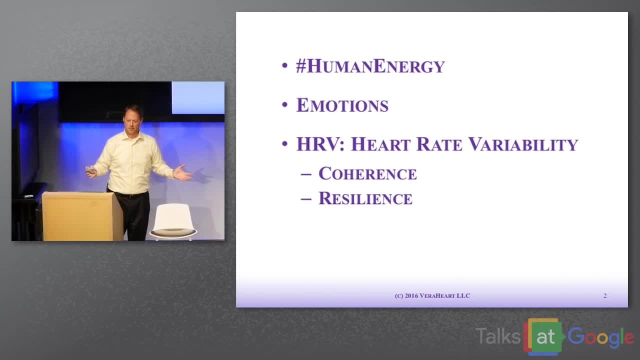 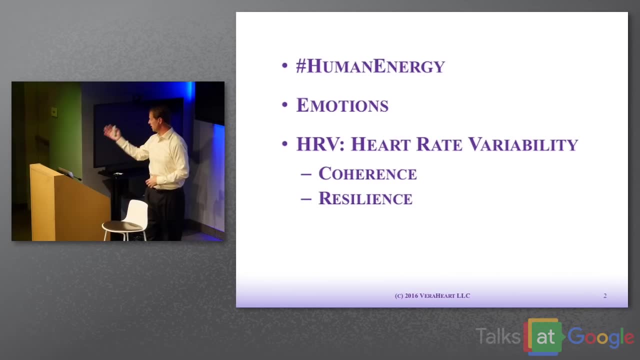 non-existent, still out in all the social media. So let's launch it, Let's get it going. So, hashtag: human energy: We're going to start drawing all this stuff together. everything GPOS is about, We're going to pull together the ideas that we are energy systems. 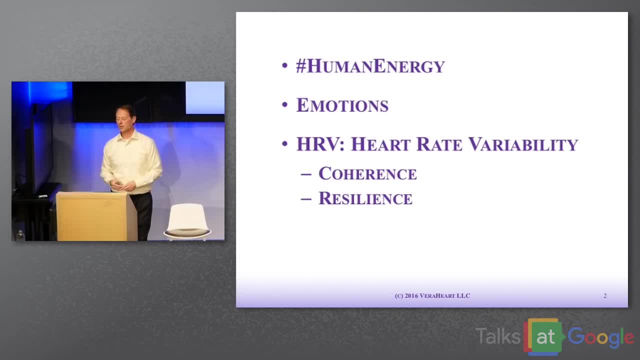 And I'm going to touch on a couple of important aspects with us as human energy systems related to this topic of being able to move with mindfulness and heartfulness and increase our energy. Necessarily, we've got to touch on emotions. You go ugh, emotions, ugh. I don't want to go there. 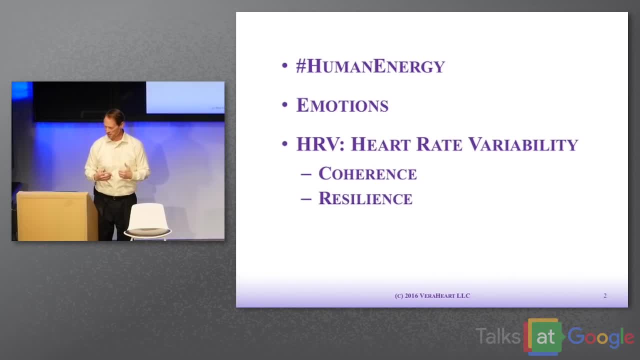 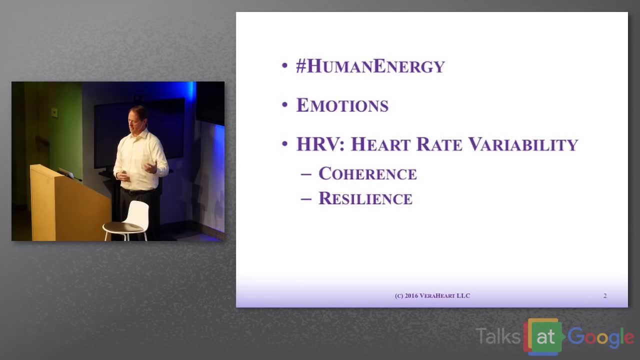 And the reality is that I speak from experience, not wanting to be there. having been an engineer- And I had a great career with Hewlett Packard- went into consulting. You can imagine high tech and then management consulting. there's not a lot that you do with emotions in there. 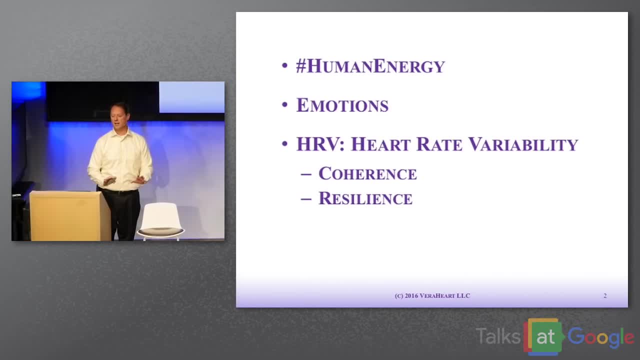 In fact, if anything, keep it out of the way, Don't go there. And the reality is that along the process I've learned the role of emotions, I've learned how those relate to energy systems. So I'm going to share some important points with that too. 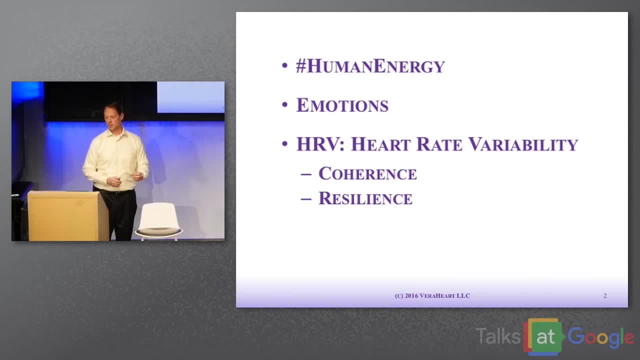 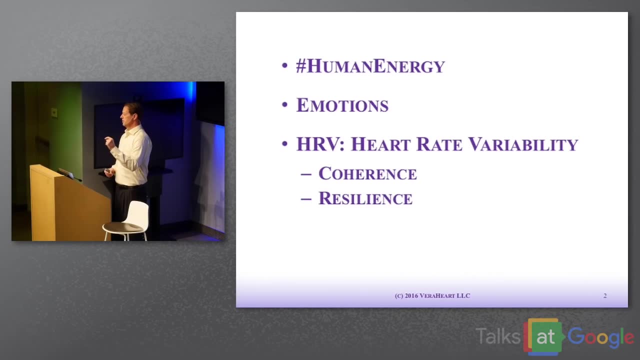 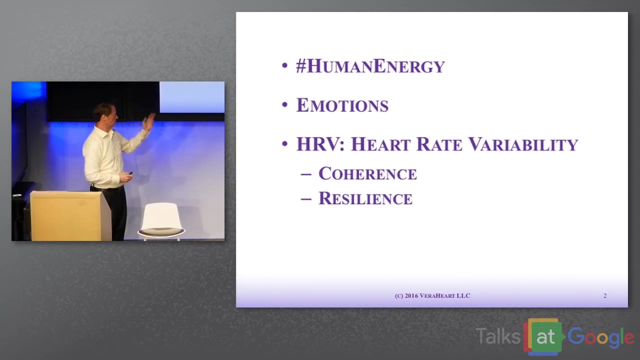 And then we're going to get into what science, research, has shown as really what we believe is the most valuable tool for being able to manage your energy system intelligently: manage your energy, direct it and be able to build more. So we're going to touch on heart rate variability. 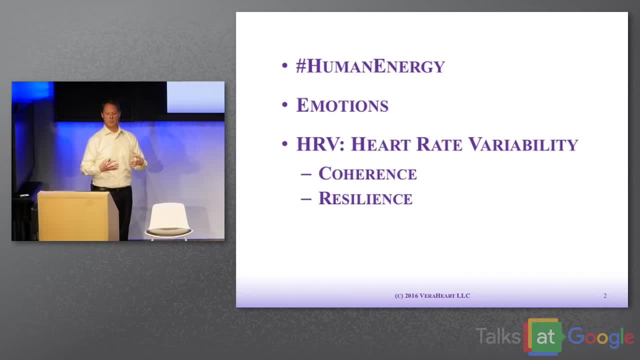 That is the key metric, the key biofeedback determinant, And we're going to demonstrate heart rate variability used to be able to raise energy and deliver coherence and resilience. Now, those may not be different words than you've heard. They won't. 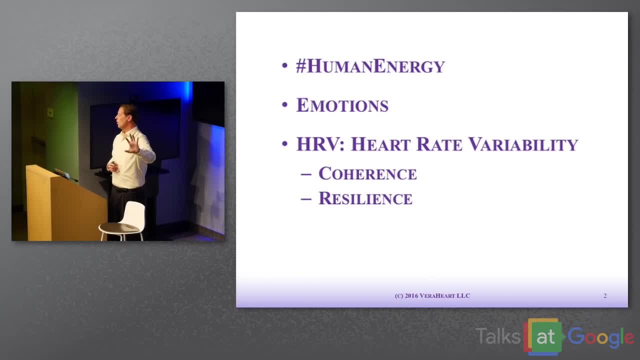 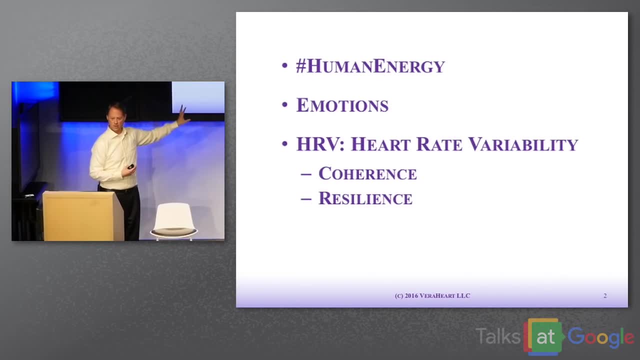 But how they're used and how they're going to be used is we all go forward in managing our human energy is very, very important. So I'm going to help define those And then we're going to put those into practice as well. 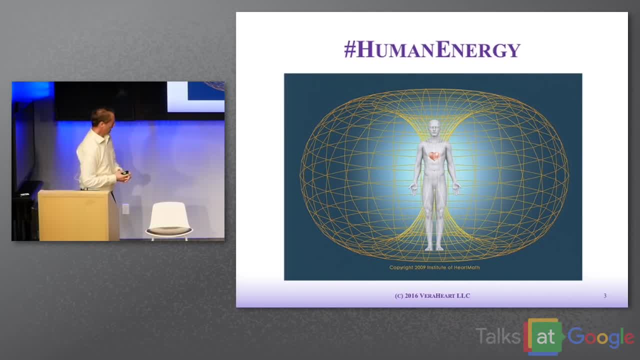 So human energy. Let's start with the idea that, first of all, we need to be able to manage our energy systems. Now, there certainly is human power, which is our kinetic abilities. We can move things. We move. There is our metabolism and the energy in our system. 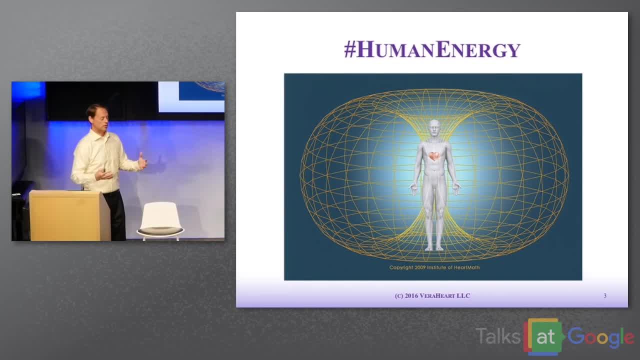 the power that we have in our system itself. We actually produce electricity. There's actually interesting science going on right now: all the matrix that maybe we could be our own battery. Having matrix is the movie still prevalent in everybody's minds, But we do produce electricity. 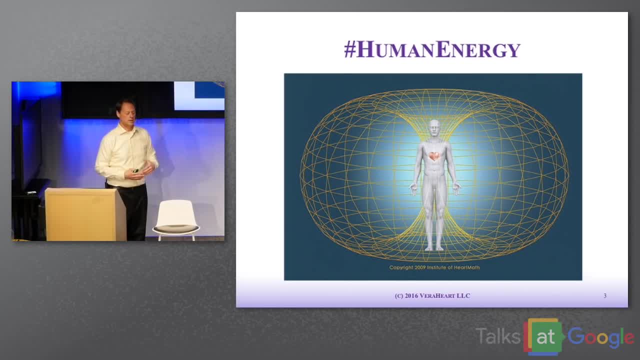 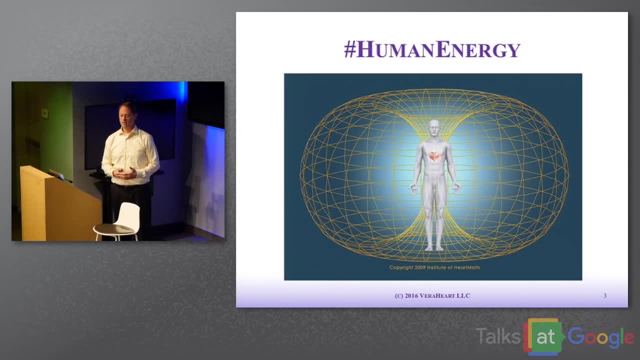 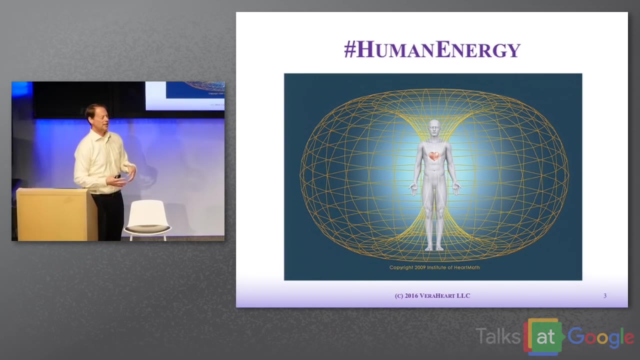 Maybe only four watts, but maybe there's a way to harness more of that. In reality, what we think of is the energy and the power that we typically understand that we have. it's depleted, It's used, It's inefficient. We have more heat in the production of energy. 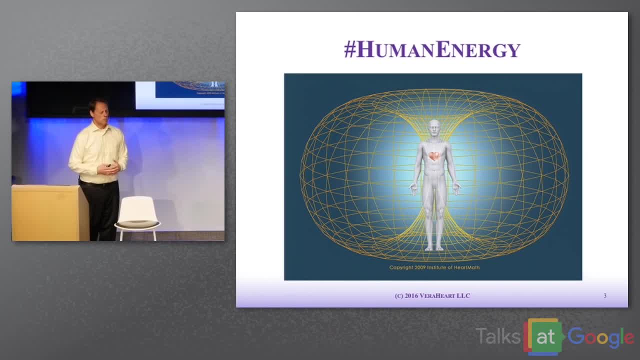 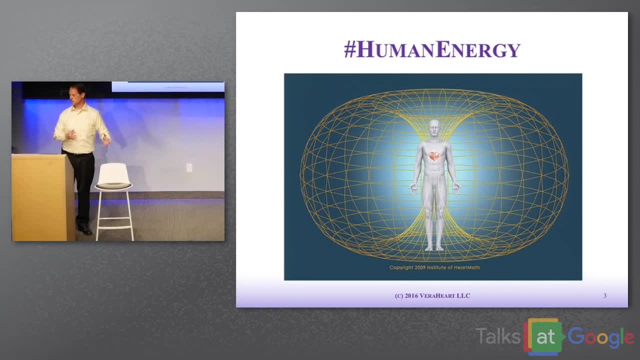 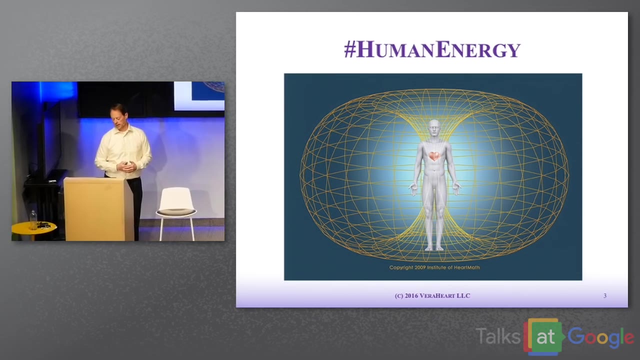 that is, heat loss and so loss of energy. Most of the time when we talk to people about human energy, it's about the loss and the inefficiency of our system and losing energy, And the reality is that we're going to turn that upside down here. 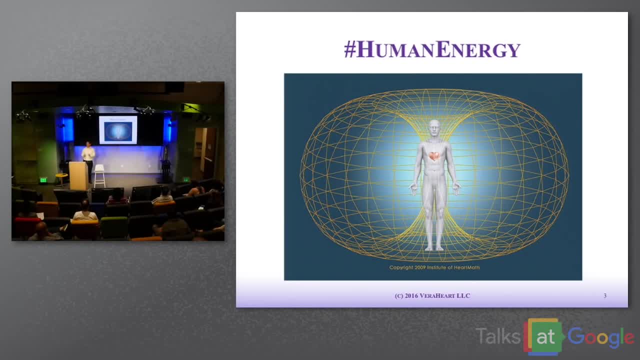 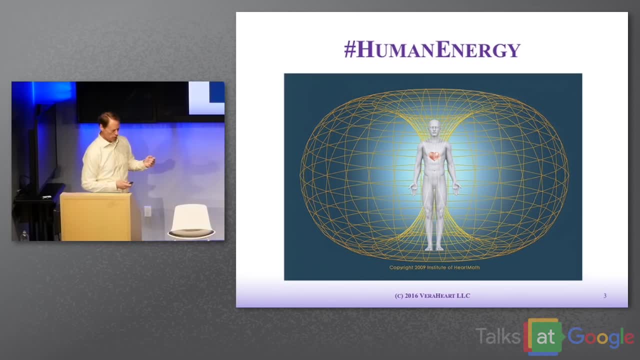 Because what we have to recognize is that, as humans, we expend and renew energy all day long, And in that process we're going to have two important aspects that you may not know about that science has covered. One is that we have the ability to produce energy from our heart. 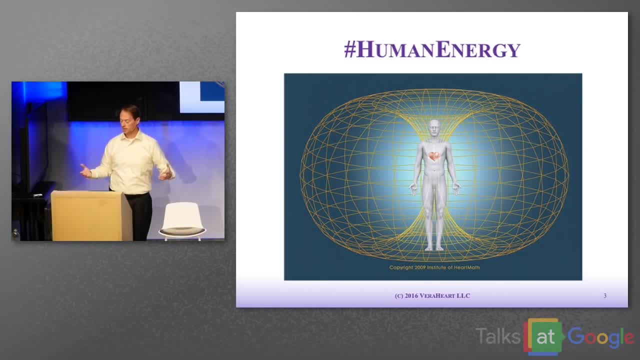 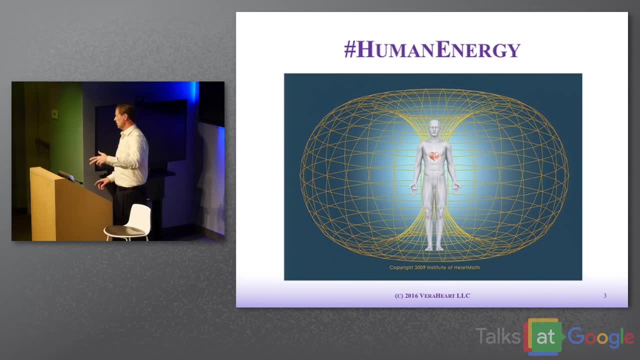 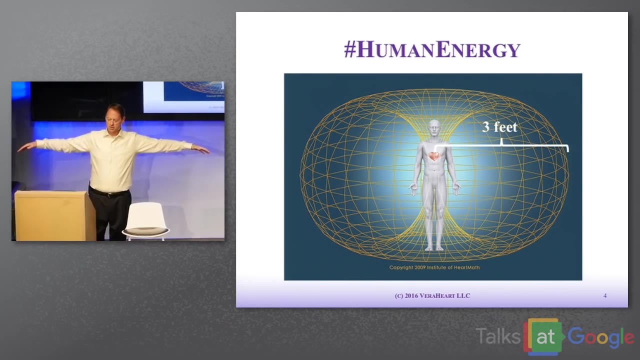 And we have a heart field, an electromagnetic field of our heart. This is a computer-generated model representing the heart field that has been measured with magnetometers. That heart field extends three feet out from your body, So what I want you to do is just reach. 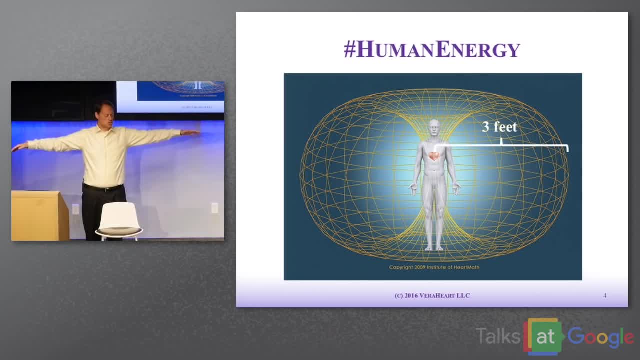 your arms out, go ahead, intrude on your neighbors. Now, that's a little bit less than your heart field that's generating right now. How is that? as everybody's arms were over each other? Well, the reality is all of your heart fields. 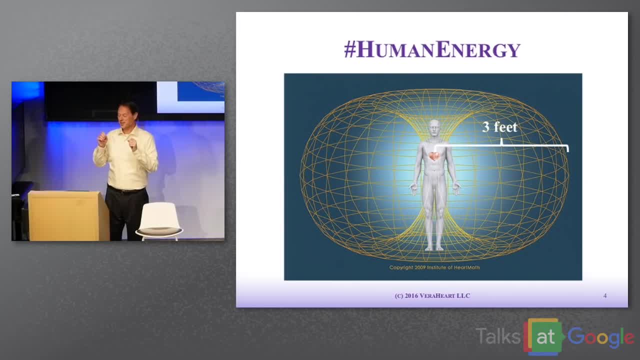 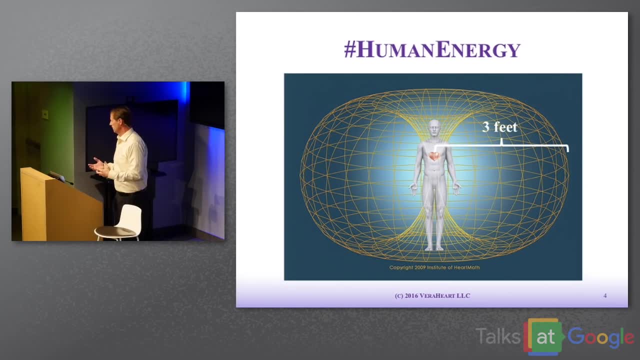 are intermingling as well, And we're going to come back to that point. Your heart as an electrical device. as your heart beats, it is creating an electromagnetic field, And that is this three-foot field, And there are other devices that measure it much, much wider. 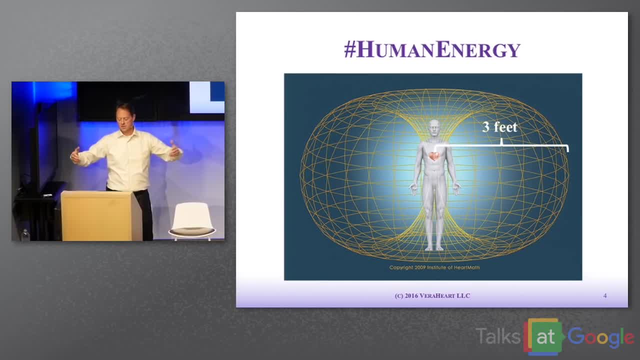 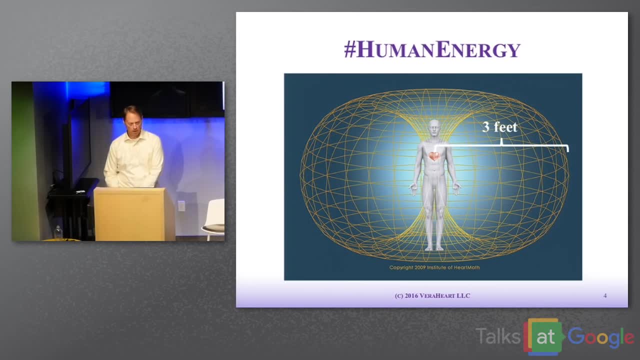 as well, But let's stick with that- where the science is behind this magnetic field, this electromagnetic field that we have of the heart And the idea that your heart continues to beat in producing that field. And we're not talking about auras or more esoteric. 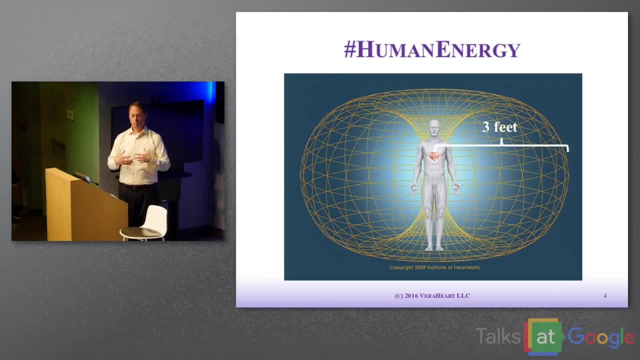 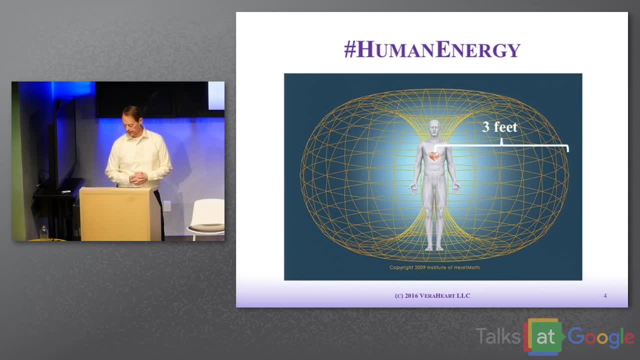 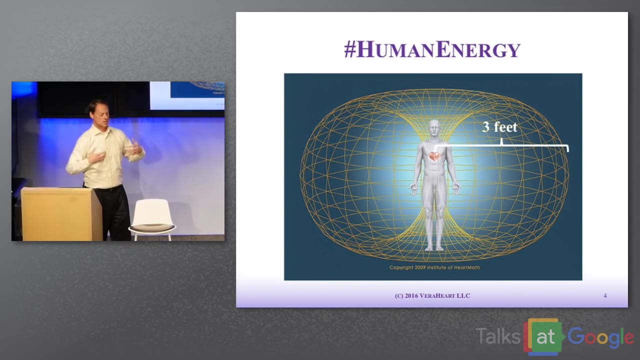 or Eastern belief in mess. We're talking about real, measurable electrical field. We're talking about the electromagnetic field that you have, we all have as long as we're alive. The other thing is think about this energy that's being produced in this electromagnetic field. 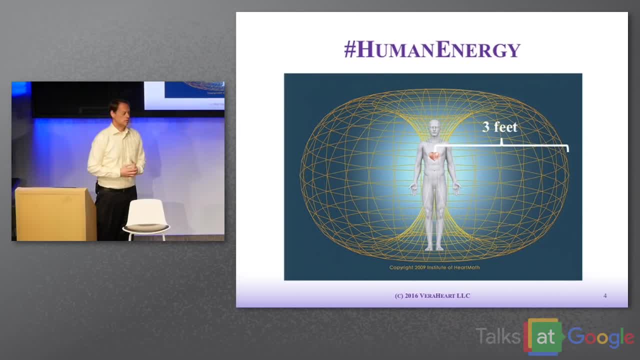 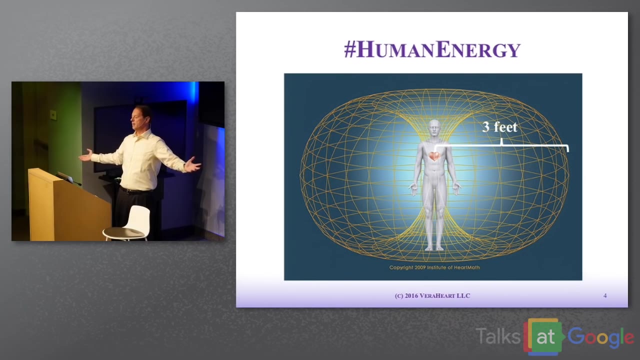 that you have. It's a carrier wave. It is a carrier of what you are experiencing through your heart, And what I'm telling you is that your intentions, thoughts and your emotions are carried as messages through this electromagnetic field. What do I mean by that? 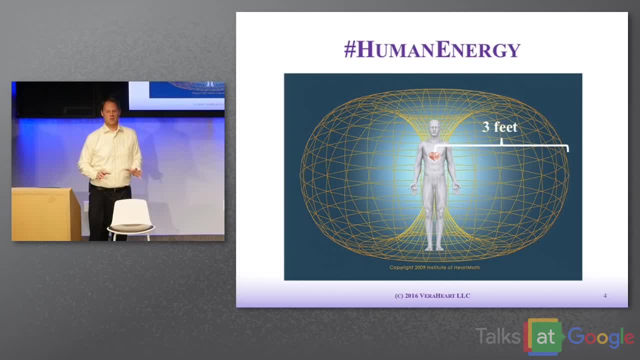 Have you walked into a room and felt kind of dread or like this is icky or not this meeting again? Well, that could be other reasons, But have you had that experience where you just don't want to be in that spot? 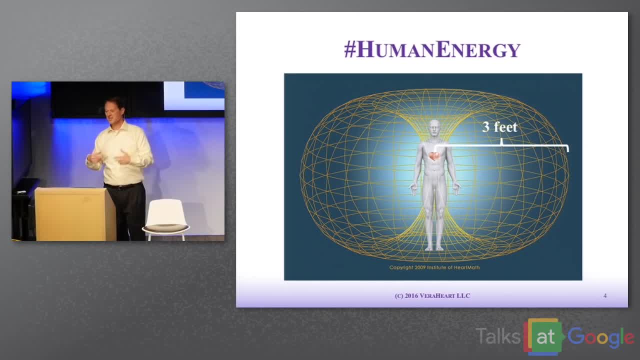 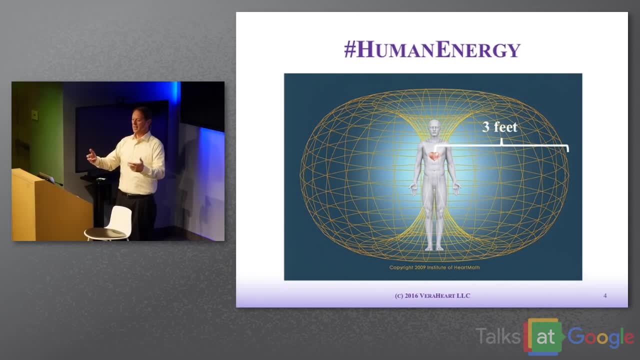 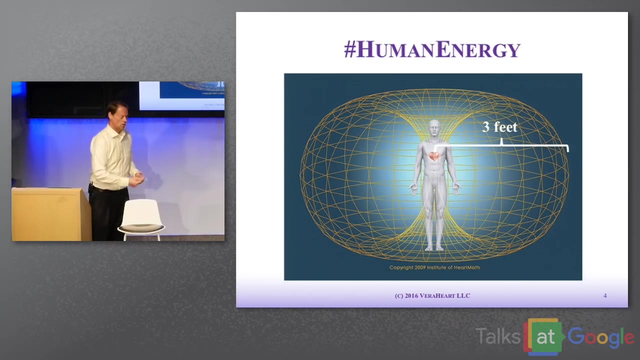 Well, what's happening is you as a sensor in this electromagnetic field. you are receiving information, But you're also transmitting information as well. If you have been in a place where it was feeling down like that, and somebody walks in and they shift the energy in the room. 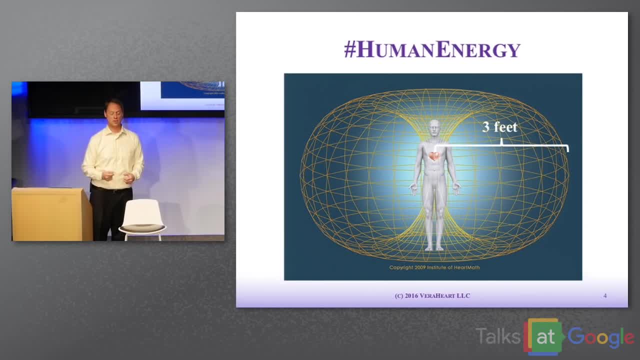 or you walk into a room and the energy feels very different and you're lifted. what's happened there? It is this whole interchange of this electromagnetic field, the heart fields, that is at play here. It's a real and tangible sense that you have. 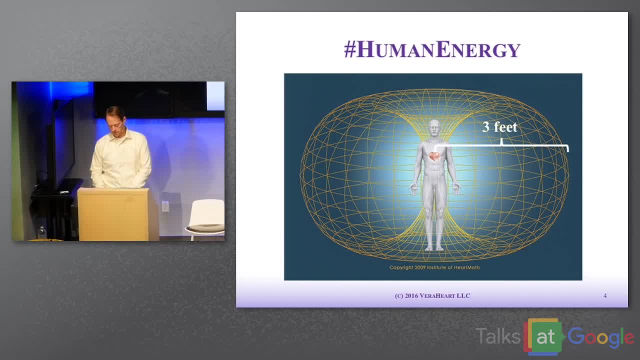 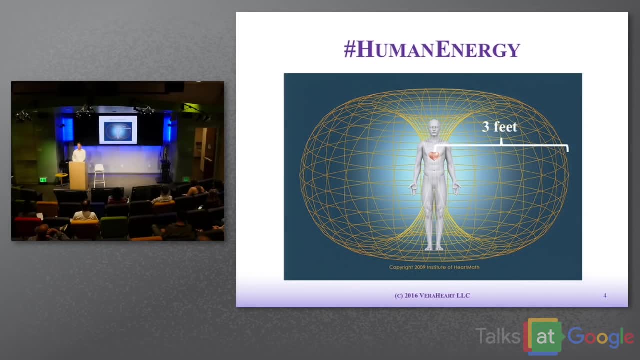 It's a tool you have as well. It's part of your humanity, It's part of human energy, And science calls that, by the way, a coherent field effect. that is real and measurable The more that we all synchronize and we're. 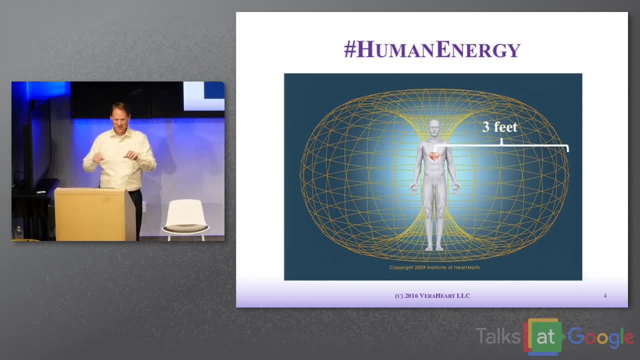 going to do some work. the more we all synchronize and our heart fields become coherent, that coherent field effect creates that environment that is a positive and uplifting environment. A lot of mindfulness practice in the meditation or the breathing, the work of mindfulness itself is even feeding. 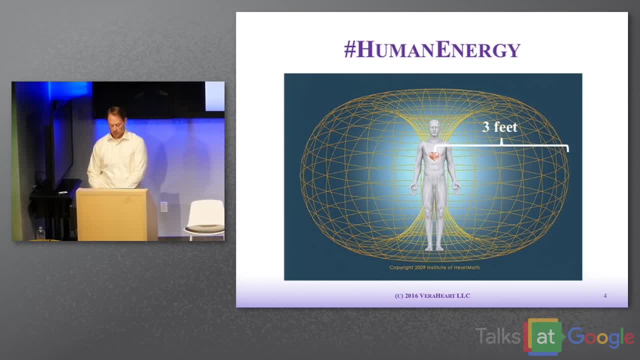 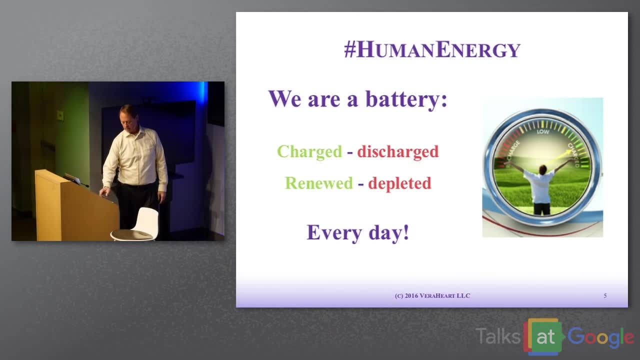 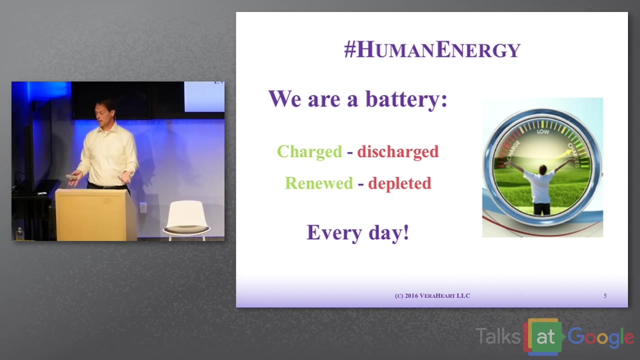 It is feeding this coherent field effect, So we're going to build on that as well. So electromagnetic field three feet from you. The other thing with human energy to touch on is that I mentioned you're a battery. You really are. We're all batteries. 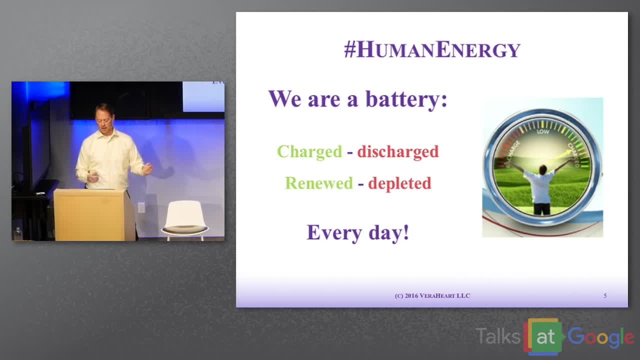 What do batteries do? They charge and discharge. In the case of the battery, what we're talking about here is renewing and depleting all day long. So what are some of the things that we are renewing with? Well, the biggest one, we're supposed to renew and regenerate. 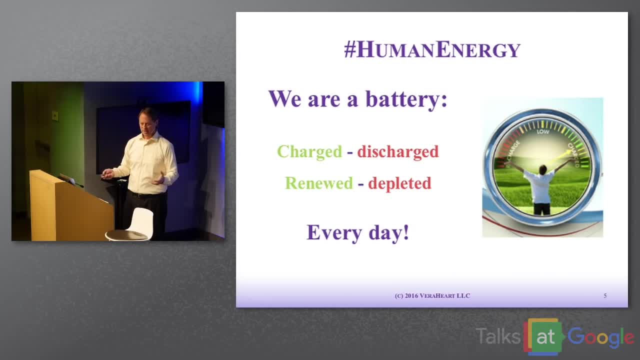 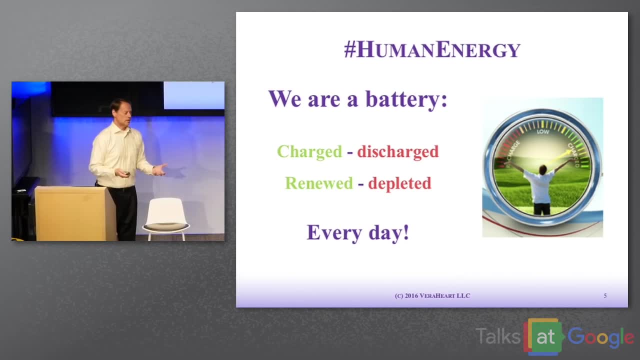 is with sleep. Our sleep cycle is the biggest regenerator that we have of our human energy. If we're not getting sleep and we sustain sleeplessness, you never get ahead of having enough energy And you get towards the end of the day. 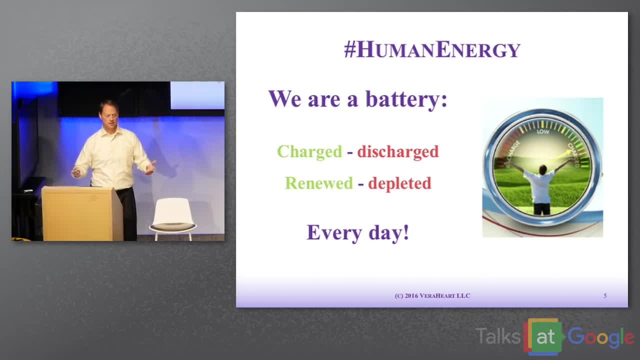 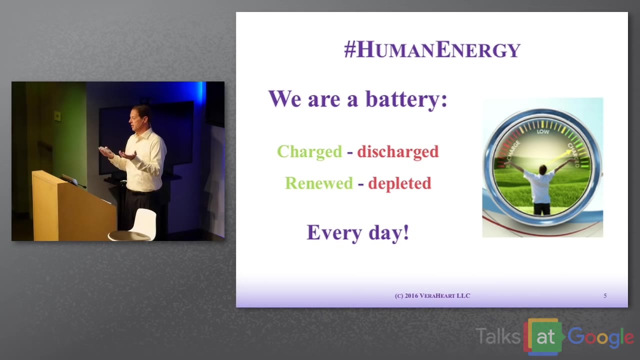 and you just don't have enough left Right. So another generator, though, is the practices that we can do that, through our heart and through our psychophysiology, are able to produce and lift energy, to draw more energy in as a part of our human energy system. 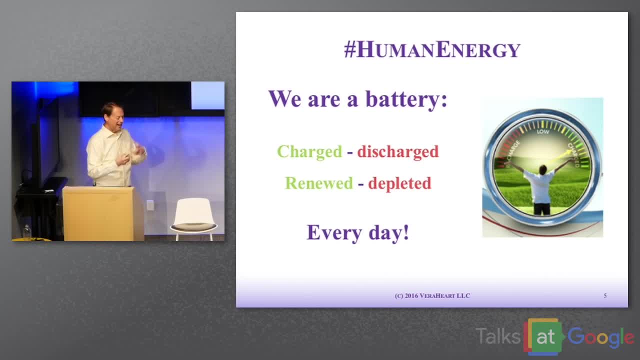 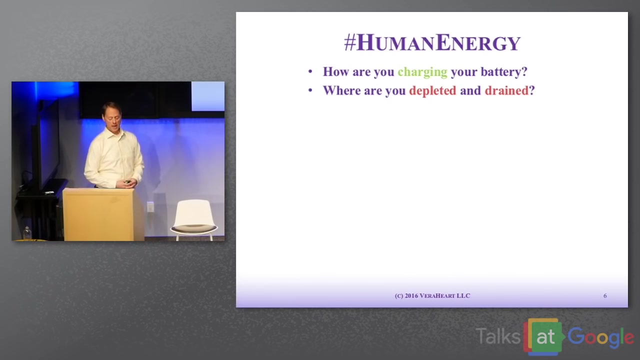 And so that kind of work is facilitated through the devices that we're going to demonstrate today, the practices That we can do that allow us to harness breath as the number one tool for being able to produce our energy, So as a battery. think about these two questions. 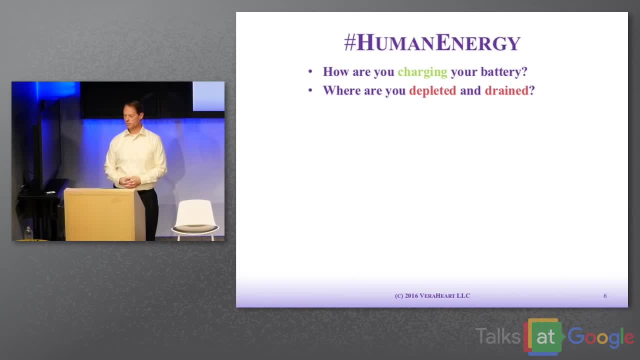 Each day. right now, you can think about: how are you charging your battery? Are you getting enough sleep? Well, maybe not Right. Are you having broken sleep If you start with sleep and sleeplessness? sleepless disorders are a big reason for our discharge. 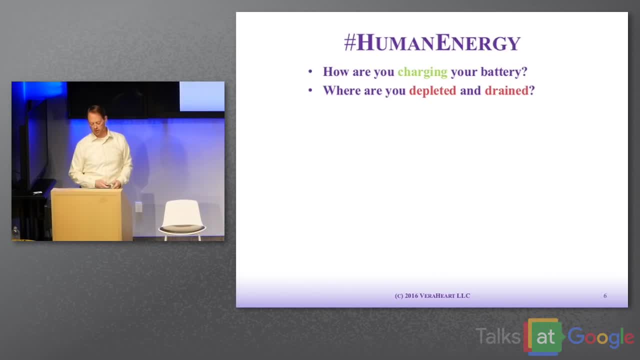 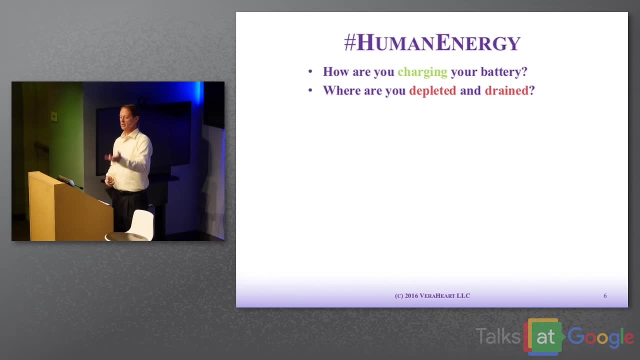 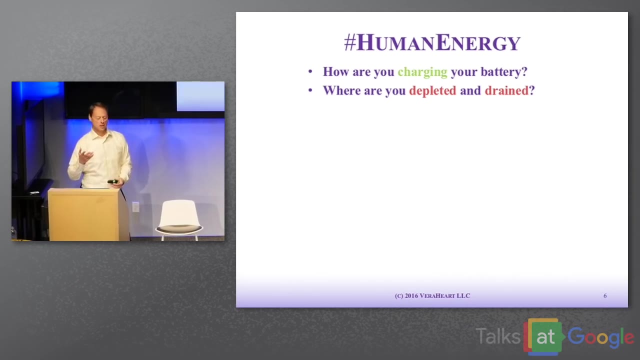 and our inability to bring up that battery. bring up our human energy and our potential. Are you doing things that allow you to take a break? Are you getting into nature? Are you finding the ways that you're able to charge your battery? There's something that we're going. 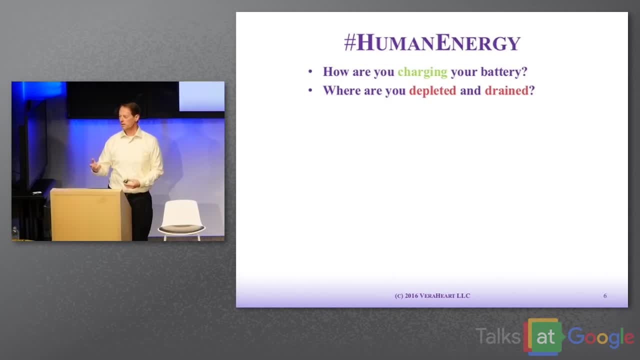 to talk about here, about appreciation and compassion and care, accessing that. It turns out to be a big lift of energy as well. What about depleting or draining? What's going on that depletes or drains your battery? If you allow the first two or three thoughts to come in, 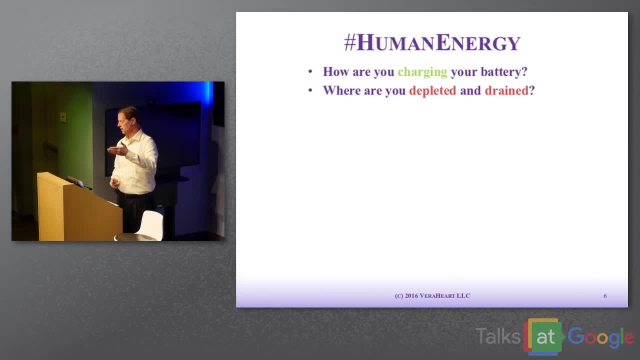 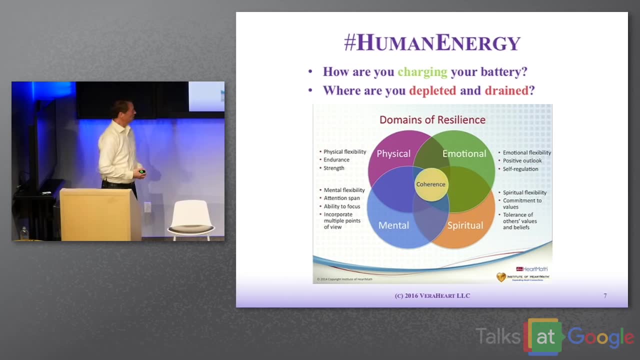 I would pretty much guess that something emotional is in that list. Something's happened that is draining your battery, But the first two or three thoughts that come in. I would pretty much guess that something emotional is in that list, But it can come from any of four domains. 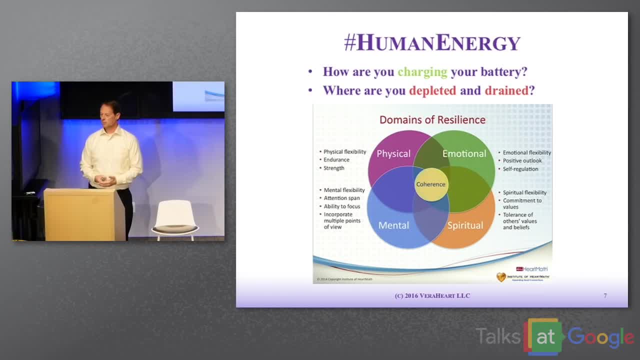 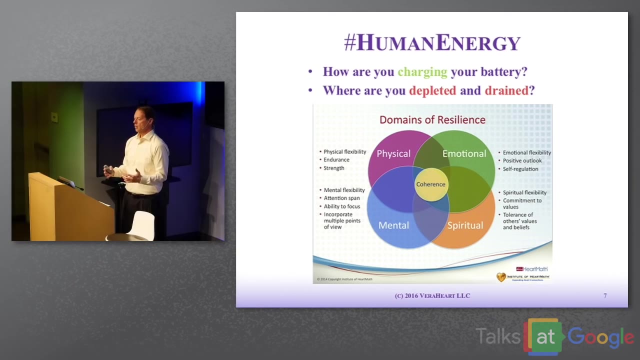 It can come from the physical domain. Maybe you just really exhausted your body. You did a major workout but didn't allow yourself the time to rebuild. Maybe you've got accumulated things that are going on in your physiology that don't allow you to efficiently in your systems. 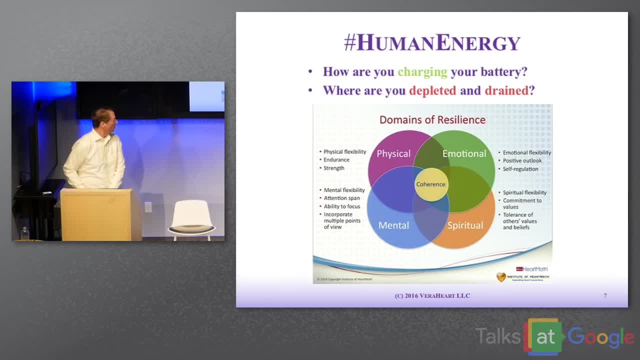 be able to generate more energy? That's a great question. Thank you. The emotional domain over there turns out to be the most important in terms of being able to build energy or stop the discharge or release of energy. Mentally, this is something we all in high tech. 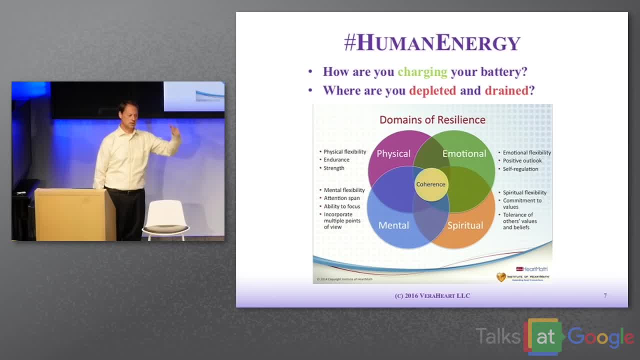 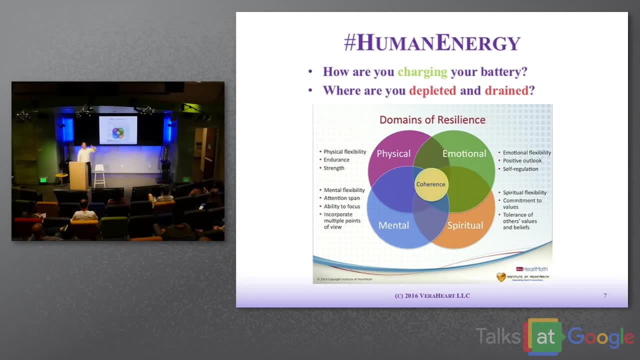 have got a real challenge. We are continually processing. I tell people all the time I have an A, B, C and a D processor and the C and D never stop. for sure, I try to hold the A processor in the front, which is problem solving. 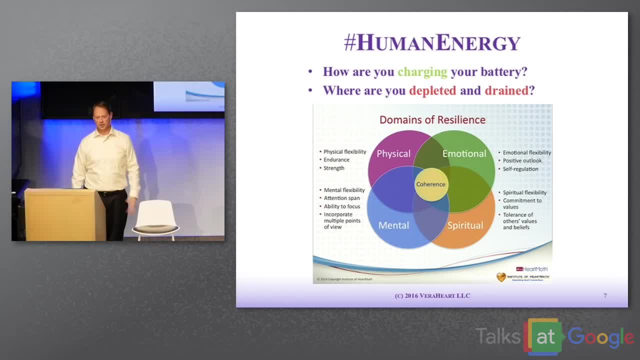 All the time. But the reality is, all four are working in that hyper-mental state. I could be exhausting my energy in that place. And then, even in terms of spiritually, are we operating within some place, that is, in our values? I go to a lot of places where we're going to work on the culture of the company. 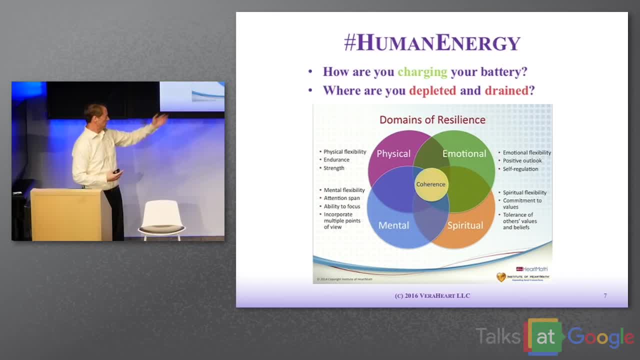 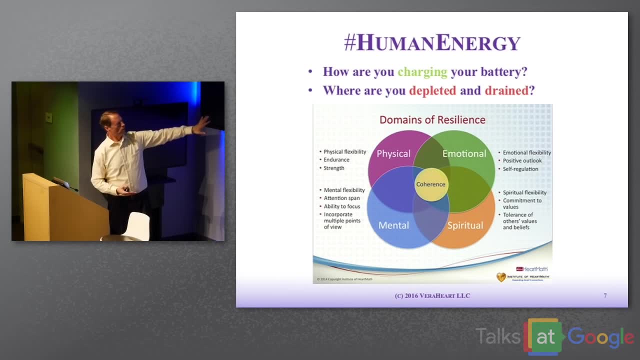 and the people's values and the values of the company don't match, And in this domain over here, people feel exhausted just walking in the door, And so you know it's hard. It's hard. You can look at all four of these domains for how you're charging. 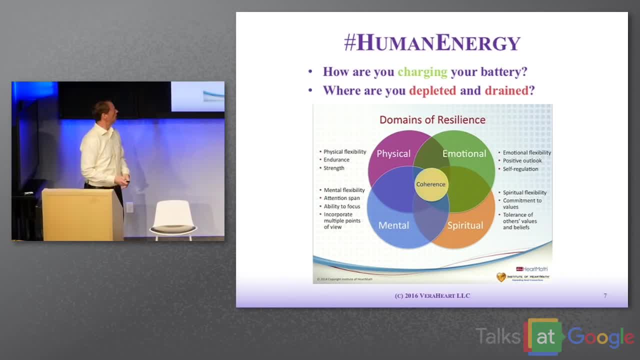 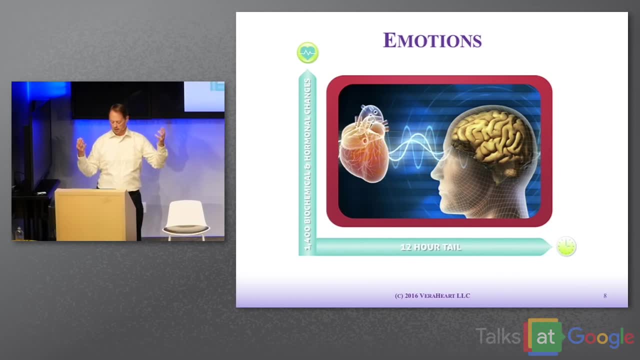 and how you are depleting your energy, which brings us over to emotions. Now here's something: Heart-mind connection. Let's explore that just a little bit. Emotions are key to energy. I've said that before. There's something that happens that when you experience an emotion, either depleting, 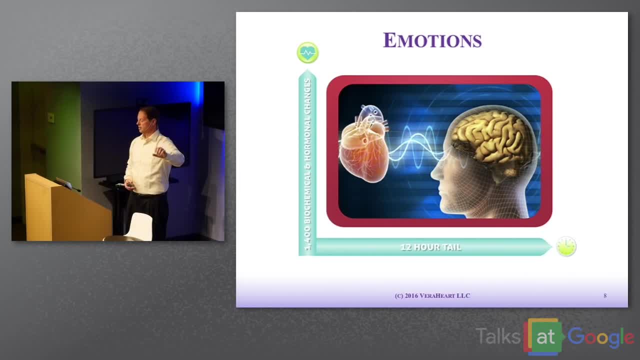 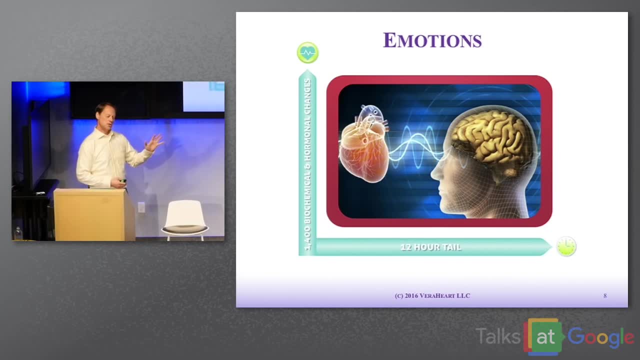 or renewing. depleting emotion might be anger, frustration, anxiety. When you experience one of those negative emotions or depleting emotions, it launches a 1,400 biochemical and hormonal set of changes in your body that have as much as a 12-hour. 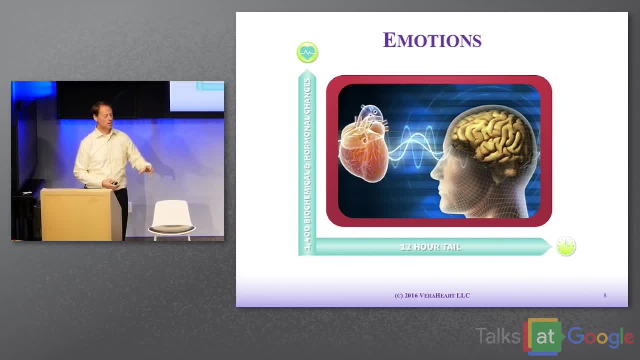 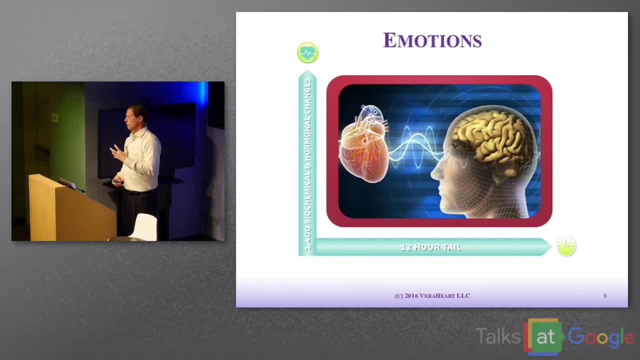 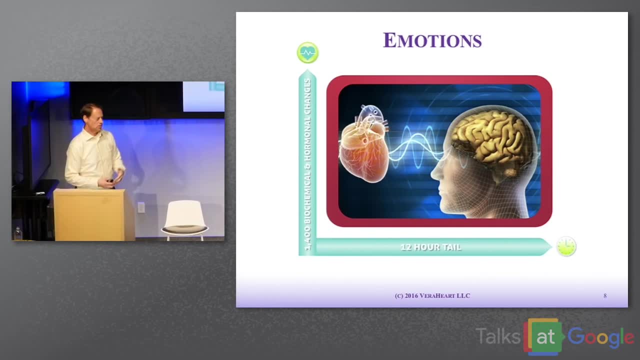 It has an effect on both your energy. It has an effect on your psyche and your physiology, both It sustains for a long period of time as well In the renewing side. so happiness aspects, joy, appreciation- they also, by the way, 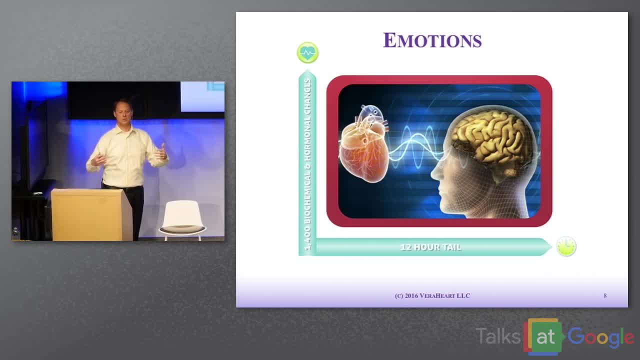 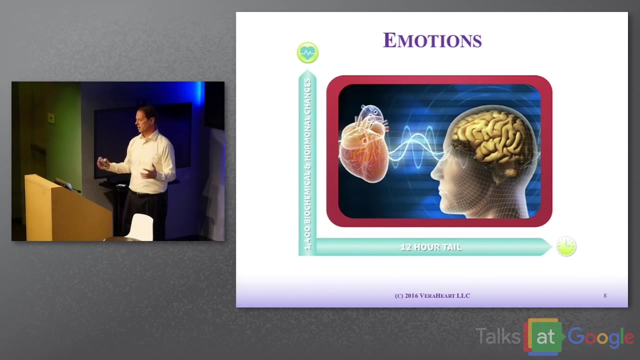 have an equivalent 1,400 biochemical and hormonal cascade effect in your body. that also can have a 12-hour tail. What's going on on the depleting side is the release of energy, in particular cortisol, and all the effects that cortisol, that that kind of drug, that. 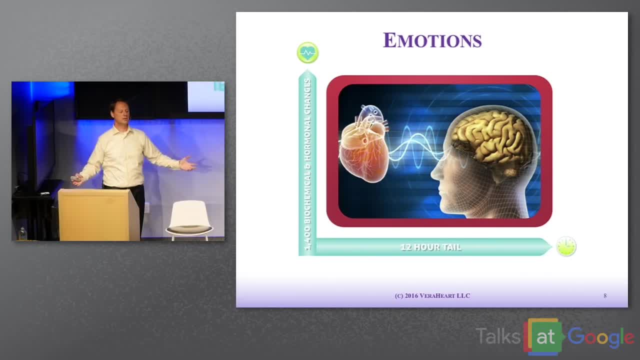 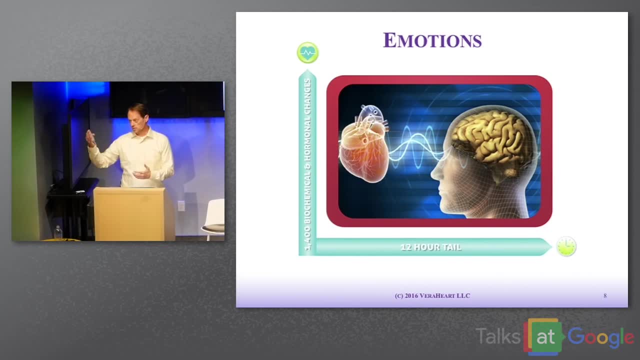 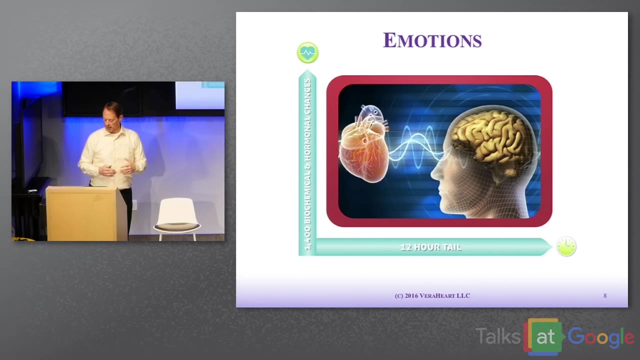 in our system that just takes us down and hard to get out of a cycle. or, on the renewing side is the release of dhea, and dhea is that that joyful joy kind of hormone. it's the one that we want to feel its bliss. the reality is that we're always drawing our bodies. they're trying to as human. 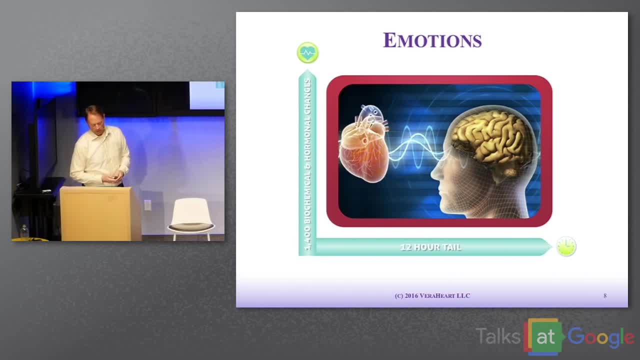 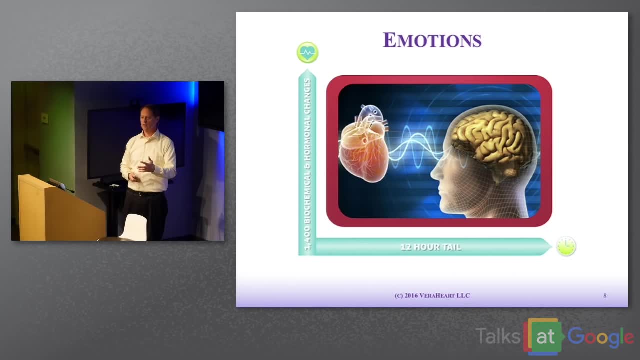 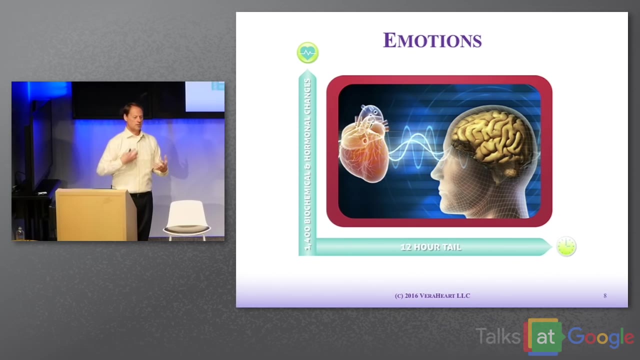 energy systems trying to balance those, and it's through our autotomic nervous system that that balancing effect is going on continuously all day long, through the sympathetic hitting the gas and the parasympathetic hitting the brake part of our system. we're wired to have this continual back and forth to be able to balance our system and balance our. 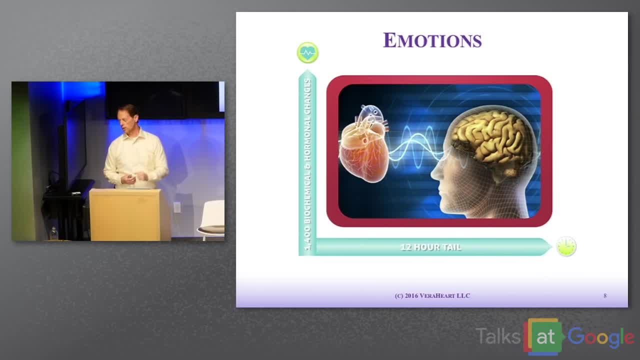 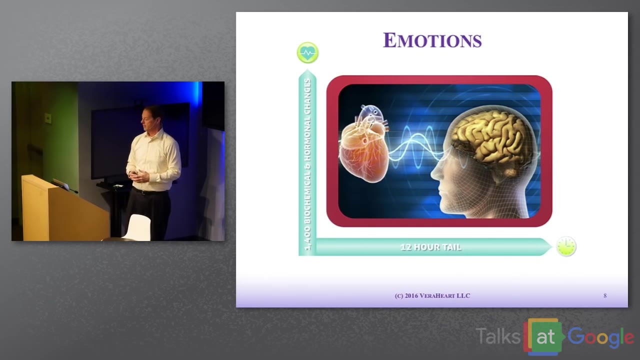 our body. our heart sits right in the middle with that whole process. our heart is where emotions are being encoded and affecting our energy in what we do all day long. that autotomic nervous system regulates about 90 percent of your energy and the functions that related to that, so it's breathing heartbeat. 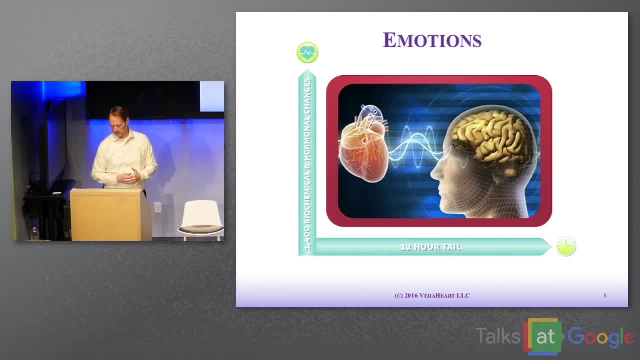 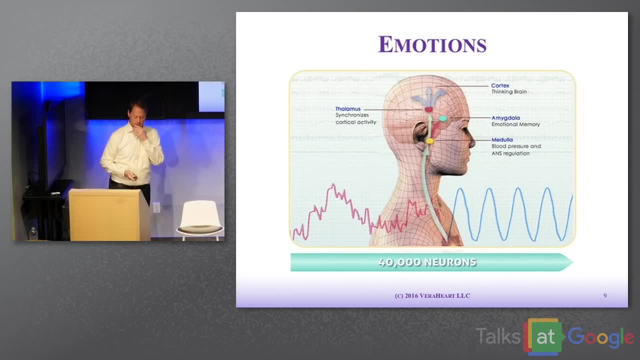 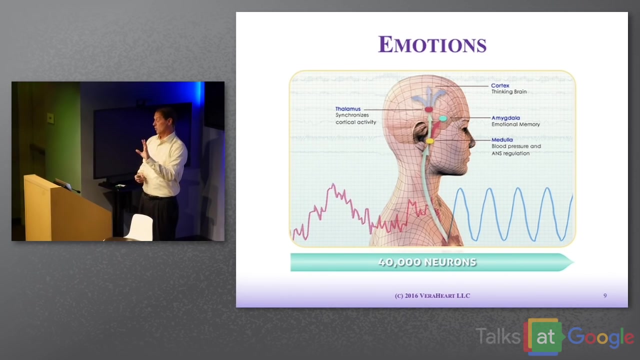 digestion, immune hormonal responses. they're all affected in this auto on our autotomic level nervous system. so the emotions part gets very interesting, because with our emotions you know you have 40 000 neurons in your heart. how many people knew that? okay, a few, it's it is. and just to be complete, by the way, you have 86 billion in your brain and you have 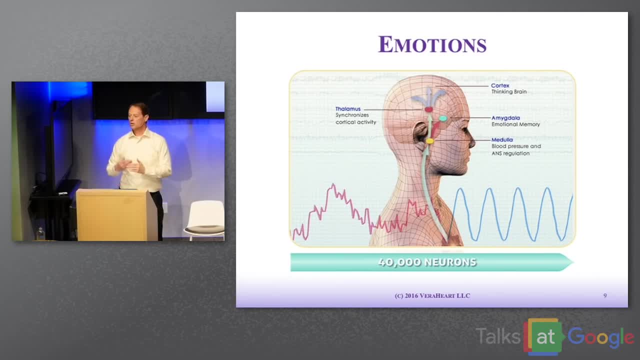 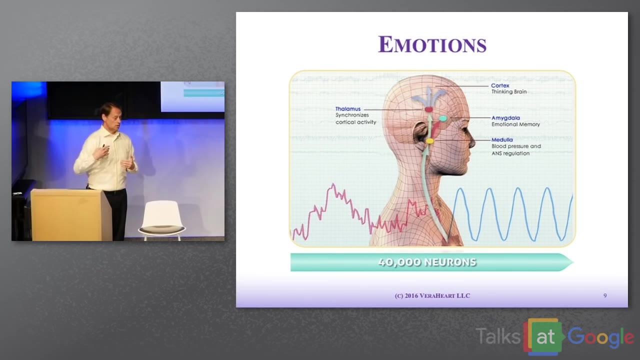 about a hundred million in your gut and those are all interconnected. now the forty thousand neurons, your heart, very interesting. these have been known about for a long time, but only it was about 20 years ago- began to be explored more and the organization that bear heart is aligned with. 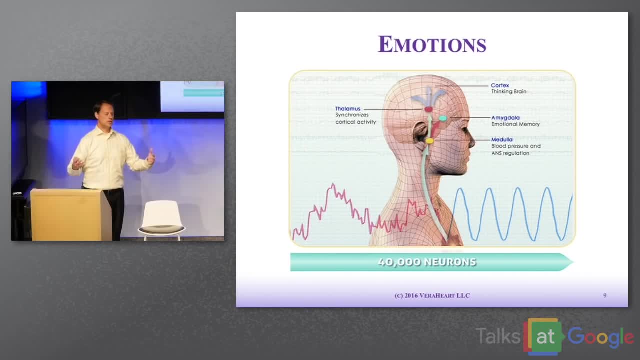 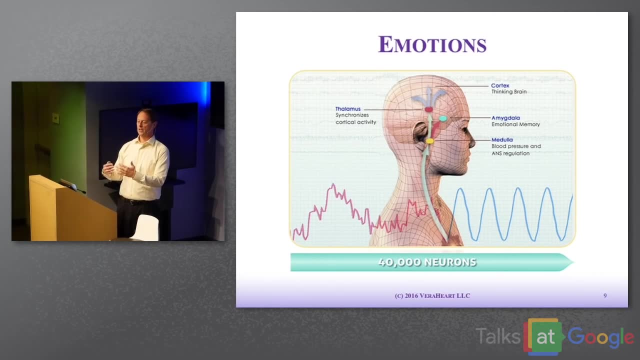 the institute of heart math is the leading researchers and practitioners. a lot of what we're covering here and the devices that come that we're going to use are from institute of heart map, where they've explored those. what's going on with the heart mind connection? what's 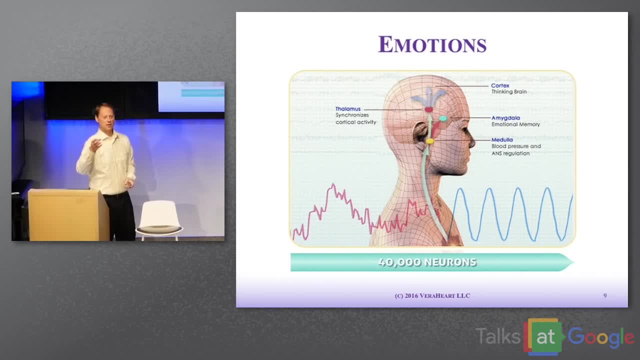 going on with these neurons. for instance- here's a little known fact but very important: there's a cluster of these neurons that in your heart that when you hold a feeling of appreciation, care or compassion, for just about 10 seconds you hold that, you feel it in your heart. that sends a message to. 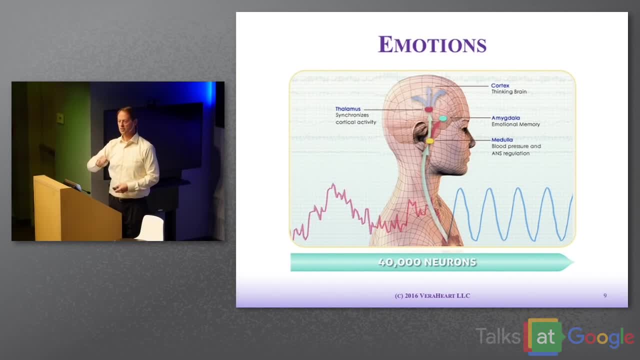 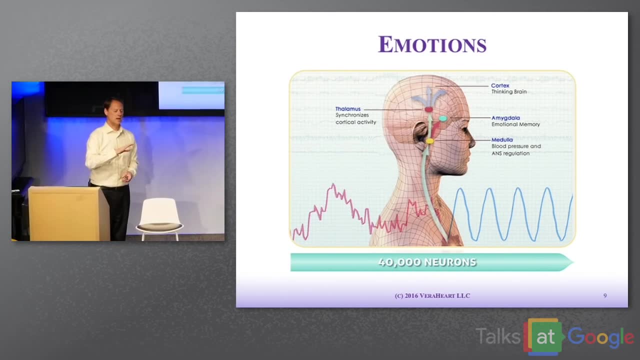 the, your frontal cortex, to your brain and it launches a very specific uh hormonal and biochemical set of drugs that can be used to treat heart disease. and to treat heart disease, changes in your body that carry joy and carry appreciation, carry it throughout your system. you're in control of that through being able to hold that kind of attention with appreciation. 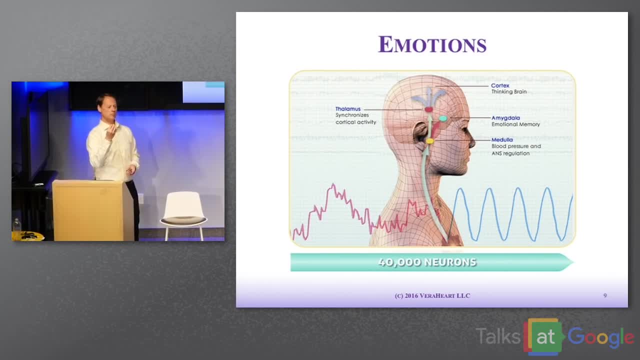 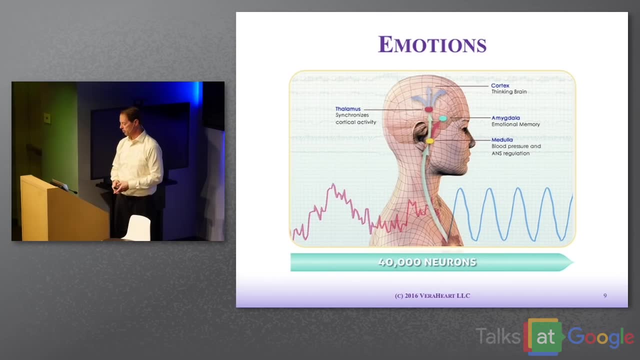 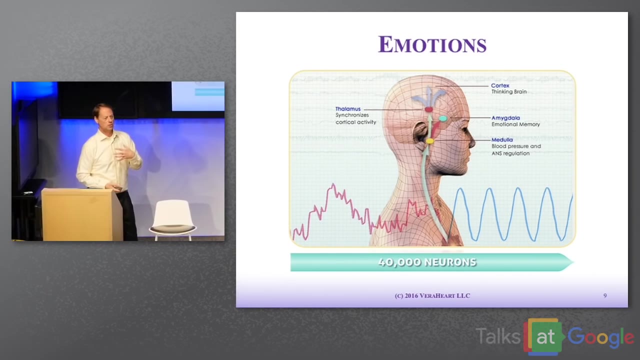 care, compassion- again researched, proven peer review, published research that is out there. that's talking about this heart, mind, connection with emotions. our, our emotions are really the world's best at doing these things and our brain meals part and parcel into our gut. very many of you will feel it here, because that's matter of fact, that the word heart is, i'm guessing. 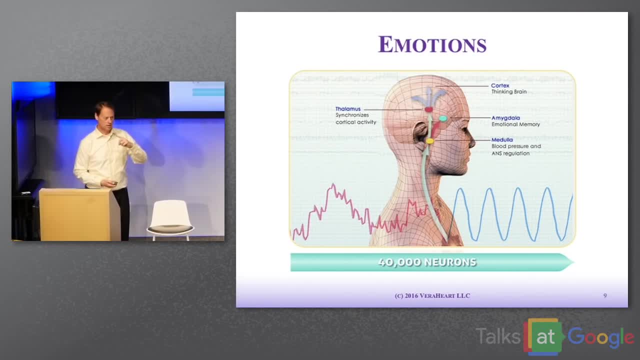 ethylene gas and in fact, in other words- this is unique- building these peleurs, we are actually communicating through our heart, through communication with the heart to the brain and through the channel of the brain, the medulla and the amygdala, and then up into the cortex. the reality is, when you measure the communications that are happening through the vagus nerve, through this connection, here the heart is communicating way. 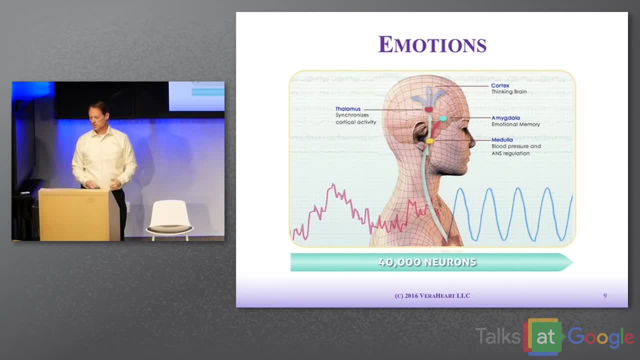 more with the brain than the brain with the heart. this say that again, the heart is continually communicating brother brain, brain with the heart. significant disparity. and disparity in that the heart is trying to send messages all the time. the heart is sending those same messages in the electromagnetic field and the the by being able to do spectral analysis of our 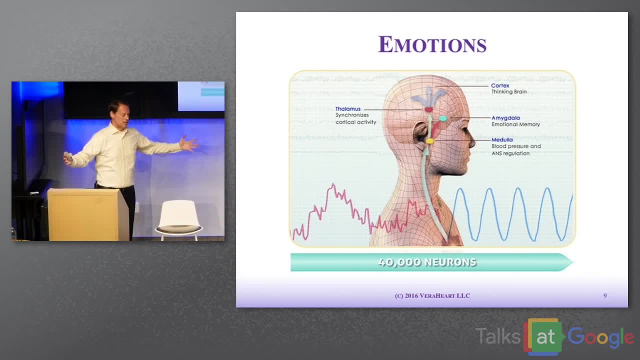 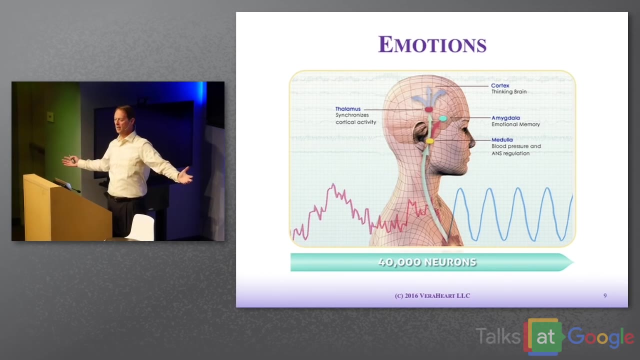 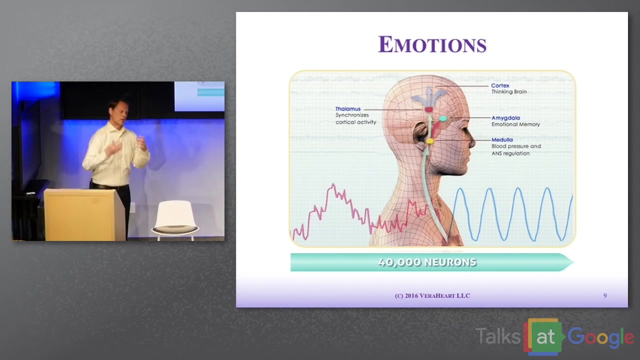 electromagnetic, your heart field, science. now researchers can predict with 75 accuracy what emotions you're experiencing. that's pretty phenomenal to be 75 accurate with using spectral analysis of your electromagnetic field on emotions. your emotions are centered around this heart mind connection and that's what's taken their heart, my company and us into focusing more on. so what? 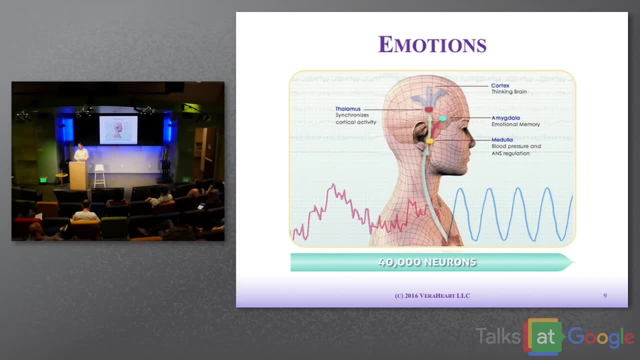 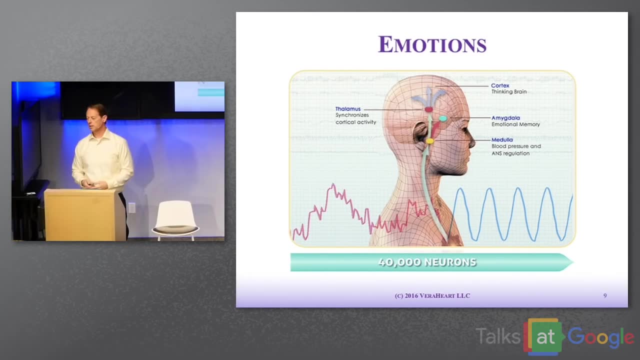 really is going on with the heart and these communications that are are continually happening, what the heart is signaling. there's other research that has really astounded me. what researchers love to do is to hook up people to to computers. of course, right brain activity, you know, heart monitoring, skin conductance on and in. 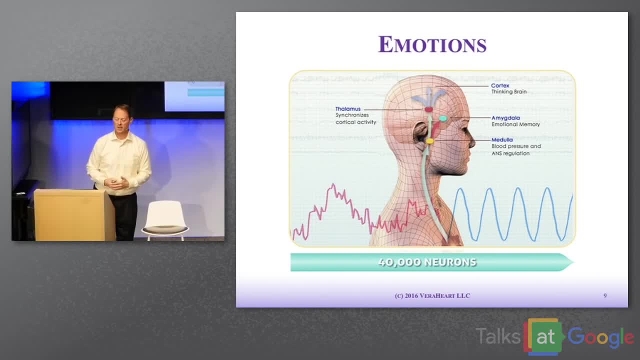 this particular study that was a very significant breakthrough, done with Institute of HeartMath. they would serve up either a horrific image or a beautiful, joyful image randomly selected by the computer and the participants that went through that study had they had control. they had the clicker to decide when the image will come up. 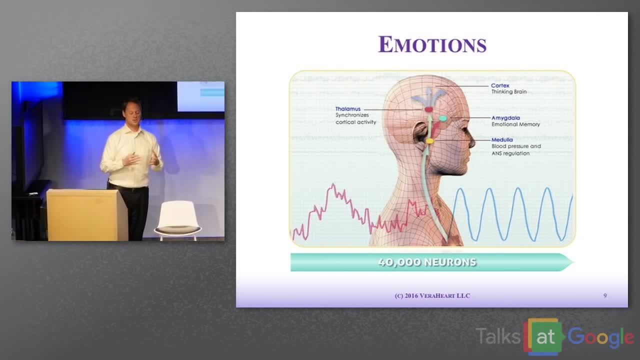 and there's more information that we want to get to. but it is has been good to see you're a part of this peer-reviewed study itself. and here's what the astounding thing for me: before, the computer randomly selected whatever image the heart new with the greater accuracy whether it was the 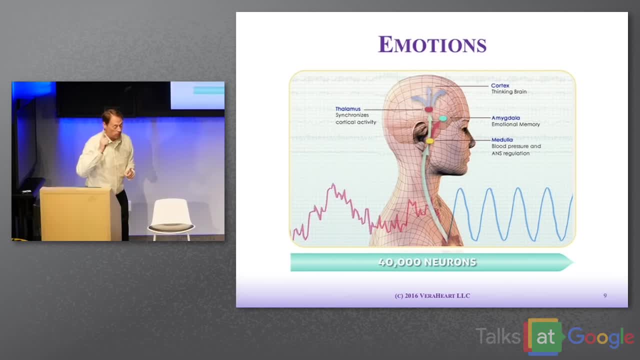 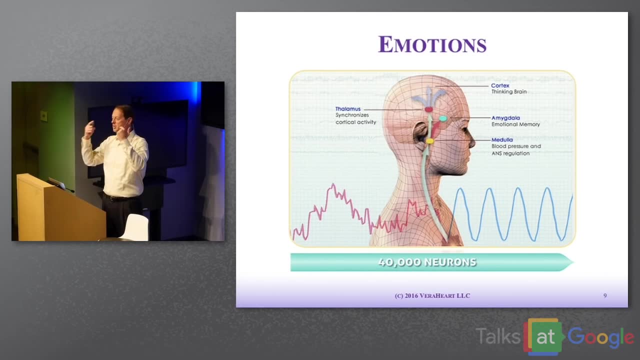 horrific or the beautiful, and sent a message to the brain. that's before the image was looked by the computer. and then, you know, the image comes sensory, we get the visual sense. the brain then gets the message and then sends a whole lot of messages out through the body. 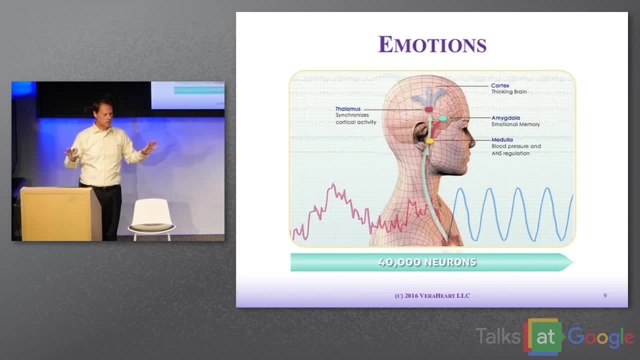 what is going on there? that is a that is a huge, huge piece of science that is just now being dug into deeper. our heart knows something more. our heart is sensing things. in this field, our heart is connected to our brain, trying to help our brain be prepared for what we are going. 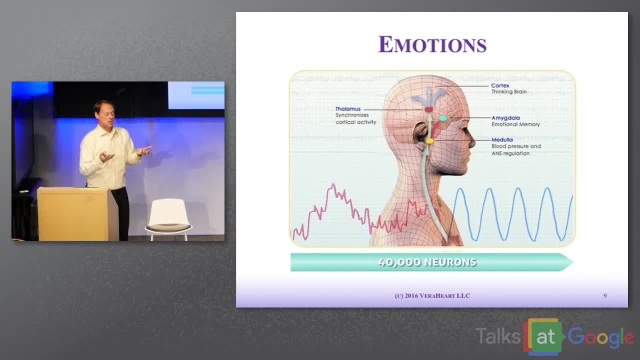 to experience, be prepared for lifting our energy. remember the heart is connected to our autotomic nervous system, obviously, and it is sending signals through the system, causing this release of chemical and hormonal changes in our body. your heart is way more active in what is going on with. 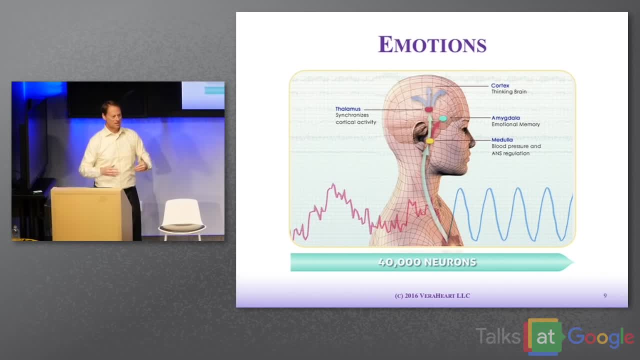 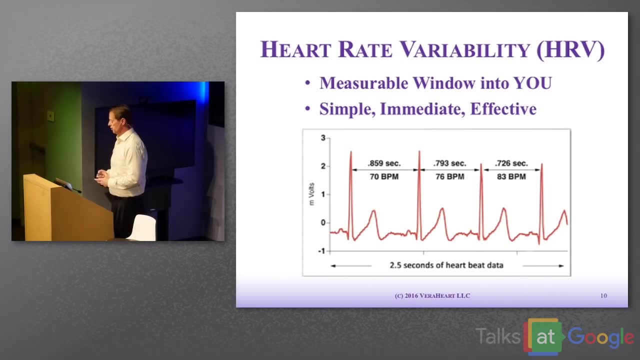 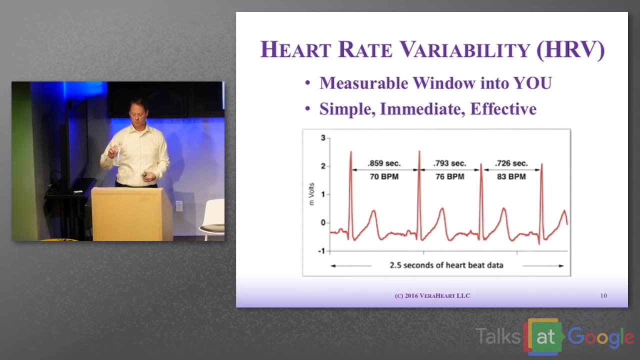 your energy than you're aware, and this, this now, is the good news- is that we have the ability to manage that intelligently manage, and that's where we get into heart rate variability. so heart rate variability gives us a measurable window, gives us the tool, and what it is simply is when we look at the amount of time between. 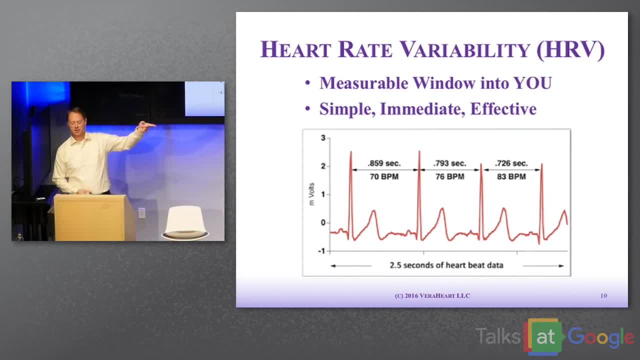 heartbeats and then we compare those, that's heart rate variability. it's a simple measure. now, i i love simple models and simple measures. maybe it's because i can't figure out the complex order of things, but it's a simple measure, and it's a simple measure, and it's a simple measure. 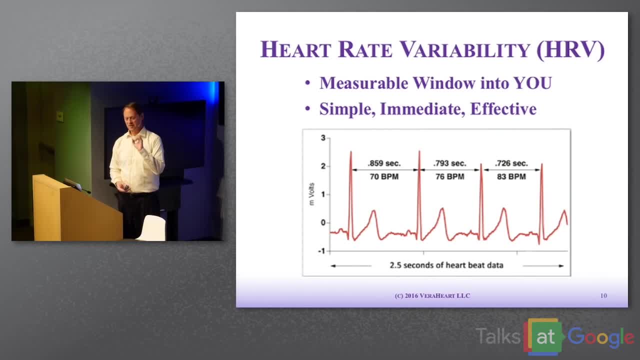 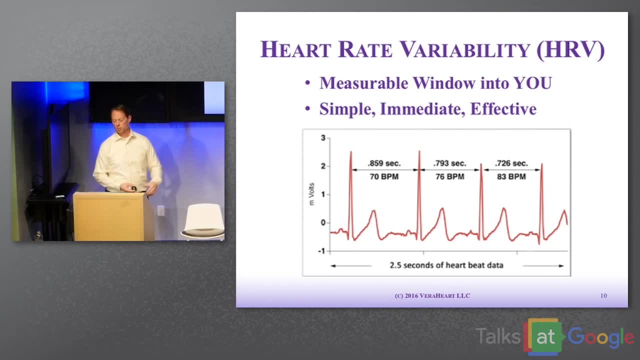 maybe i'm just too tired of complexity, but this is simple. it also is very quickly becoming much, much more reliable predictor of many, many different things in health care and and and the health care research fields. that's fundamentally what heart rate variability is all about. as the 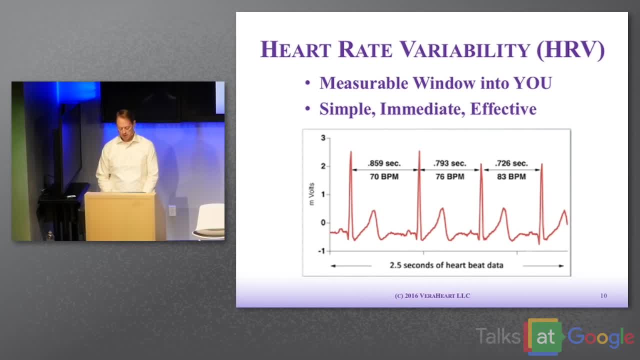 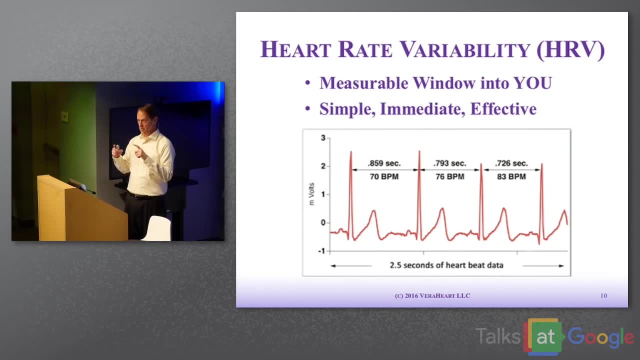 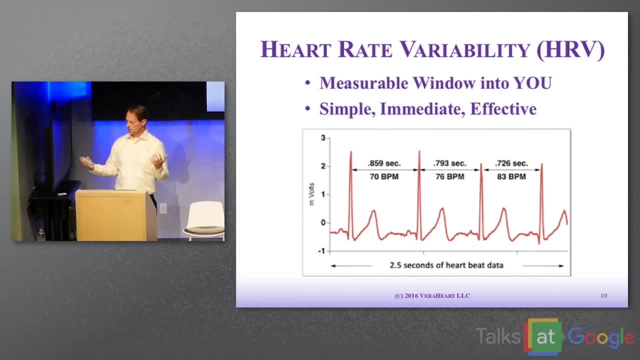 continual interchange and adjustment in our systems to try to find balance or to, if the heart sensing something to get ready to react to, then what happens? heart beats faster, right. variability, you know, shifts to be able to and reflecting this increase and a decrease in heart rate. variability is all about the heart rate. variability is all about the heart rate. 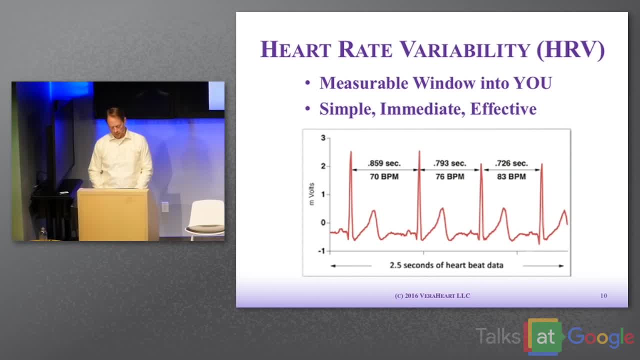 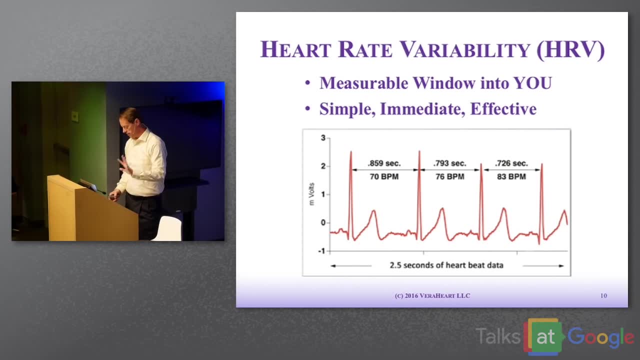 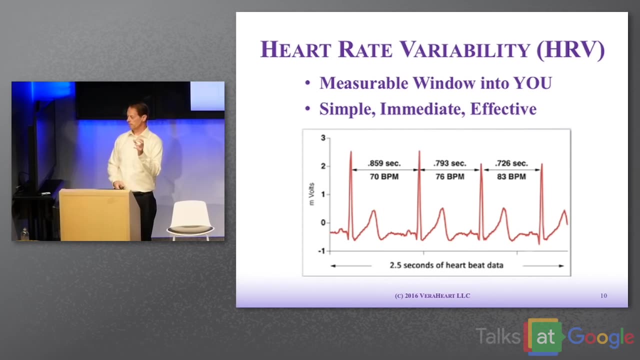 the amount of time in between, but the increased heart rate. and just the opposite occurs as well. so emotions are changing our physiology. we talked about that. well, depleting emotions create an an incoherent heart rhythm, a more, a greater degree of shifts in the variability of heart rhythm. 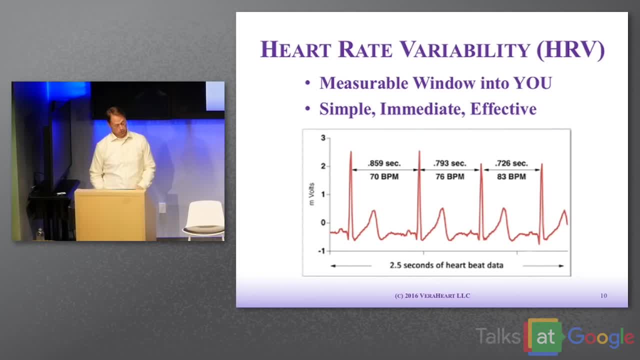 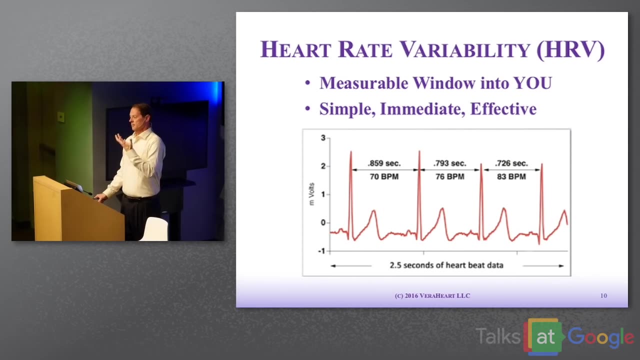 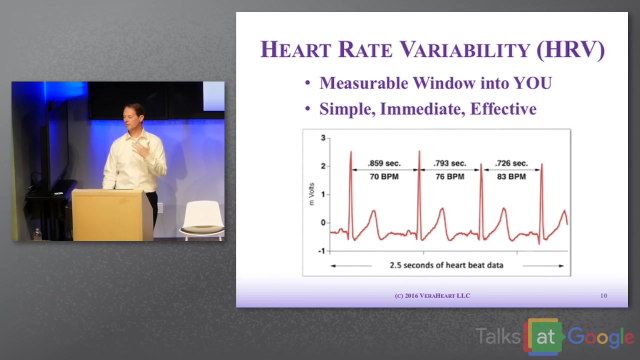 and renewing emotions, those that lift our energy, create a more harmonious or coherent pattern in the shifts of our heart rate variability. and the physiology too, by the way. as you breathe in, that increases your heartbeat, and as you exhale, you get a decrease. that's one effect of increase. 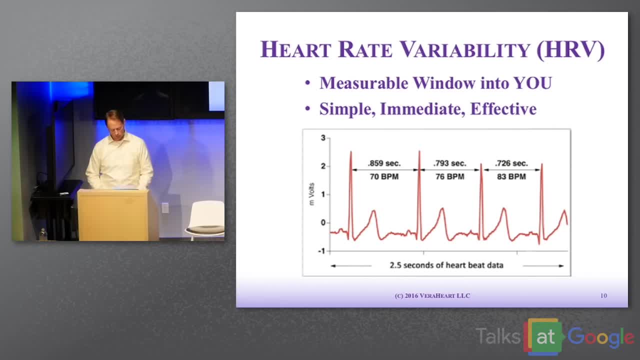 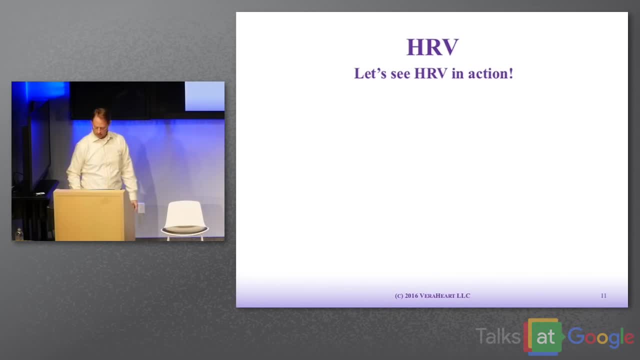 and decrease, but not the total effect. so what we what we have is a tool to be able to look at heart rate variability. now what i want to do is demonstrate, you know, heart rate variability in action. so i need a volunteer, someone who wants to come up and, you know, experience the biofeedback device that we have. 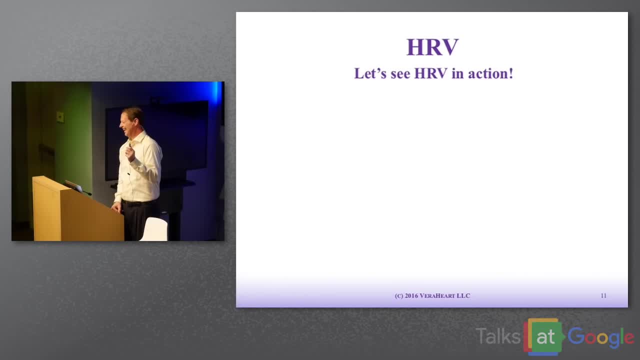 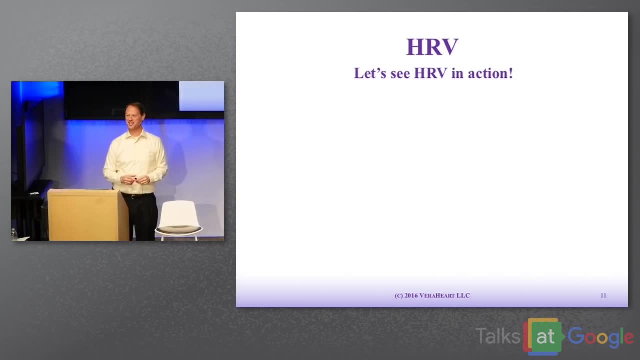 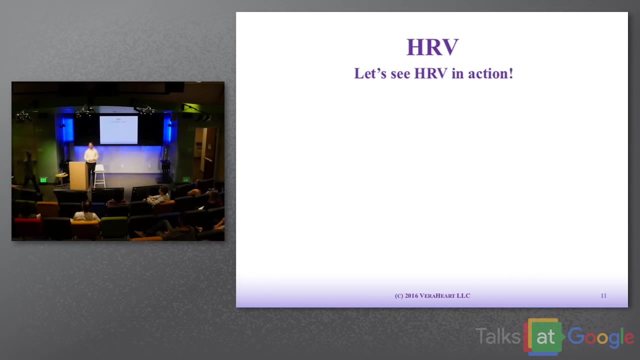 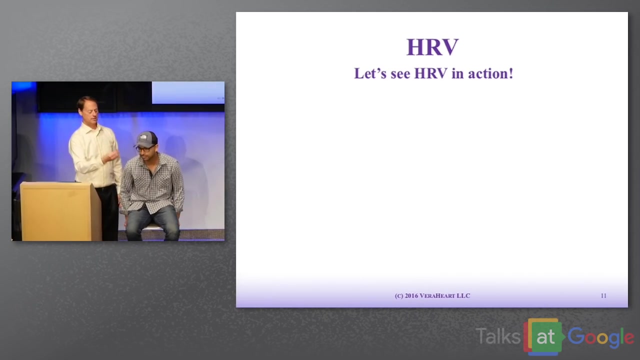 okay, come on up. you raised your hat. it's like a. it's like a, an auction. you know you had an auction paddle that you lifted up. thanks for coming. oh, did i miss someone? okay, we'll make time. yeah right, there's good. all right, we're just gonna hook that. 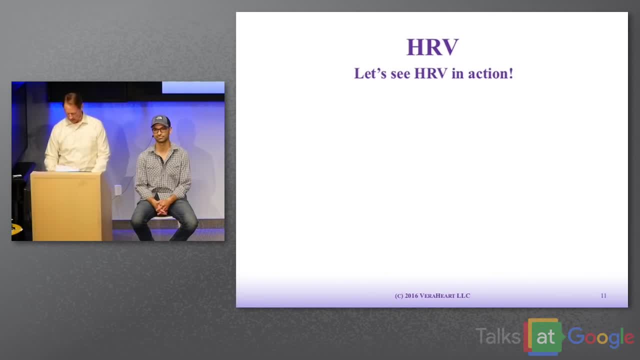 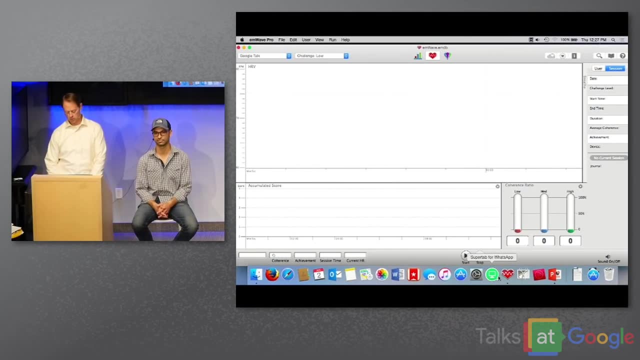 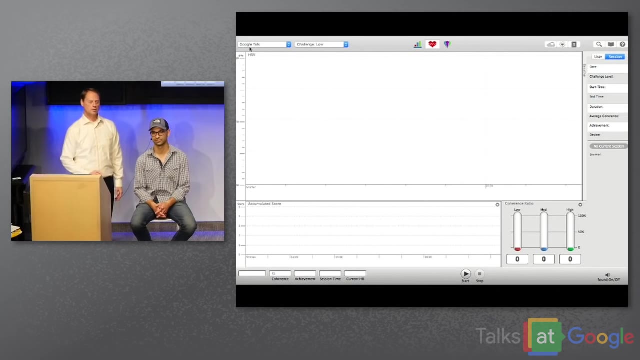 right up to your earlobe there. now what, uh? what we're actually using is a um, a dual biofeedback tool, and a piece of software from institute of heart math. uh, it's called mwave. this is the mwave pro version um, so that you can all. 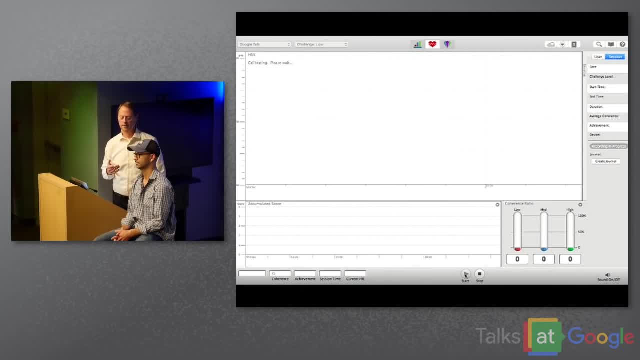 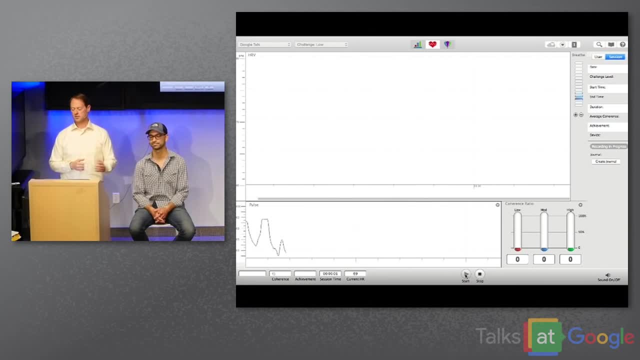 uh see it and and we can demonstrate what's going on with it. the sensor is an optical sensor. it's actually detecting pulse. what's your name, chris? chris, it's uh detecting chris's pulse. um, and you see, chris won't see because chris can't turn around, but it's. it's showing us that there's a. 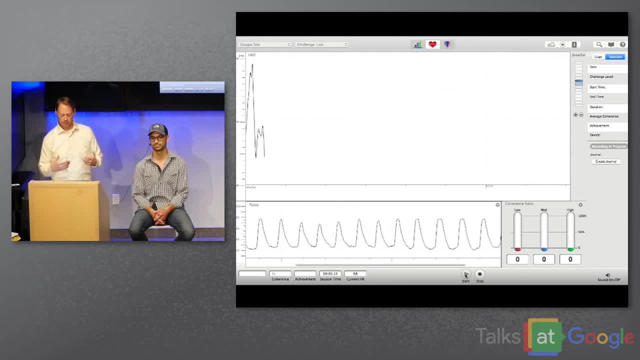 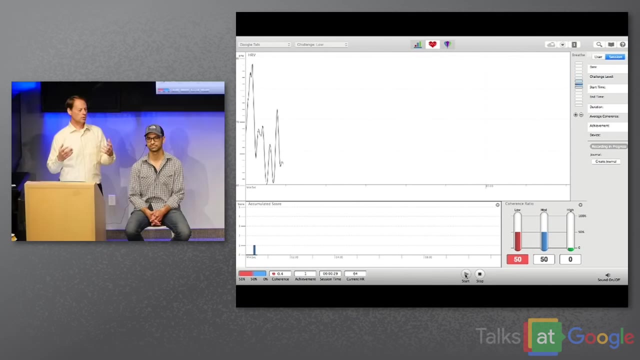 good read, so we've got good data. uh, this is a very good read, so we're going to go ahead and show you reliable data to be able to look at how this device can provide feedback or measure heart rate variability. so so, as this device is working, what it's doing is it's just literally trying to help. 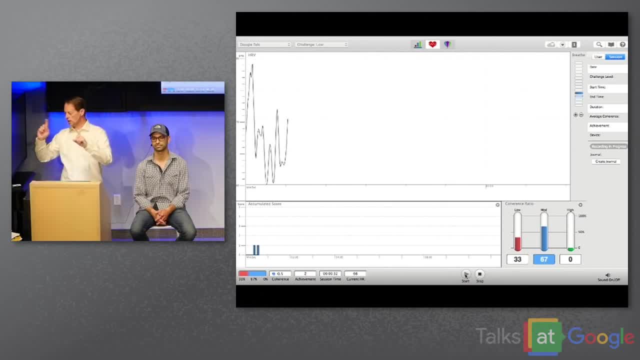 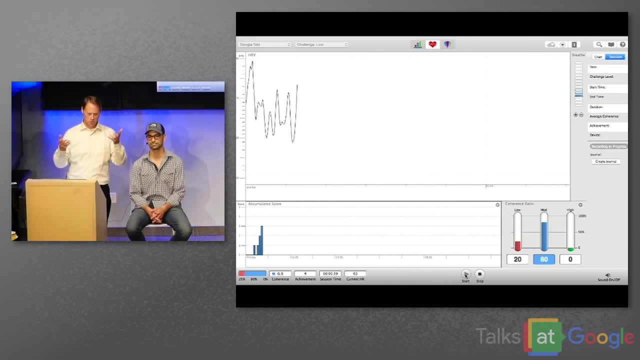 encode. it helps encode this variability. so those beat-to-beat changes that are happening and as chris is experiencing- you know, standing here with all of you staring at chris, who obviously loves this- um, you know, it's like his body is reacting, his heart is reacting. are you reacting? you think? 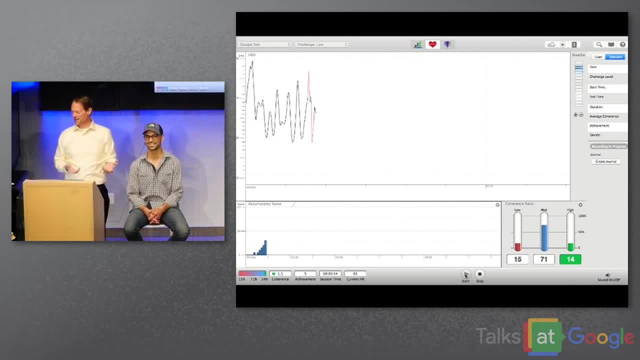 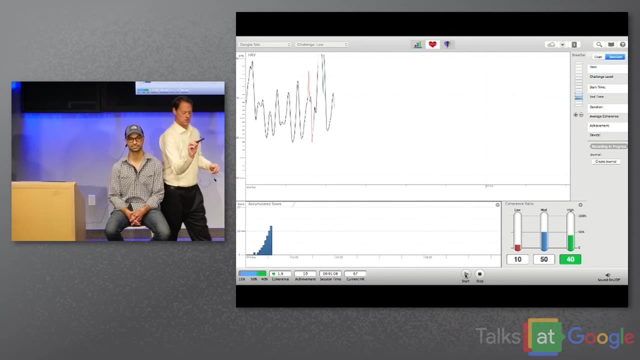 you don't look like you're reacting. you know, on the on the surface you look kind of calm there, chris. um, so so it let me tell you about these devices. um, first of all, there's, um, this is the mwave pro. there's actually a device which is, uh, mwave 2. this is a standalone device that. 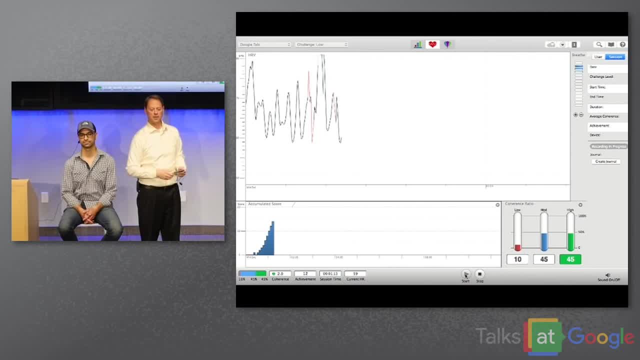 does the exact same kind of measures you. you get software very close to this that you load onto your system- mac or windows- and you can take this anywhere and what it does is help. it's an entrainment device, a biofeedback device that helps you to find. 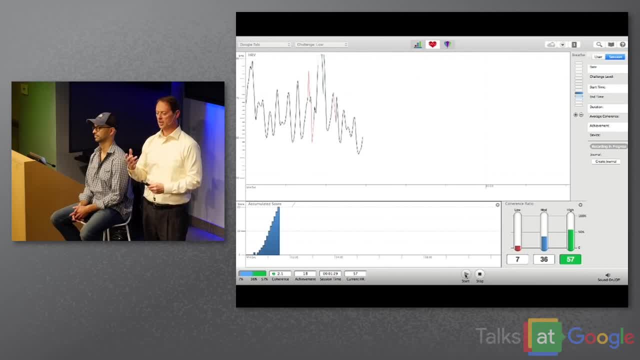 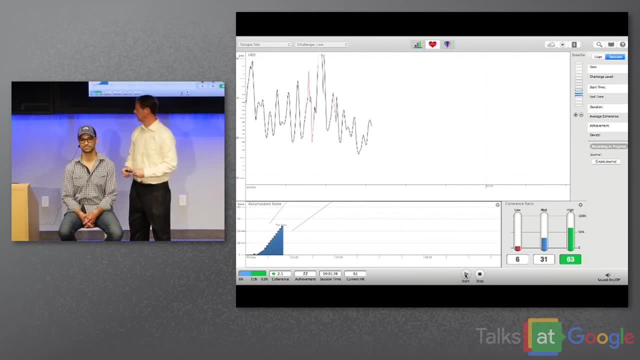 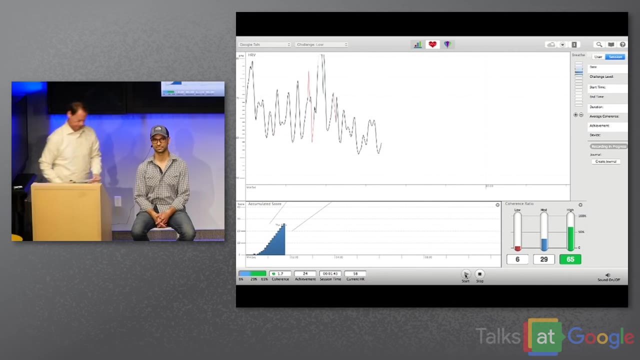 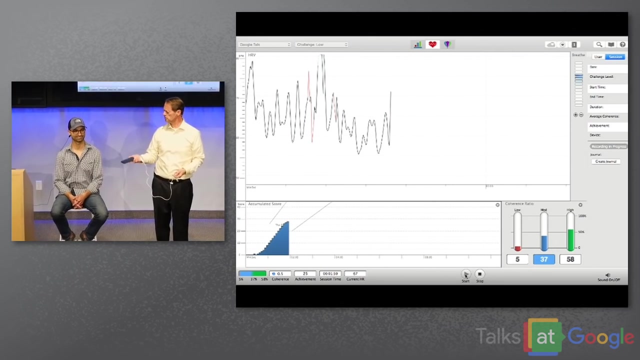 a natural way of being able to have the kind of heart rate variability that's going to build coherence and resilience. now i'm going to start using those terms as we go forward. so with these tools. oh sorry, i want to look. there's also another device. there's an app. the current app is ios. why do they always start with ios? 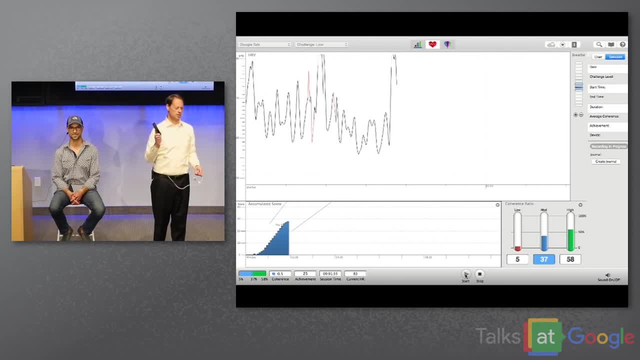 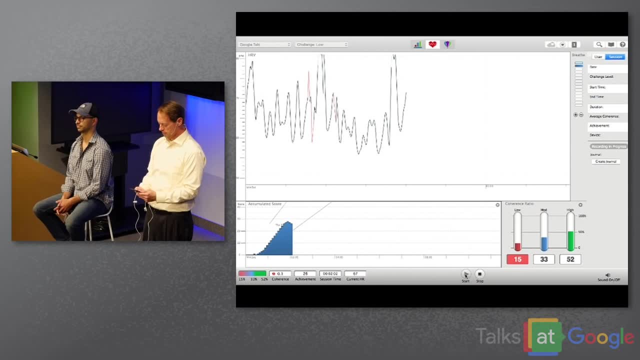 instead of droid. i mean, come on, let's create a shift here. the, the droid version comes out at the end of the year, i'm told. fundamentally, this, uh, this app- this is the ios version- has the ability to do the same thing as that standalone device. 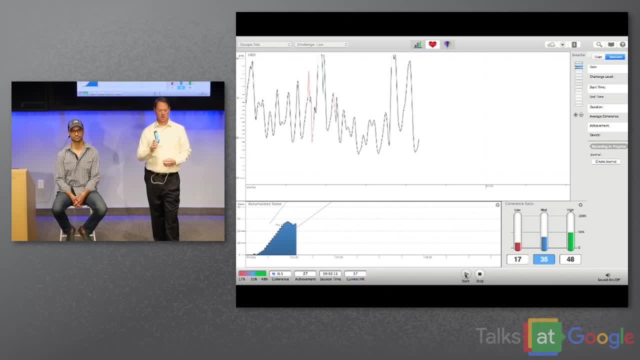 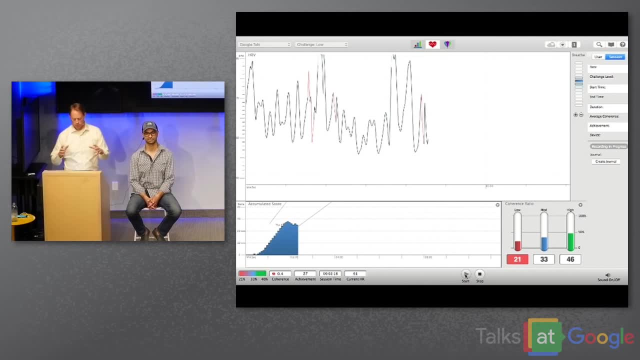 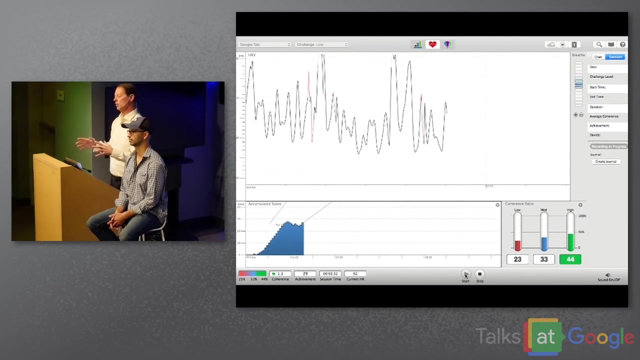 entrainment, biofeedback, being able to use heart rate variability. okay so, um, we're all going to get a chance to use the most fundamental part of of improving heart rate variability and and this is called heart focused breathing, and so we'll. i invite you all to to do this with chris and myself. okay, so, um, in your seat, find. 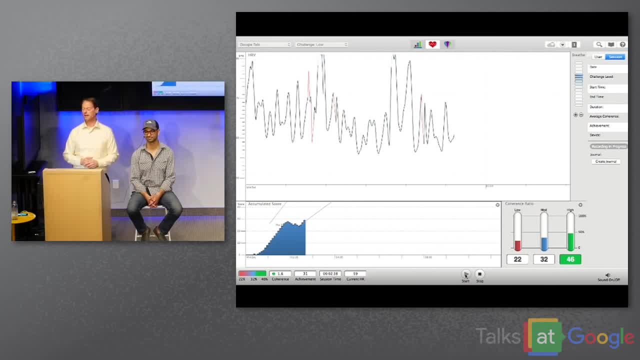 find just a comfortable position in your seat. you comfortable, chris. okay, you've looked comfortable all along, but not really. i. i have data proven otherwise. okay, so, in that comfortable place, pay attention to your heart now. if you want to, you put your heart, hand over your heart, begin breathing through your heart or your chest area. 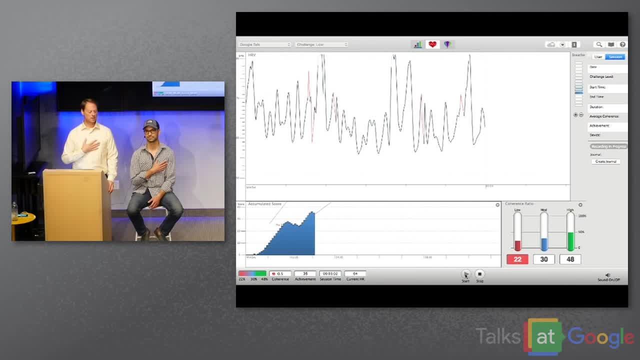 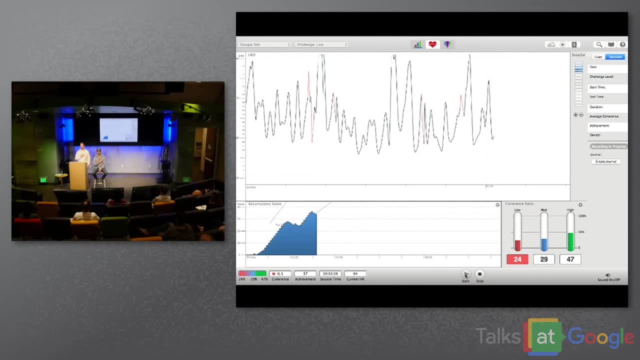 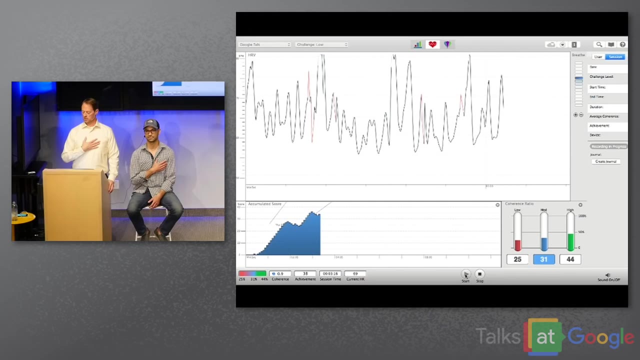 breathe a little deeper and slower than normal. five seconds in and five seconds out. again five seconds in and five seconds out. five seconds in and five seconds out. continue that breathing and as you're breathing a little slower and deeper than usual, just allow your mind to give you a 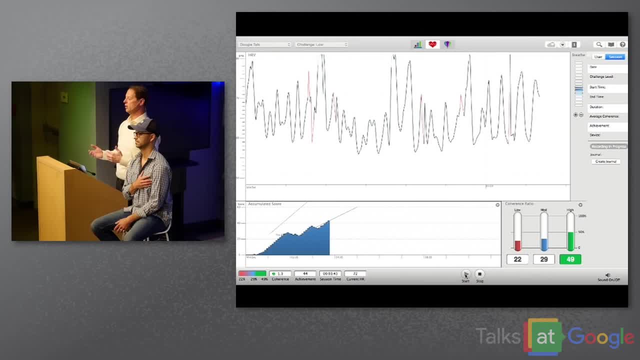 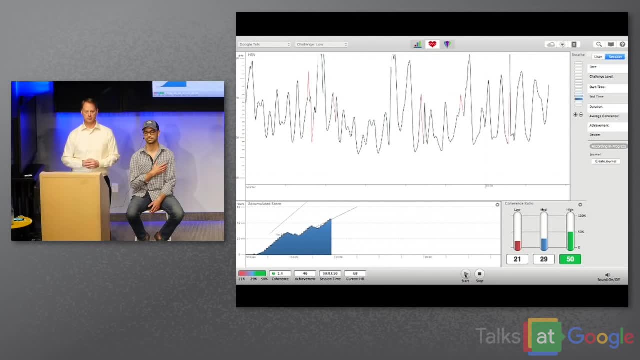 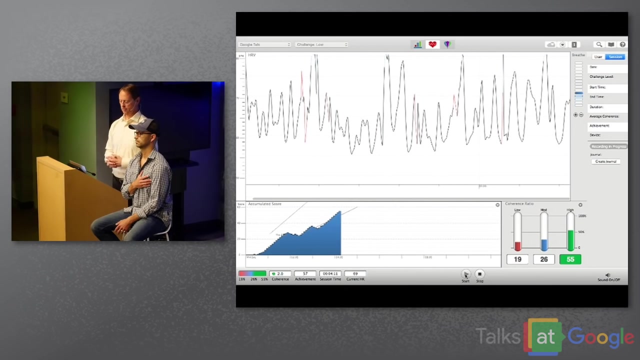 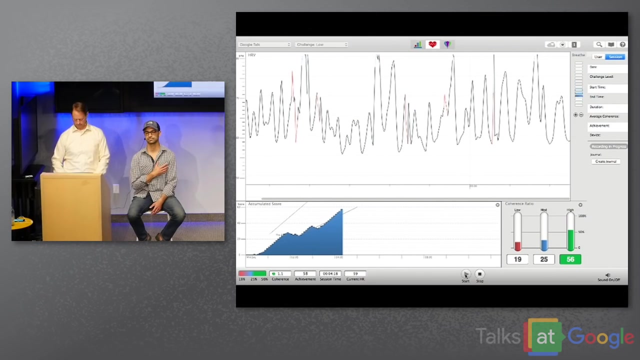 feeling of appreciation, care, compassion for someone or something, Whatever comes in, allowed to come in and just hold that in your heart as you're breathing. Continue the five seconds in, five seconds out. We'll do one more cycle: five seconds in And five seconds out. Okay, so I'll stop the data recording. Chris, Thank you. 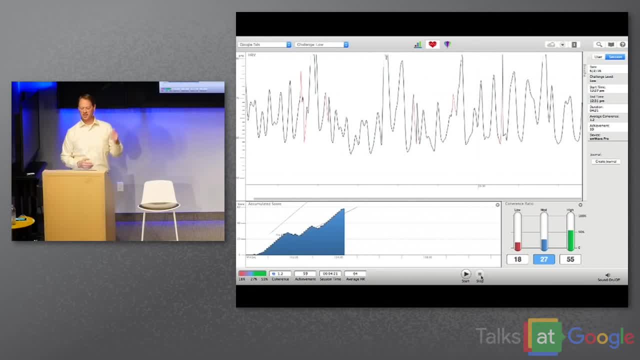 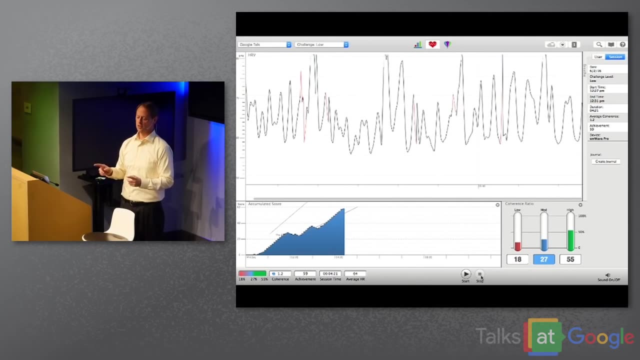 We're gonna let you go. This way. you get to see your data too, Okay, Well, first of all, Chris, you're gonna live. That's good news. All kidding aside, turns out, the heart rate variability is one of the emerging best predictors of all cause mortality. 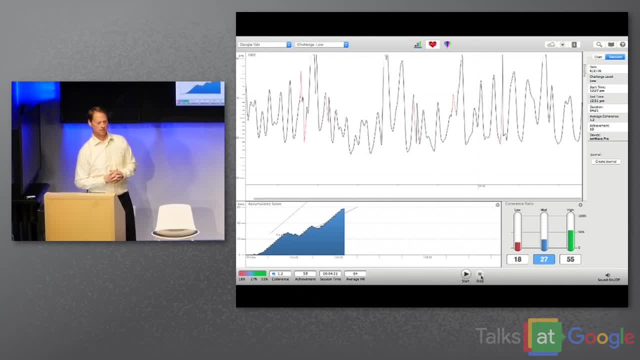 That is a very fancy way of saying. if you want to know if you're building longevity Or not, This is a good indicator of that. In fact, heart rate variability is now, Through the research being done, is able to predict someone's age within about four years. 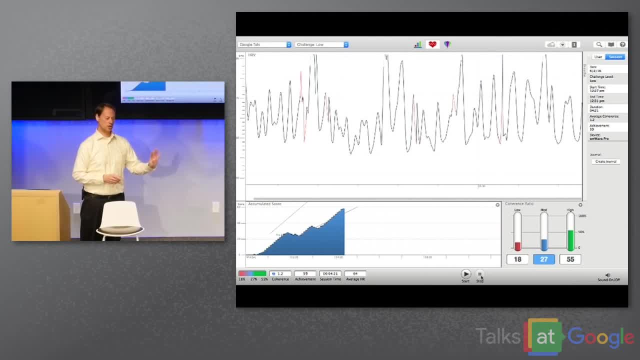 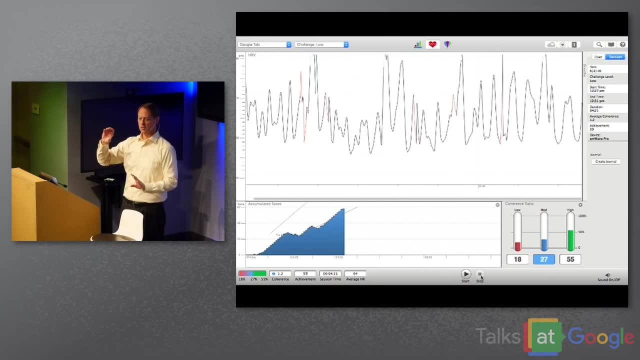 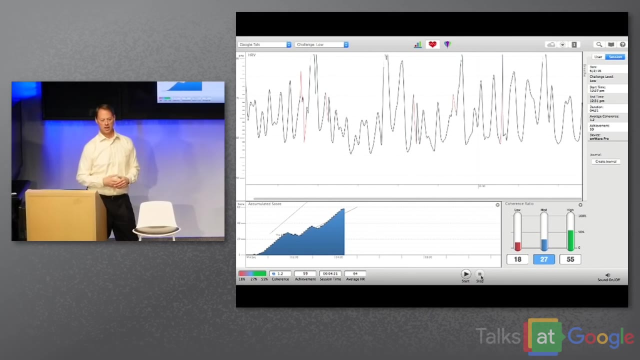 And that is because that what happens is we're younger, we have greater variability, greater amplitude in this way and Reduces over years, And so, given no other changes, science can predict your age within about four years. But the good news is, you can fool science By working with these kinds of tools. So here's what happened. We hooked up, Chris. 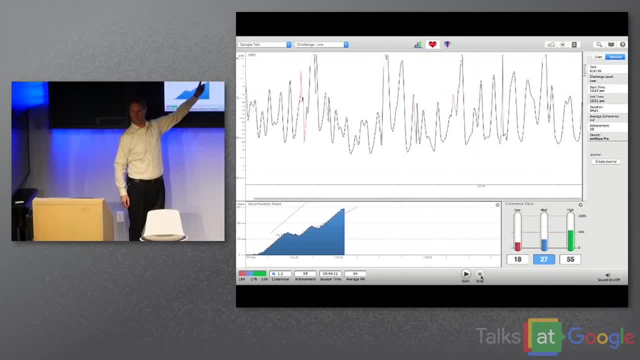 Chris is actually a Chris. Are you in the gpos group? Okay, so you might have been using some of that or you might just have all the benefits of gpos are gone. That's not too bad of a you know kind of a range. 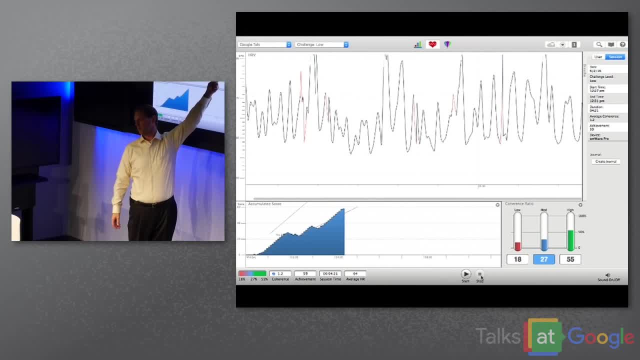 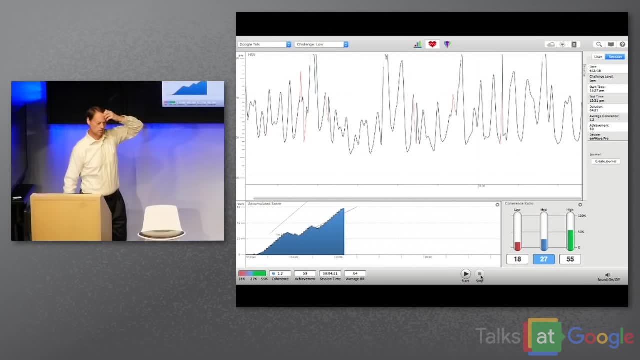 of rhythm. that's gone. you're right. here is where we started: hurt the heart, focused, breathing. and What do you notice about the change in there? I look at it and say, well, first of all, there's a more even kind of Wave. that's going on. There's greater amplitude and it's clustered, you know, together as well, and you have about a, about a 15. 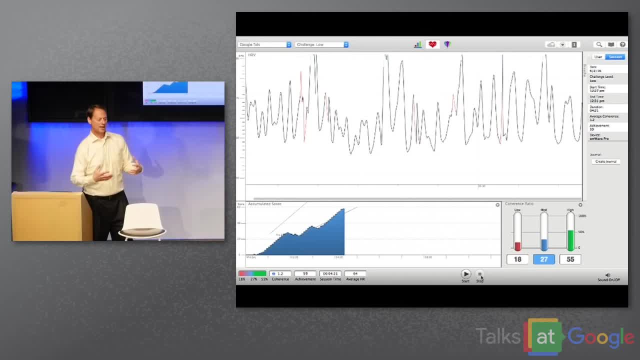 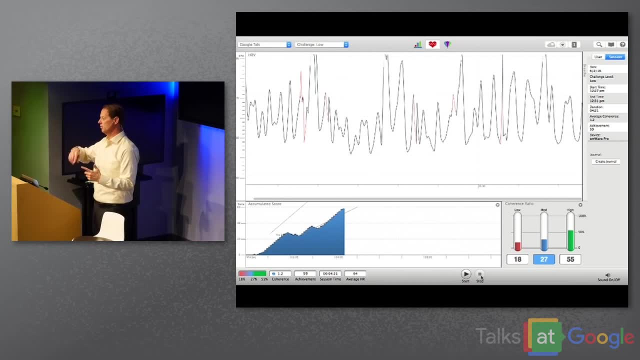 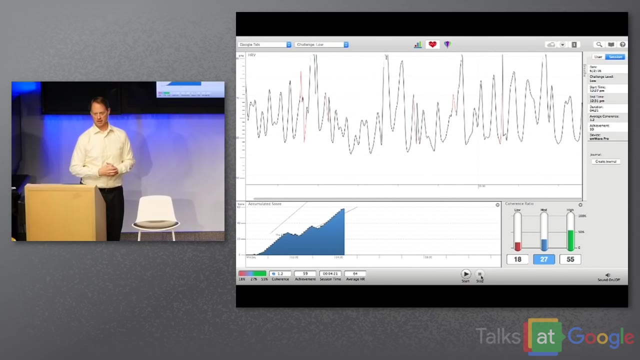 point spread over here. What? what you want to have is something that looks kind of like a sign wave that get that showing the level of coherence in heart rate variability and then the more amplitude. that's Indicating more resilience, that's indicating more Youth. that's one way people like it described. Okay, Good, Let's have we're doing in time wise. 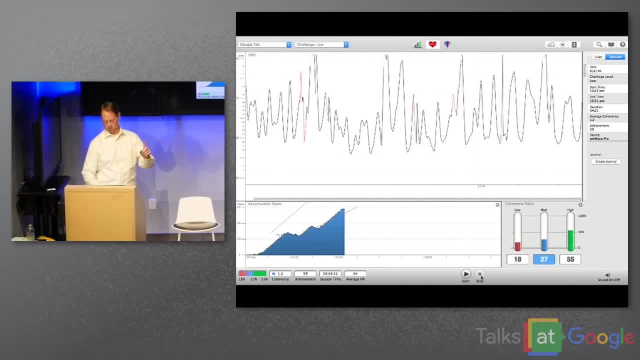 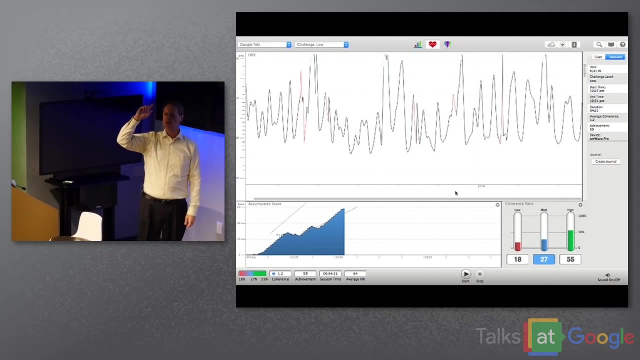 Think. I think we're doing okay to bring up for one more. Did you want to come up now that you've seen it? Come on, why not? We got time. That's. that is a drop of data, and then the pickup of data indicates that still a. 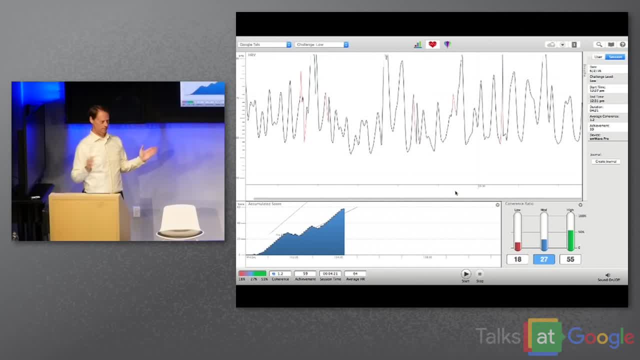 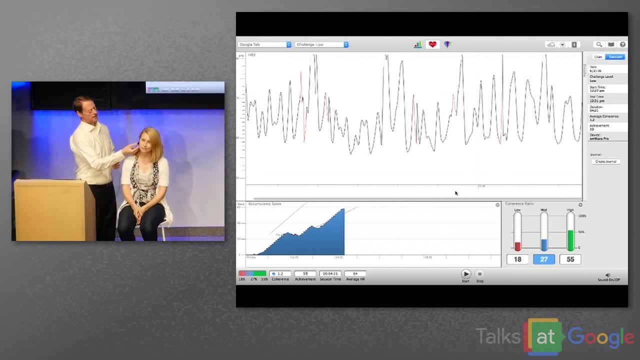 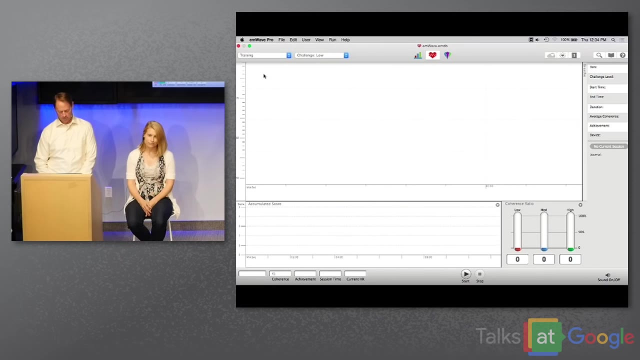 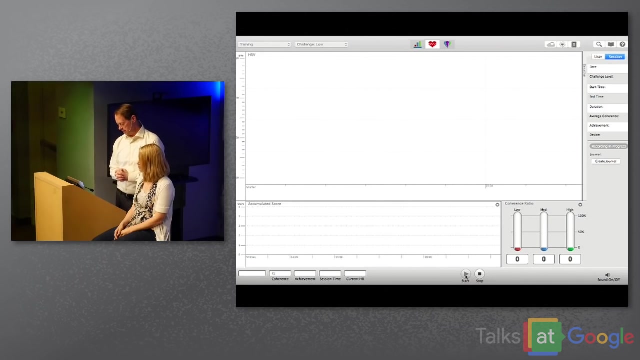 Coherent, another court, a valuable set of data. What's your name, Tiffany? welcome Tiffany. I should have asked okay to hook you up there. This is, it is now Okay. So what we're going to do is Just get Tiffany started out now. Tiffany has a little advantage in that. 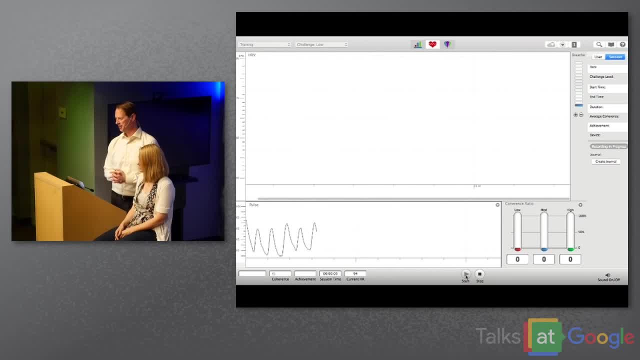 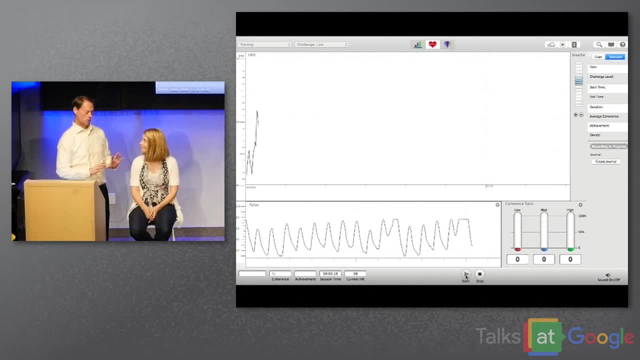 Chris kind of Was the real guinea pig and didn't have the benefit of all the other pieces that we went through. So you have a little bit more responsibility to generate a sine wave. No pressure, Tiffany, you know, Have you? have you been up in front of groups before? 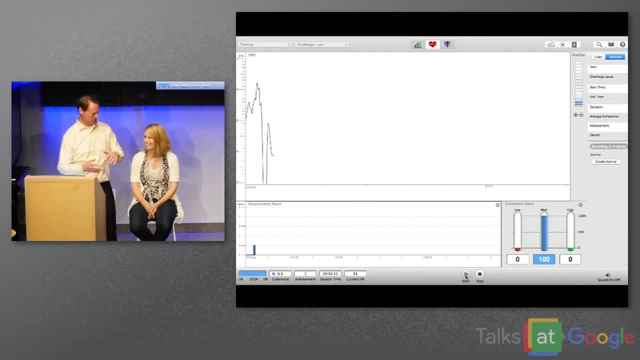 Yes, See, you know this is like interesting, huh. So you're kind of in an even place, You don't feel stressed or anything. Okay, we have more and more the more I talk. Okay, So what we're going to do is, as a group, we're going to do the heart focus breathing again. 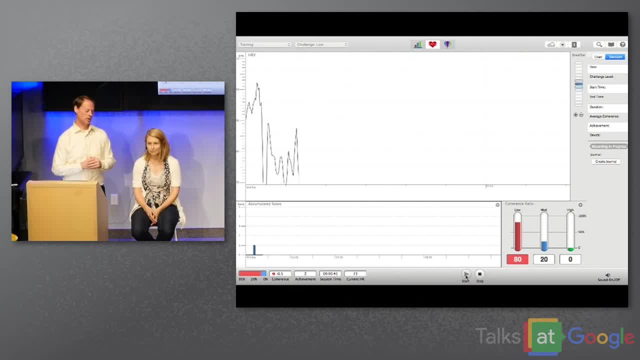 Okay, and we'll step into that. Go ahead and pay attention to the area of your heart And put your hand over your heart. if you want to feeling your chest rise and fall, Begin breathing through your heart or your chest area, just a little slower and deeper than usual. 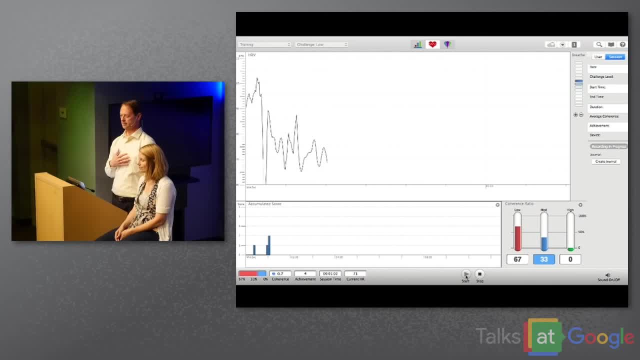 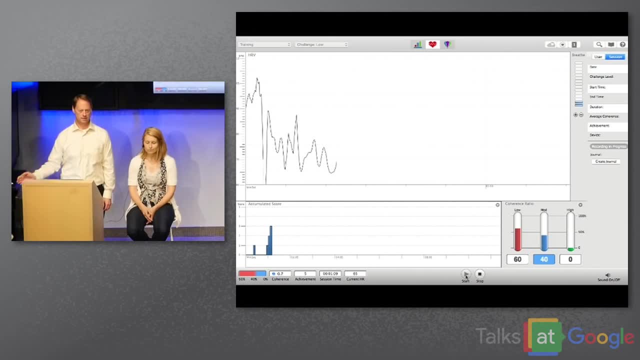 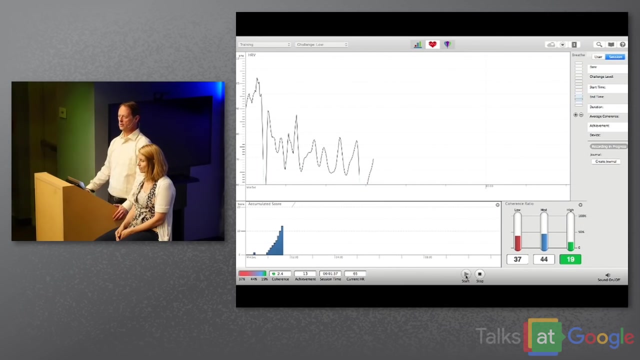 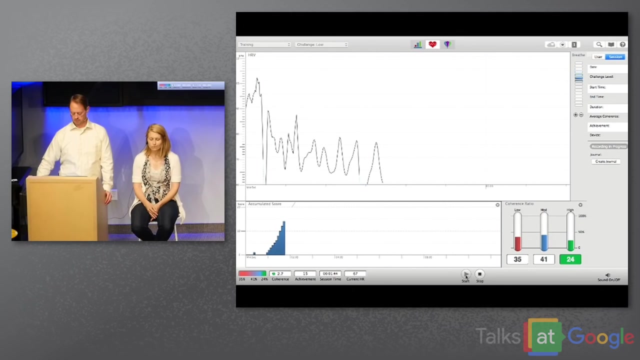 Five seconds in, five seconds out is a very good pattern: Five seconds out And five seconds in, Five seconds out. As you're continuing this five seconds in and out rhythm, Allow your mind to give you a feeling of appreciation, care, compassion for someone or something. Hold that in your heart. 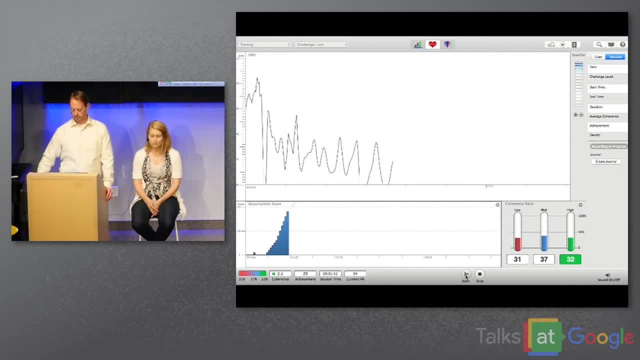 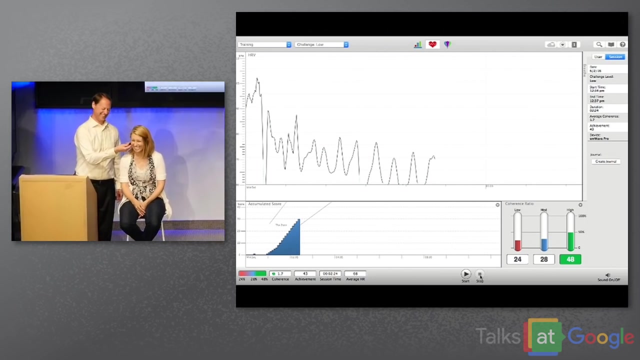 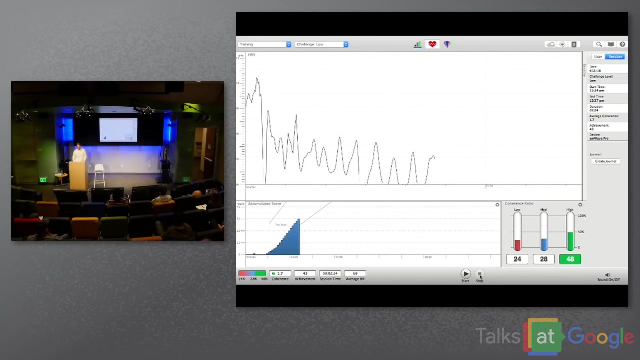 Continue breathing, Continue breathing. We'll do one more cycle, five seconds in, five seconds out. Great, now come, come back to Center And your chair is open. Let me show you off here first. wouldn't want to get a shock. no, Thank You, Tiffany. Okay, so we can look at Tiffany's data, could adjust the scale, but don't need to. we started out and she's pretty practiced. 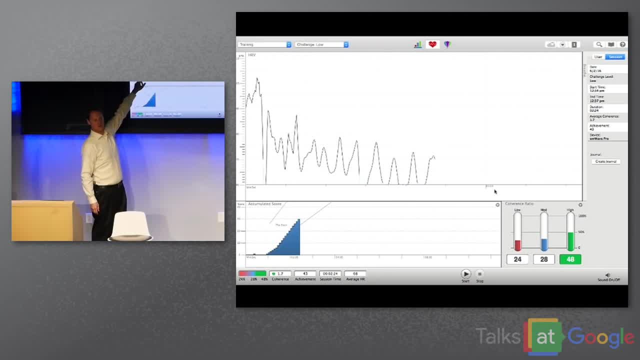 Sorry, and it was coming, but this was kind of just sitting in the chair for You know, just about a minute it. and then we started the heart focus breathing and you very quickly went right into a sinus rhythm at just a very nice sine wave and and flow. you have an amplitude. this we could pull up the. 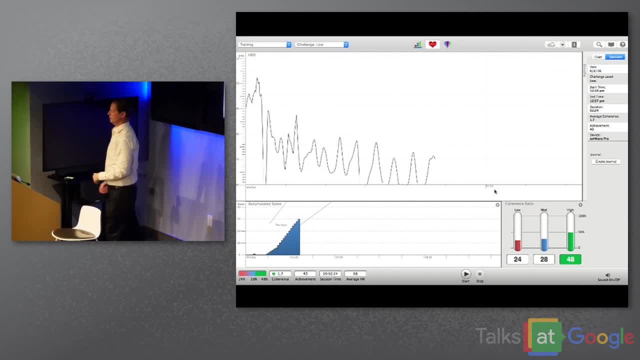 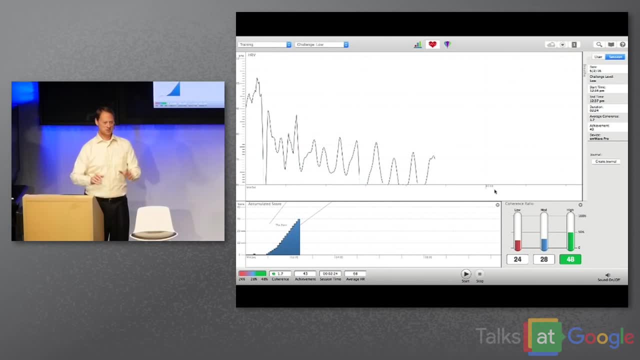 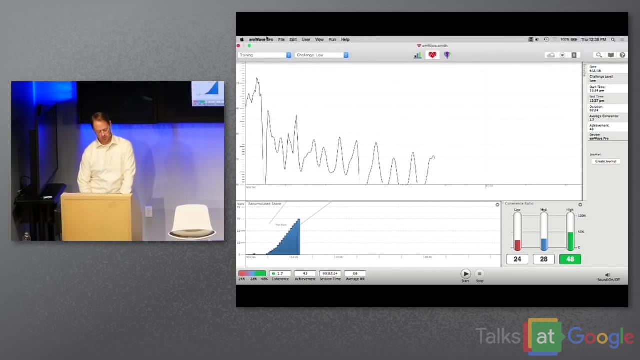 data, but won't be much below here- of somewhere around 10 to 15. you know points. so, chris, had you a little bit beat there- and resilience- not that there has to be a competition, but you have a new goal, okay. well, thank you for both, for being our guinea pigs and demonstrating the tool this, this. 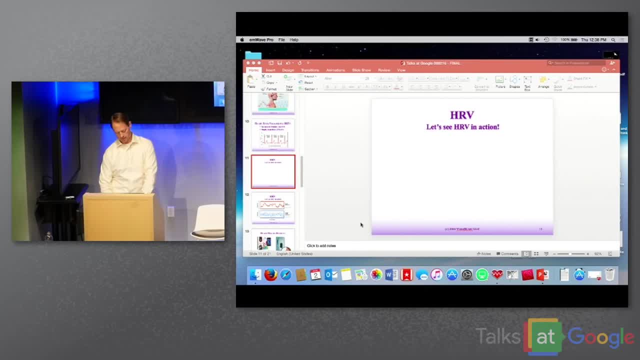 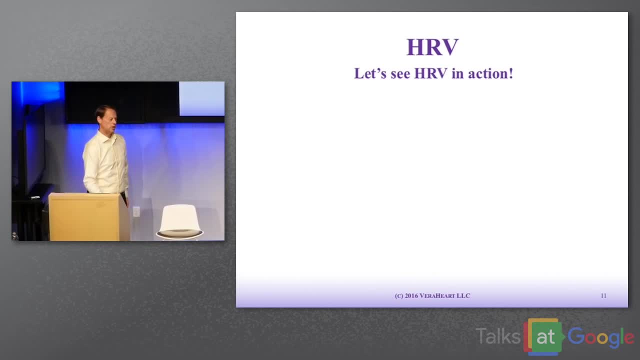 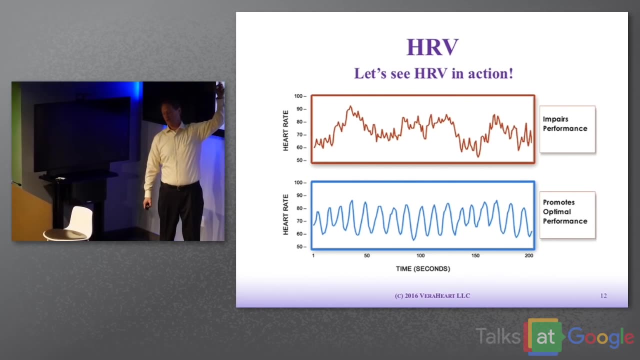 data that comes from the tools, the same data that use and the devices that I showed you, and it allows you to be able to train yourself and get the benefits of what's happening with heart rate variability. so, in in recap, this is actually the same, the same kind of process that we're. 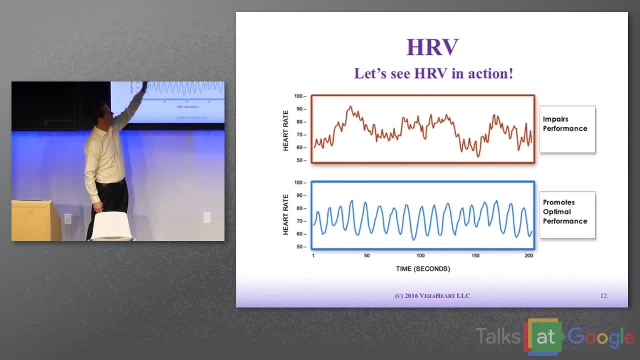 talking about so many sitting up in a, in a chair, and at the point the data ends here, come right here they begin: heart focus, breathing and that, that additional part that I added in, which is called a heart lock-in in Institute of heart math terms. what's happening in this top scale? what was? 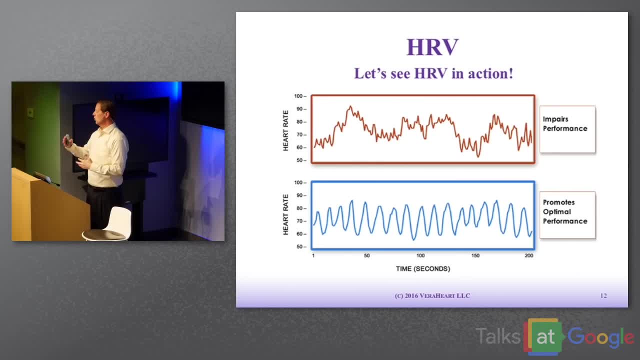 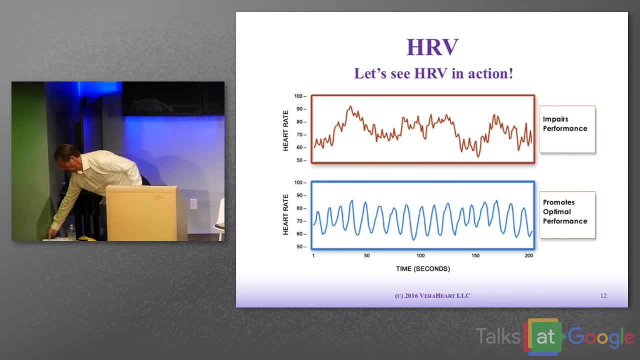 for Chris and a little bit for Tiffany- is a more erratic, more incoherent type of pattern in the biofeedback tool and that's indicating that jerky pattern is indicating that their autotomic nervous system is doing a lot of adjustments between the release of cortisol or DHEA. messages that with emotions experience. 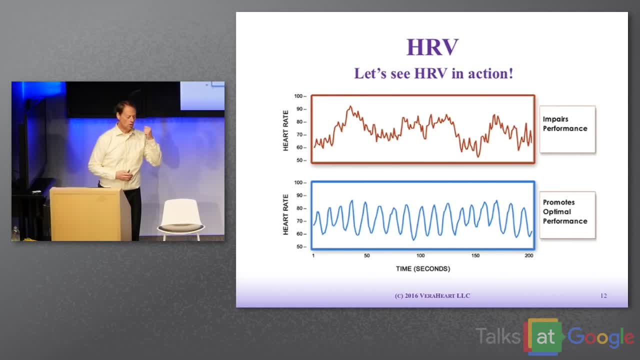 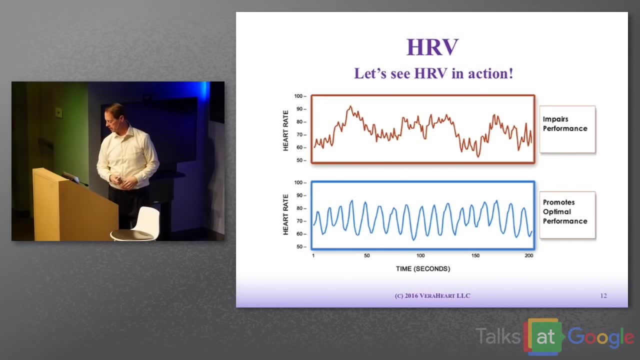 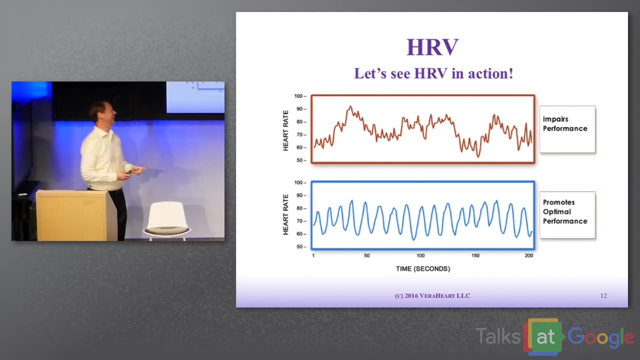 may be sitting in front of an audience, It might be a phone call that you're on or a phone call you have to make. Anything that could, or an in-law. something would cause you to have this kind of erratic pattern. Why is Daniel laughing? We'll talk later. So this erratic pattern here. 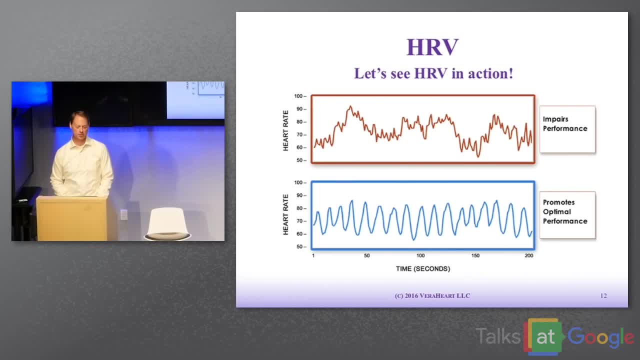 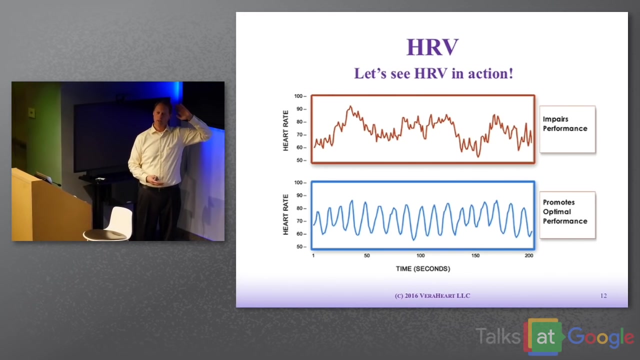 impairs performance. In fact, it greatly impairs performance. It is a huge indicator of confusion, of depleting energy in particular that we talked about before. It's an indicator of even impaired judgment, lack of communication. A whole lot of factors have been tested, measured and they indicate a lot of times why teams have 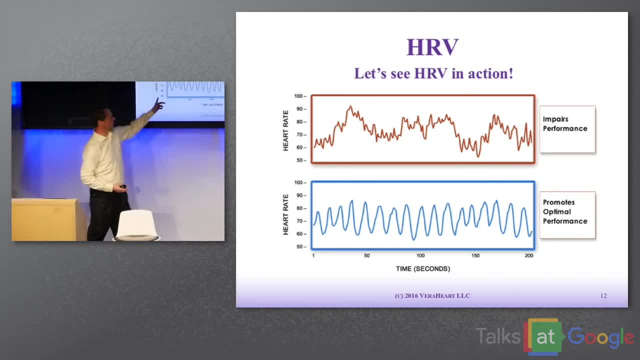 problems in working together too, as opposed to establishing this kind of more sine wave pattern where you can reach optimal performance. And the thing that, VeriHeart we're doing right now is we're teaming up with some of our coaches and consultants, teaming up with others, to begin. 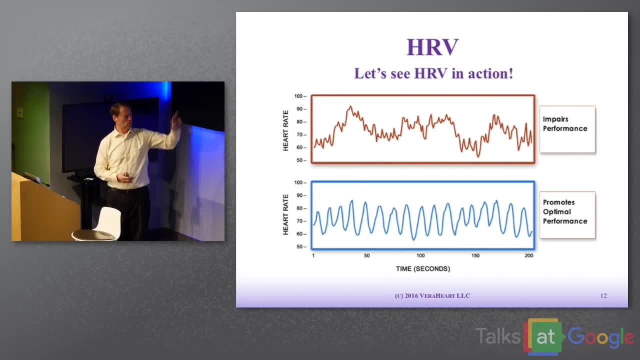 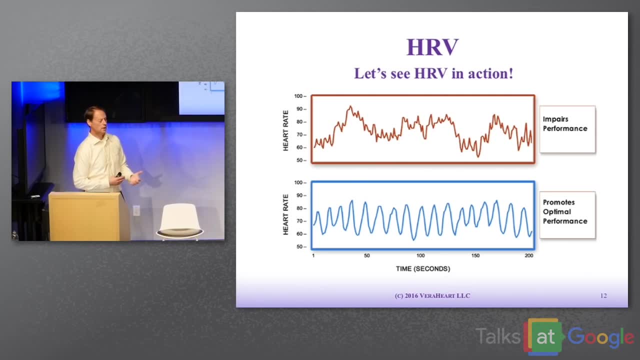 working with companies And we're doing a lot of work on that- And we're doing a lot of work on these teams and companies to shift them out of there into this and measure the difference in achievement in terms of what their goals are, And also happiness at work, being able to be more. 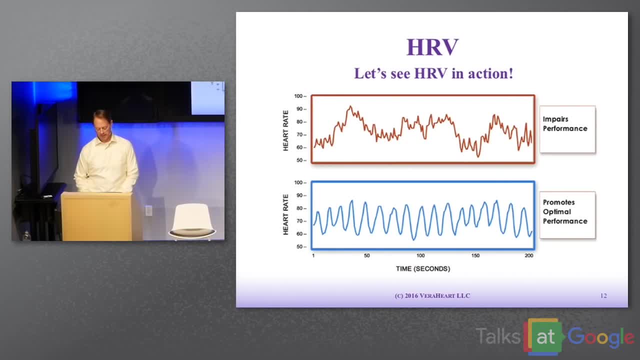 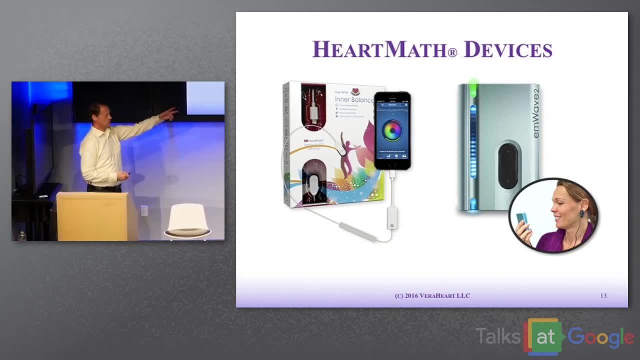 fulfilled at work, express their values and so on. A lot of different factors. So that's what we're doing with heart rate variability with our people. This is the devices that are held up and shared. They're available through VeriHeart or directly from Institute of HeartMath. 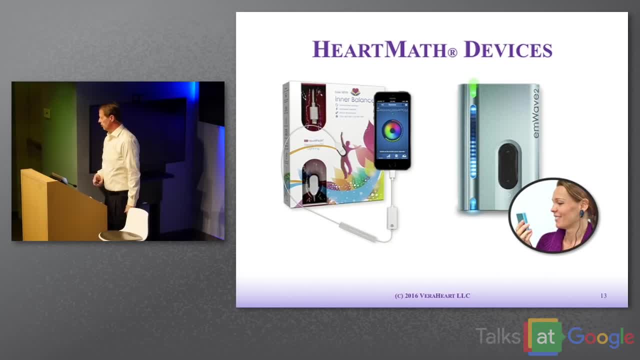 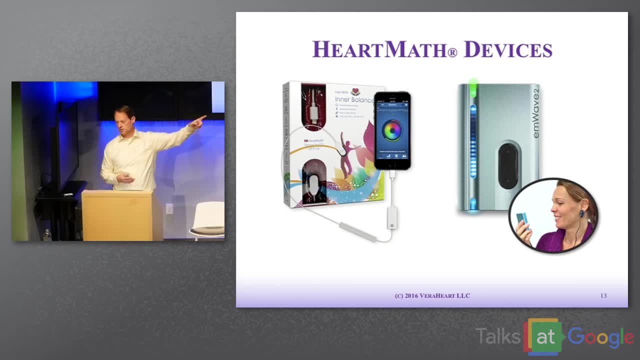 They run. $129 to $199 are the prices. They're very affordable devices. These devices have been out- The M-Wave has been over 10 years and it's gone through a generation of change. The iOS version of this interbalance and the Droid versions coming out are newer but they fundamentally are using the 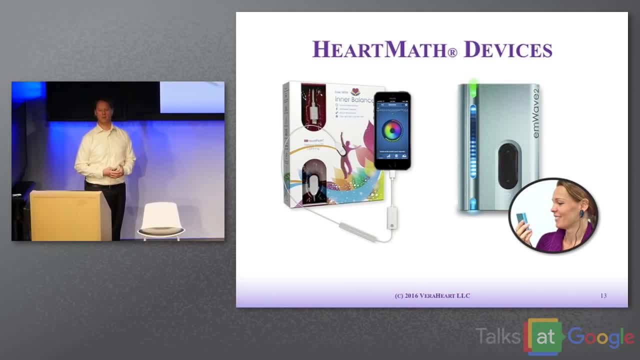 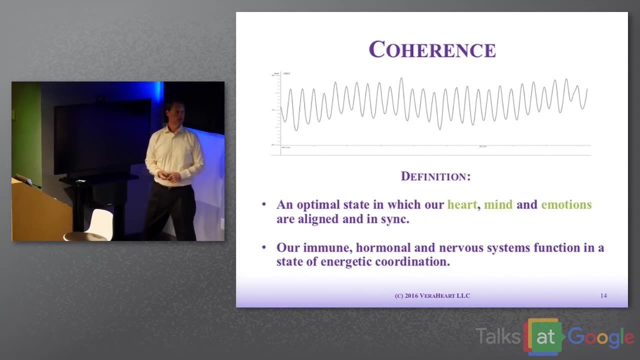 same proven, tested algorithms, same kind of tools to be able to continue to build more coherence and resilience. So let's talk about those now, because I've been hinting around to them for a little bit. Coherence, Full disclosure: that's my sine wave up there. That's my 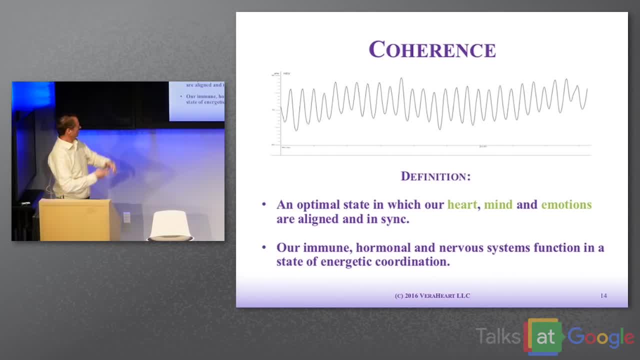 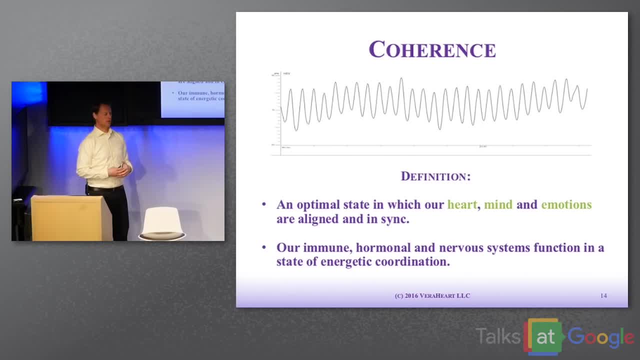 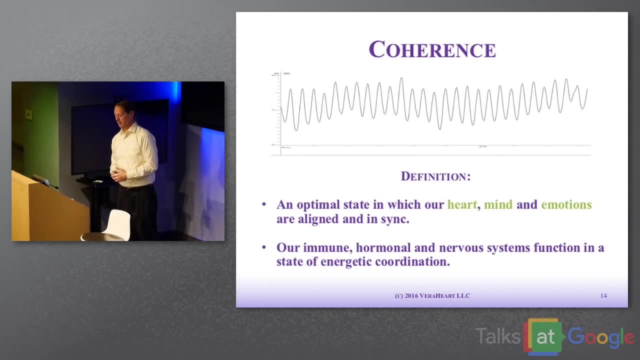 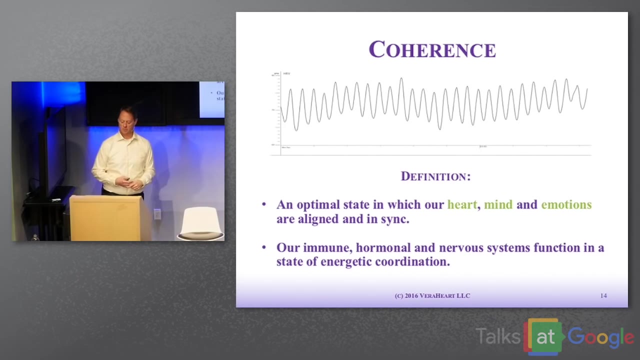 It didn't look like that at all. It couldn't have been that good at all. The coherence: What is this coherence? I have to admit emotional type of effects that were there, But now I'm able to jump into that kind of 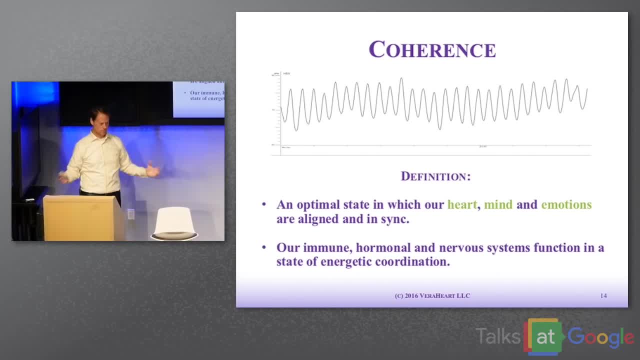 coherent place. What is coherence? It is defined as the optimal state in which heart, mind and emotions are aligned and in sync and affect through auto atomic nervous system, through the messages from the heart, the effects that come from that there's greater synchronization and the heart and emotions much. 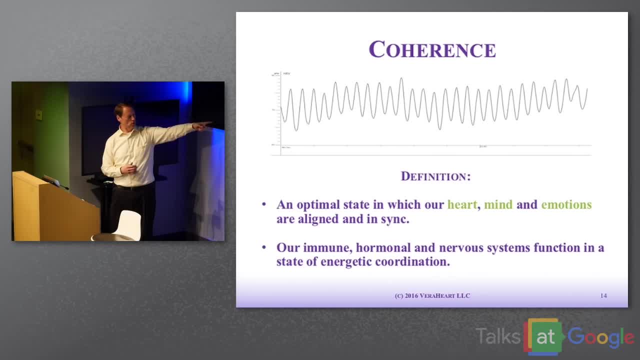 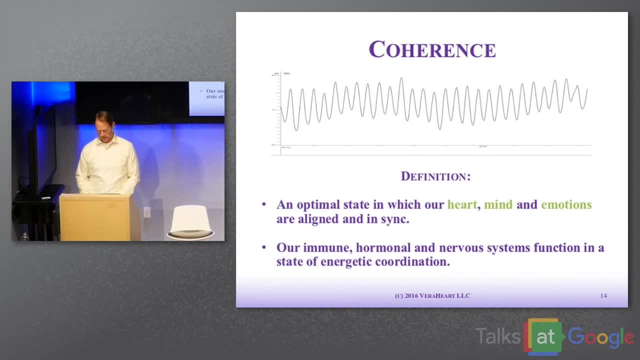 more involved in that process. our immune, hormonal nervous systems function in this energetic coordination. that's the definition of coherence. what it means is that we are more efficiently and more intelligently managing our human energy. so this is the magic. coherence is our ability to manage human energy, and it's represented in that sine wave. look, as opposed to the jagged. 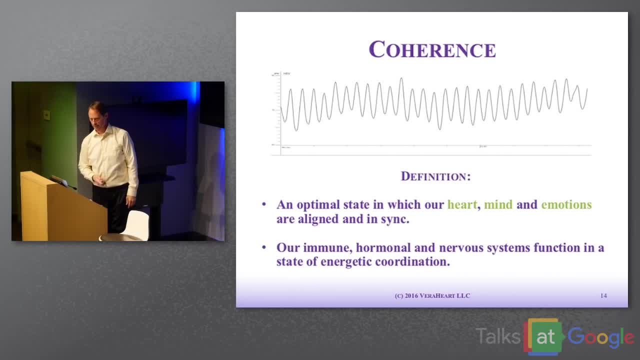 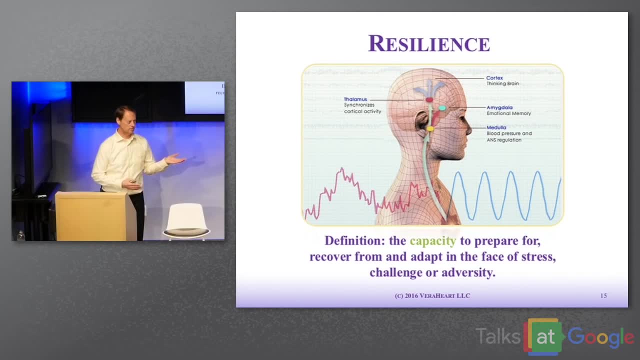 you know your incoherent type of rhythm. okay, then there's resilience. resilience now, with this knowledge of heart rate variability, the tools that you can use as well. resilience is ability to build your capacity for human energy: holding, reach, regenerating and then using your human energy. say that again: resilience is ability to build your capacity for human energy. so it's. 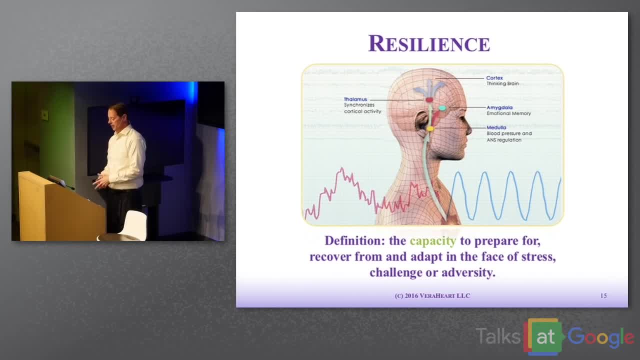 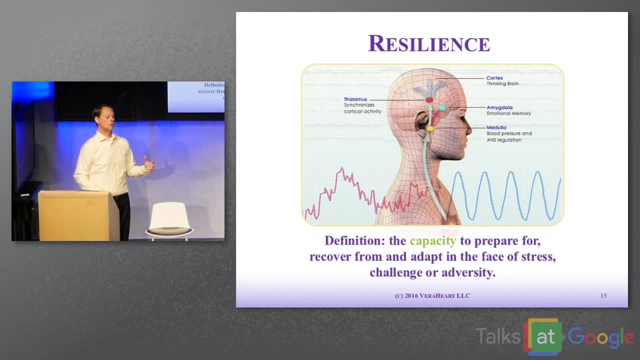 to prepare for, recover from and adapt in the face of stress, challenge, adversity. that resilience is that measure that when you're about to go into something that's going to be stressful, don't just walk right in. you take just a pause, just a few seconds even, can make a big difference. but 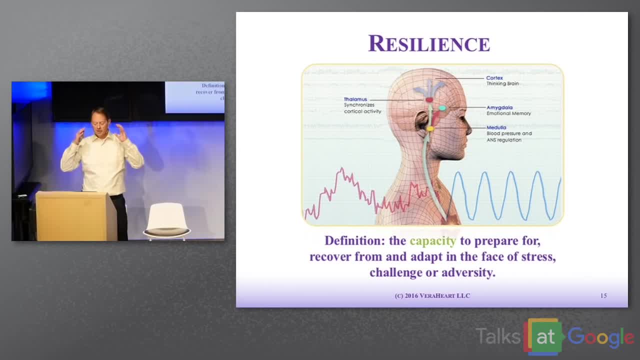 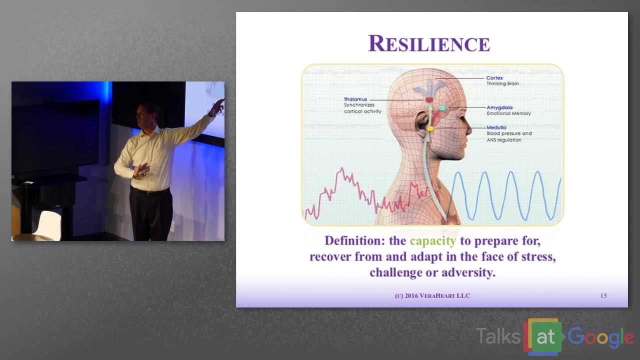 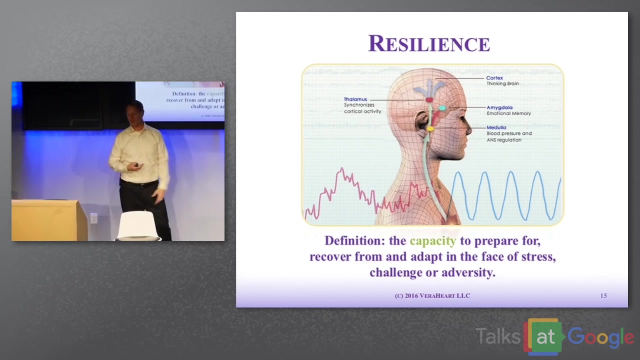 a few minutes can make a whole world of difference. you you can visualize going into a resilient pattern, moving from this erratic anticipation of what's going to happen. anticipation and emotions means you're releasing a flood of chemicals that are depleting you before you even go into your situation. you activate the heart mind connection, become more resilient. 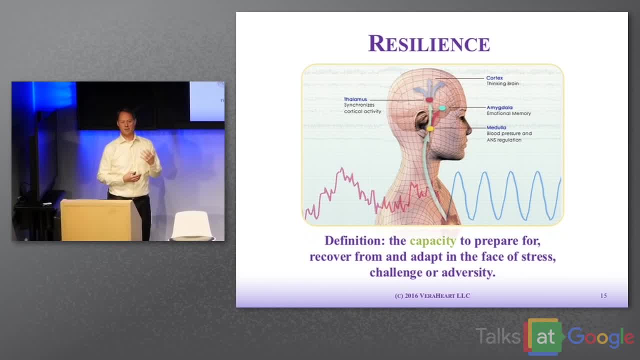 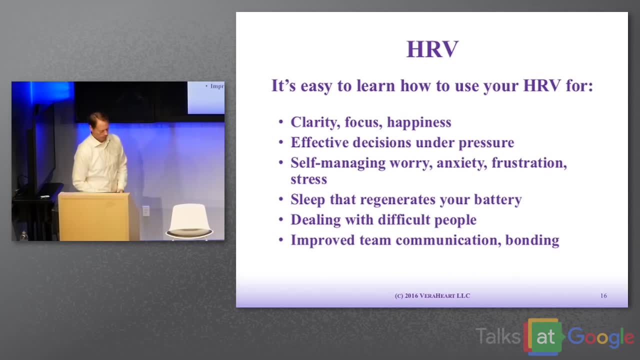 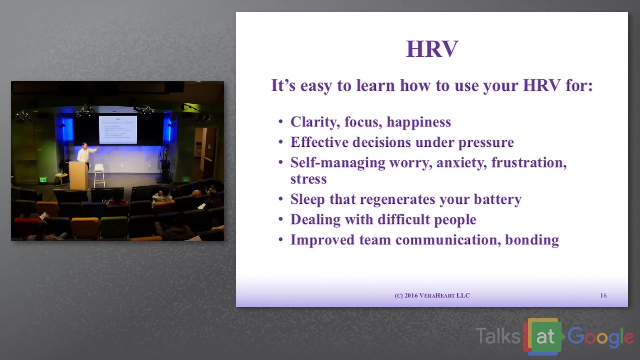 more coherent as well and you're going to be better prepared for whatever you're going into. so heart rate variability, then it is providing all these. I'll let you read those benefits, but fundamentally these come out of published peer-reviewed research. if you go to Google Scholar and look at heart, math is the lead research group for 20 years in heart mind. 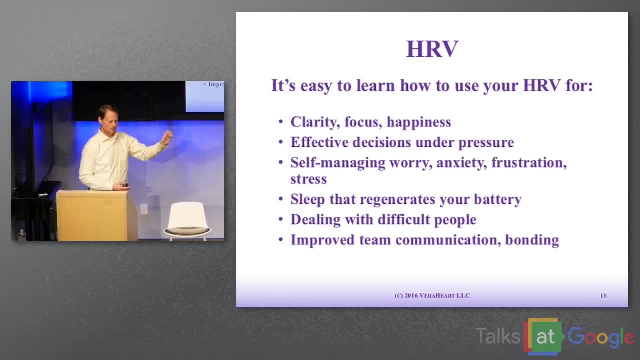 connection. the number of citations from other groups in them is is huge. there are 263 published pieces of work from Institute of HeartMath that are heavily cited. these are results out of a lot of these published works, the science that's been conducted behind and the practices. 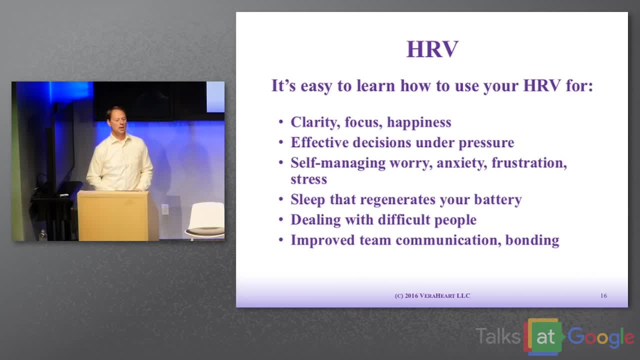 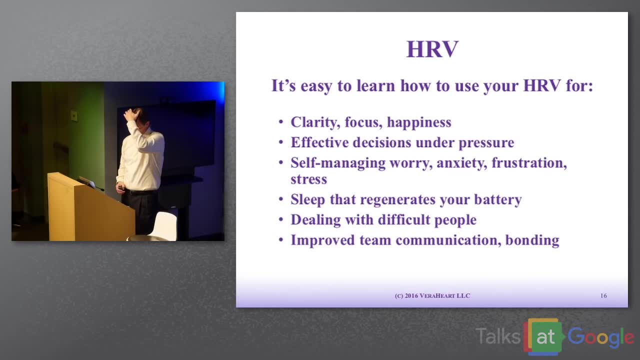 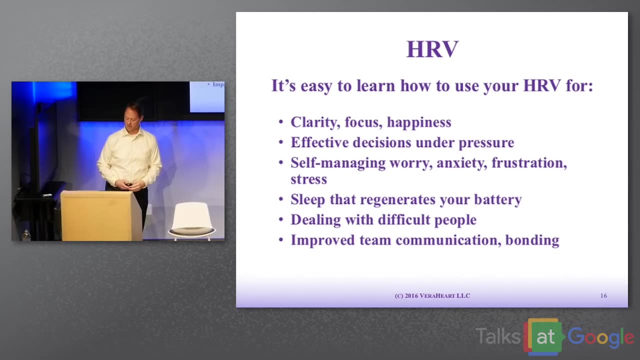 that have come out of Institute of HeartMath and the work we do to extend those practices to be able to share with you and with others. there's a paper. Roland McCarty is the the head of research for Institute for HeartMath. he has a fantastic paper that summarizes this and that I've talked about. but 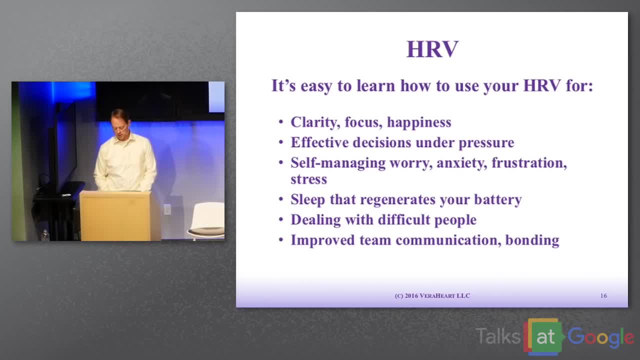 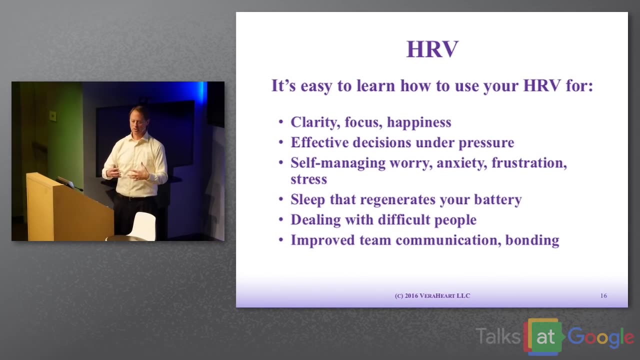 a whole lot more, and it's a consistent, heart-based, positive emotion techniques that that they're looking at show greater self-management, your ability to manage your energy system and better regulation of your physiology. even so- that's in my book- that means that we become more resilient. 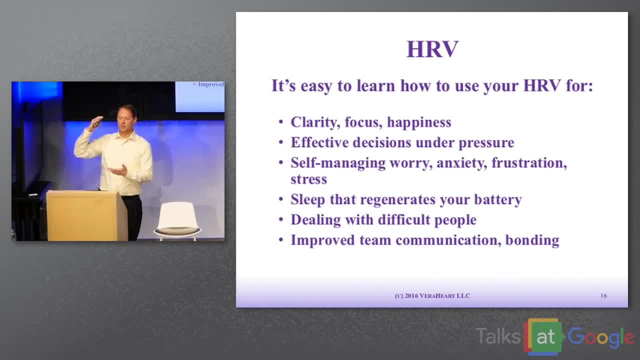 more healthy, more able to harness and and access our energy at a shorter amount of time. so that paper is called heart brain Neurodynamics, was published in 2015. so recently done a published piece and if you go to Google Scholar under HeartMath, you'll find that published there. when it really comes. 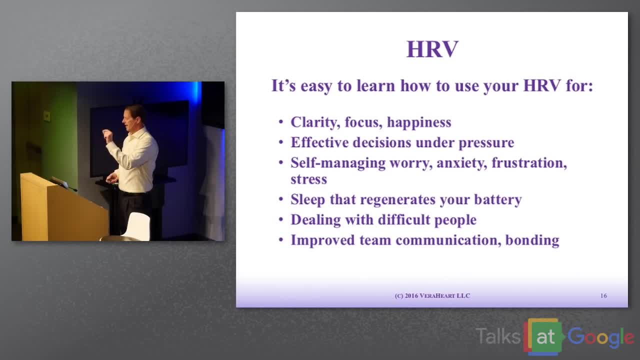 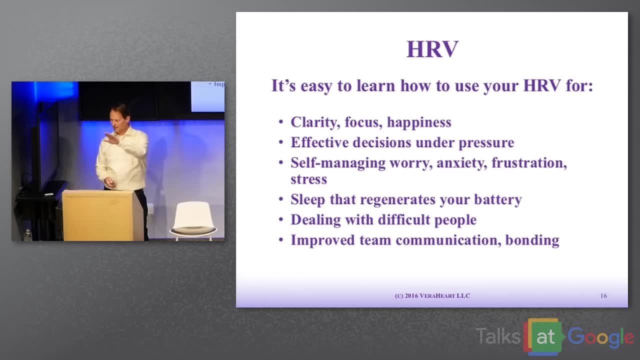 down to heart rate variability. if you just take five to ten minutes, uh, five times a week, practicing that same breathing that I just shared with you, you will have the effect of moving into more coherence and more resilience. it's even that little bit makes a huge, huge shift. now extend it. 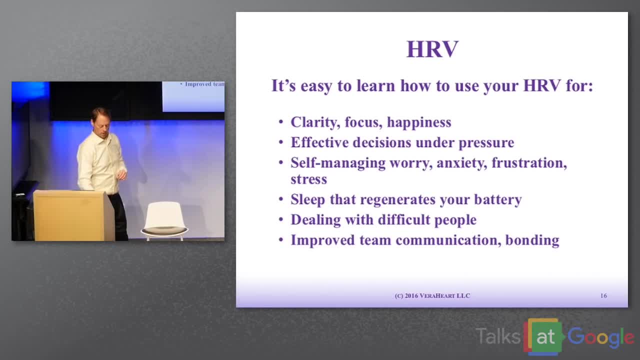 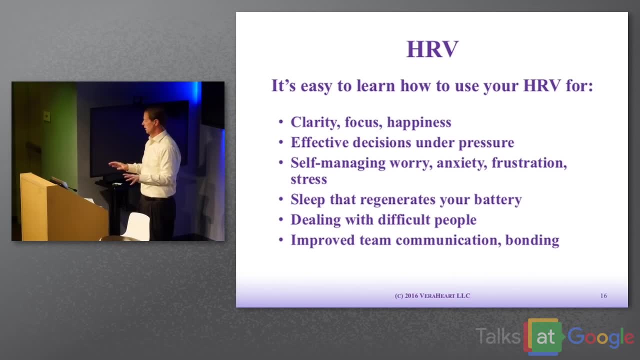 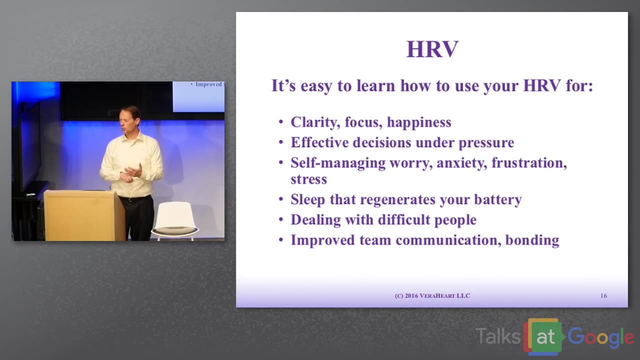 if you start your day. so what I did was, um, as I began working with these tools- and I've been heavily working with them for about a year, and then, six months ago, I shifted my whole morning. now, my morning was this: yep, what'd I do? my phone and began looking at the news. my email, social media, you know, got a company. 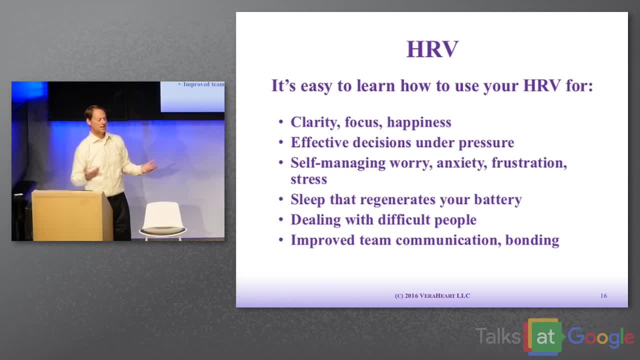 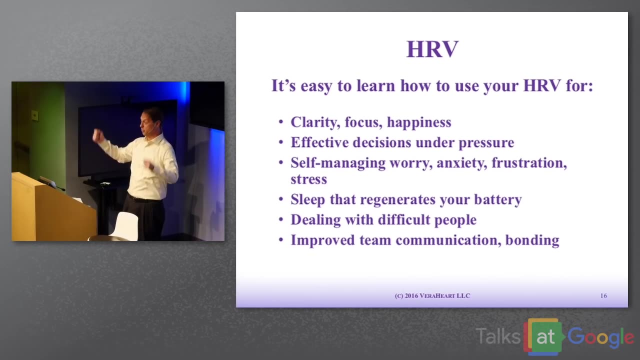 to run, I need to know what the pulse is in the morning, right. so at 6: 00 am I'm already feeding myself with um. admittedly, you know a whole stream of negative news, a whole bit of bunch of challenges that come in on email and maybe, and some good things too, but now I'm being rocked both ways. 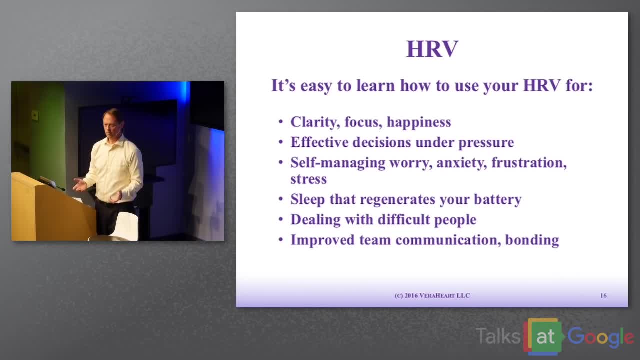 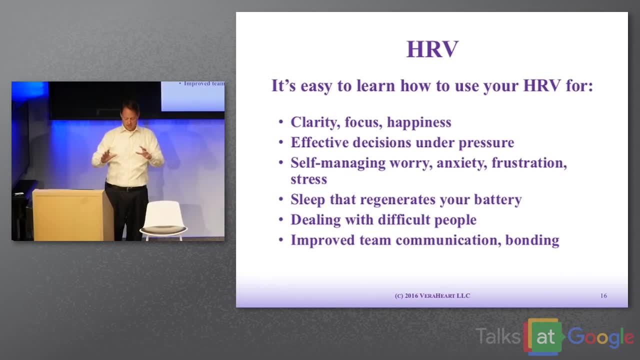 and I realized that that wasn't very mindful and it certainly wasn't heartful. I shifted my entire routine. now, when the first half hour starts- okay, I'm big admission here. yoga, all right. yoga is my way of life now. I mean I, I really have found the benefits of yoga now that yoga that starts out for 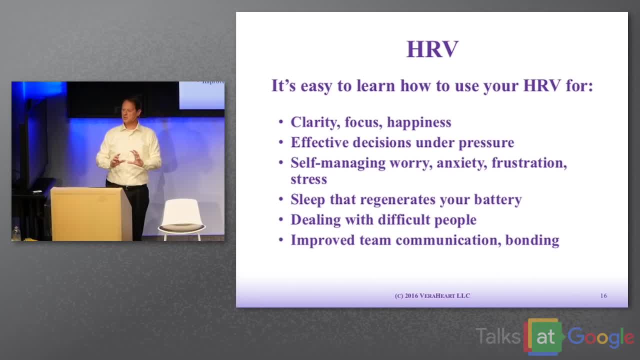 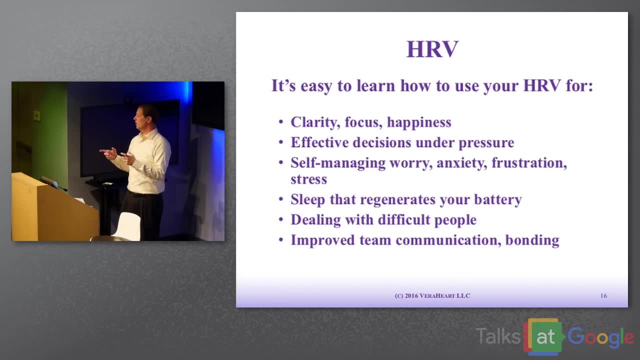 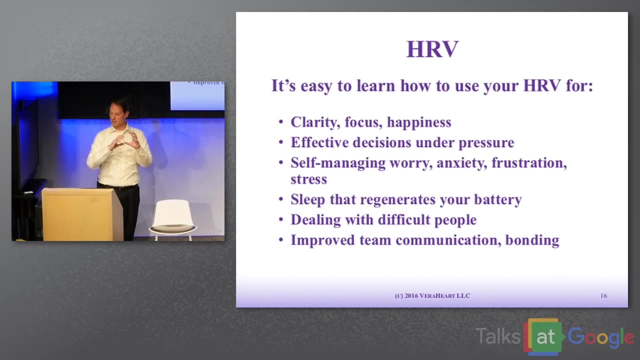 five minutes I go into my own mantra, my own meditation work to use this same tool here with people and in 30 minutes I've either established or re-established that coherent rhythm and greater resilience. when I've reached that level, I'm ready to get my day going. I'm a completely different. 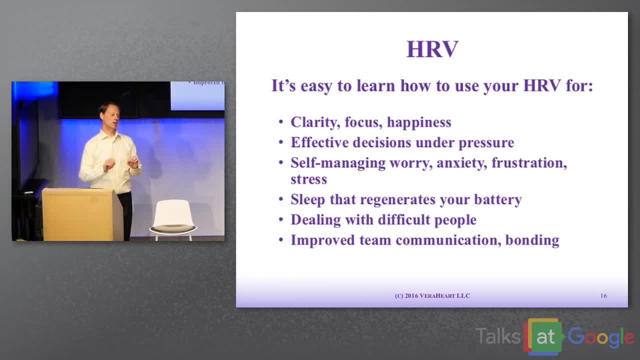 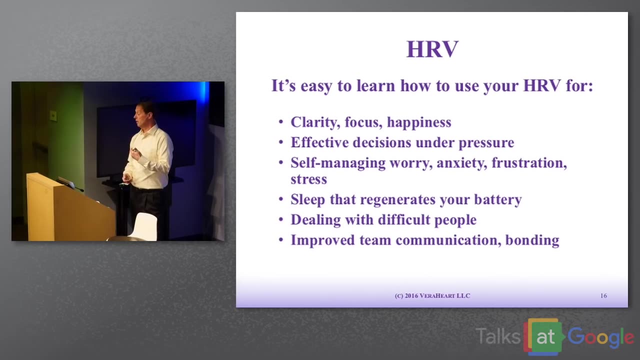 person. and that's six months of work, wasn't even? I mean, it was a month of establishing new habits and then maintaining that for another month, and it is just my habit. you could do that. it has a huge effect and a huge impact, but you can start and that. so that's the heart math part of this 10 minutes of my morning. 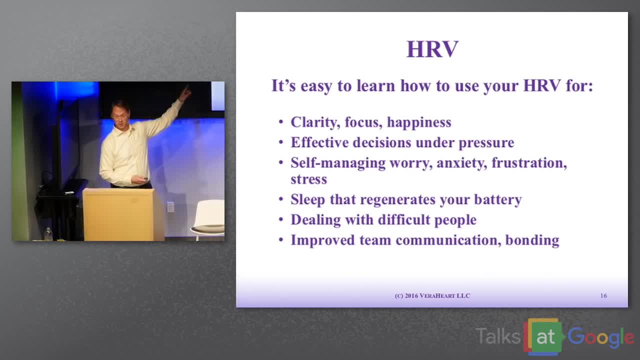 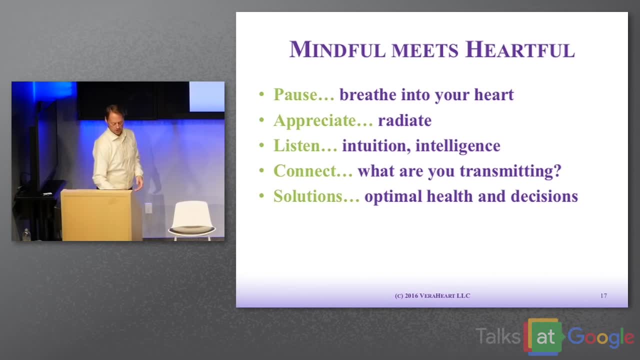 and I do that seven days a week. that's how I got that curve, by the way, that day to run okay. so, um, where mindfulness meets heartful, uh, the- I've mentioned a couple times pause, um, with their heart, one of the things we're- we've threatened to start a movement of pause for choice. 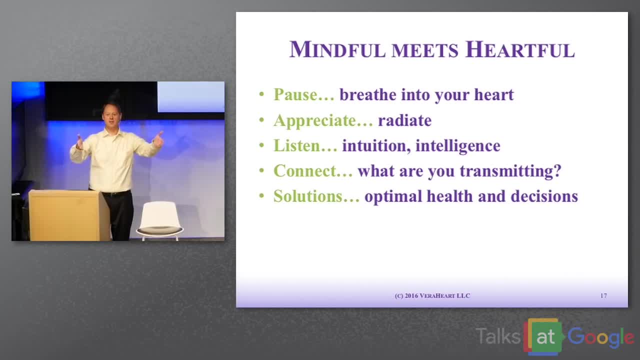 and I think we're going to do it. we'll get. we got the domain name, what you heard it here right now. pause for choicecom. we'll get it live within a week or two. the whole idea is this: I'm convinced, if this world inserted a pause, 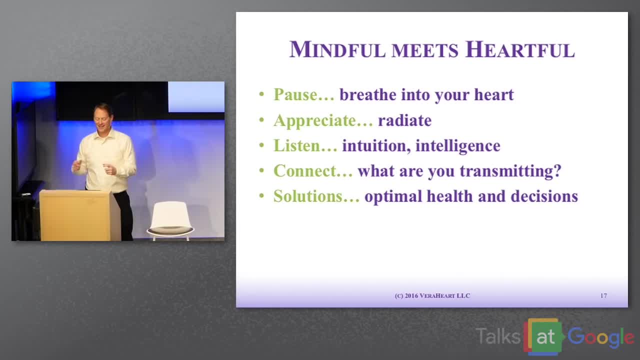 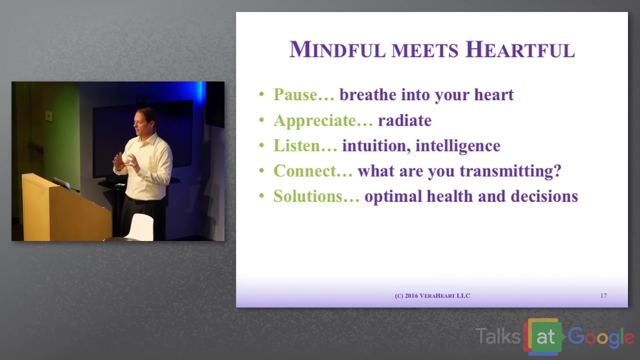 before speaking or acting and in any way, and that pause can be a few seconds to a few minutes, we'd have a completely different world. it allows us to have the heart, send a message to the brain to wake up, become more aware. mindfulness, pull ourselves in our center and full awareness, full attention and intention. and then we go about. 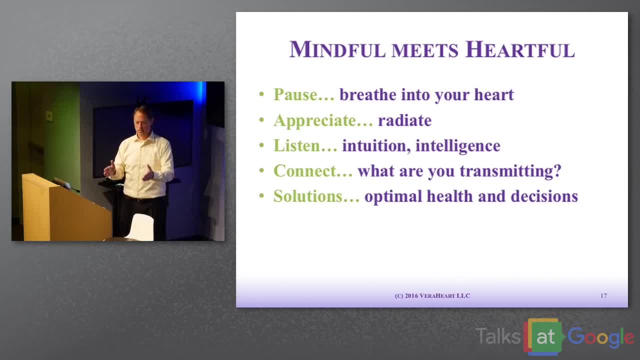 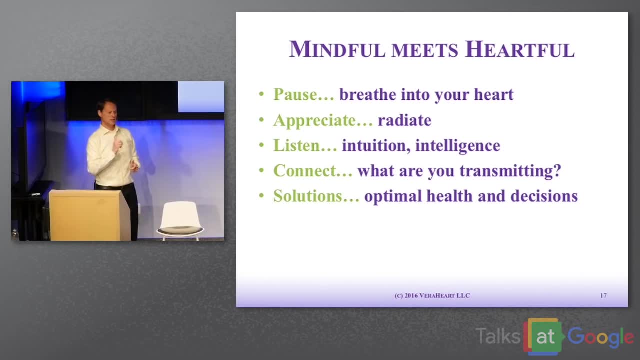 whatever we have to deal with, that golden pause shifts everything. we teach that to everybody. we work with, first thing foremost, pause, and the pause begins with even just one breath. it allows you to access so much more wisdom, so much more of your energy, your human energy. hashtag: human energy. 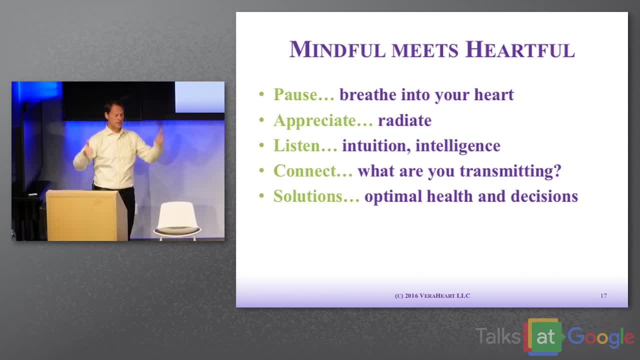 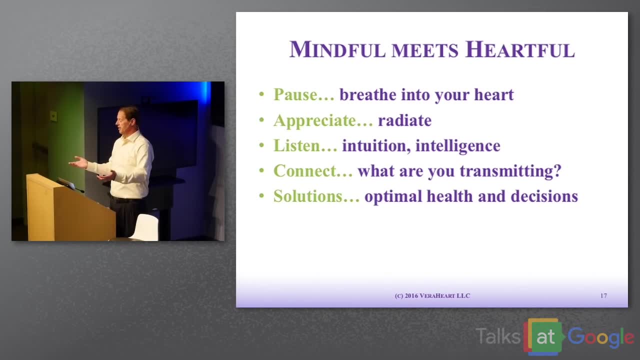 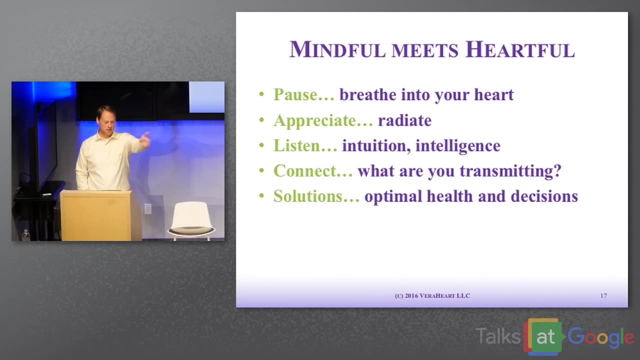 seriously, folks, within two weeks I want that hashtag like climbing way up, because it's nowhere right now. I had to. I had our team lunch like a bunch of hashtag human energies today because I wanted to use it here and it's nowhere. so if it goes somewhere, thank you. you all did it. 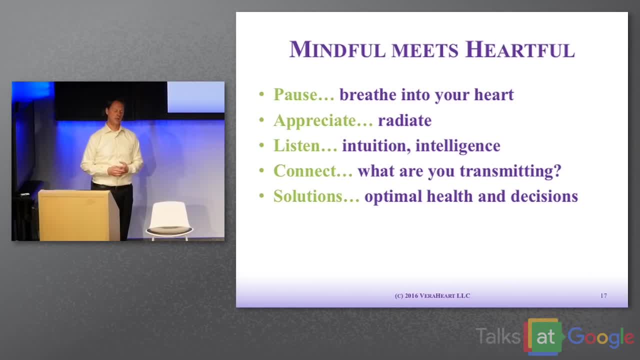 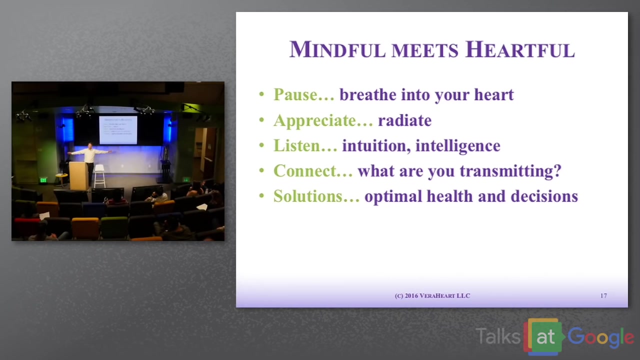 and it will so pause. number one: appreciate. so, when I I mentioned act, let your mind serve up a feeling of appreciation, care or compassion, um, that is, um accessing this appreciation. second step: now, here's the key. um, if you can radiate that- and so I use radiate three feet electromagnetic field, right, you've got that appreciation care. 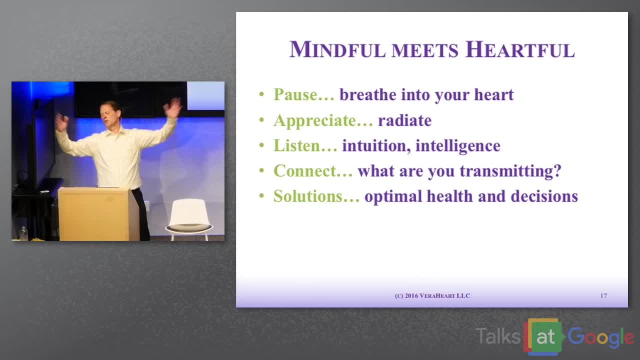 compassion, radiate it, send it in your field, let it go more than three feet. what the heck? have a joy, have a joyful time with it. that is mindfulness meeting heartfulness. third, listen, you have so much more aspiration, intelligence and wisdom that you have access to and and those who are in mindfulness. 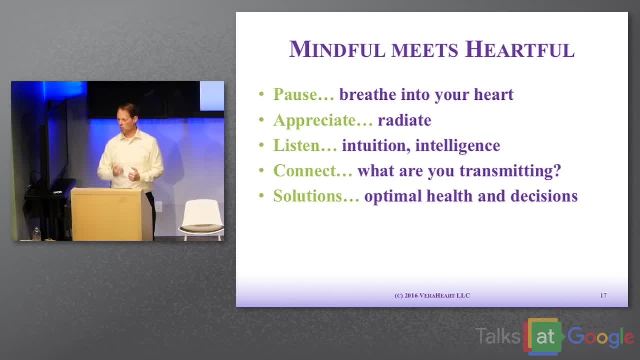 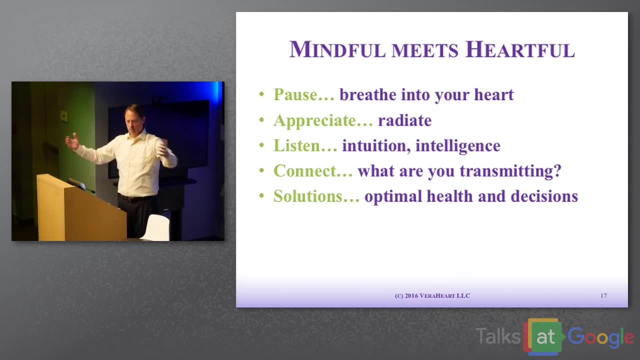 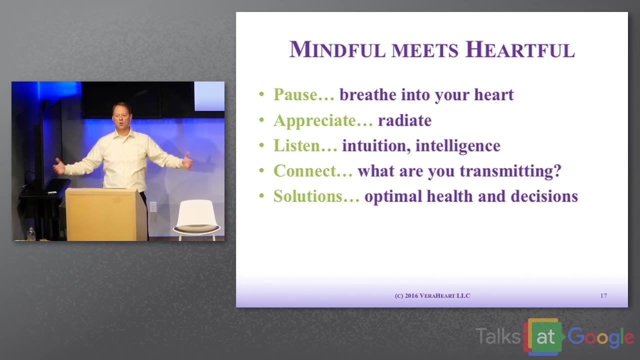 practices know that they access more. now bring the heart and more with some of these tools as well, and and even you go deeper and your senses begin to expand. we live a lot of life desensitized. there's so much coming at us all the time. let's re-open our senses and do that in a way that allows us to. 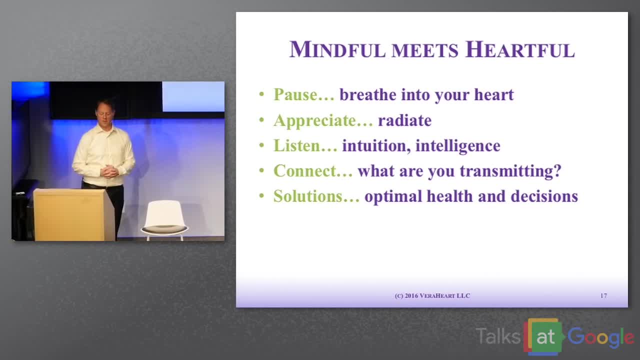 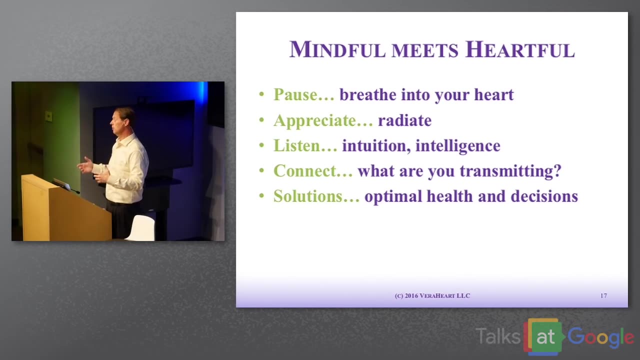 be heartful, and a good way to think in this electromagnetic field is the heart. math has a great way that they say: what are you putting in the field today? you know so. are you generating positive thoughts? are you generating things that help other? are you putting love in the field? are you, are you experiencing thoughts of? 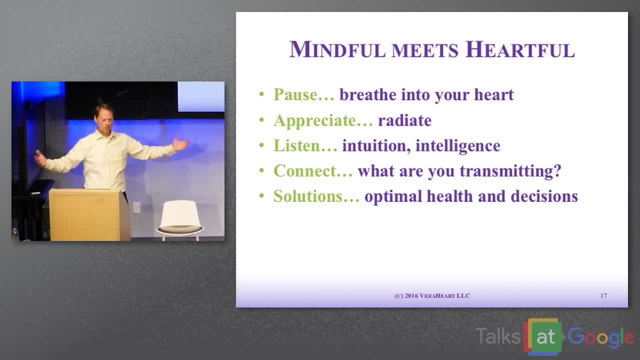 love or are you expressing love? is that coming out in your field? care, compassion, things that uplift people? you have the responsibility for your electromagnetic field. what are you going to put in it? what are you transmitting? and fourth is solutions. as we are listen, it's about results. it's 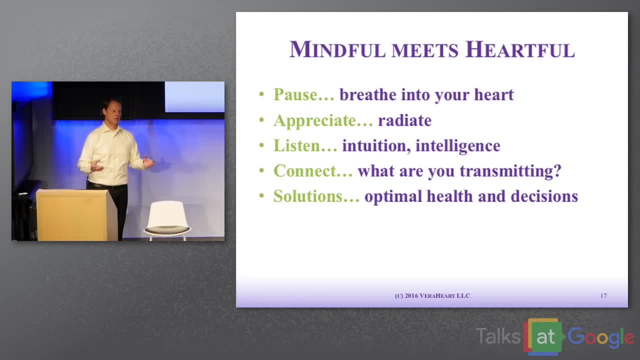 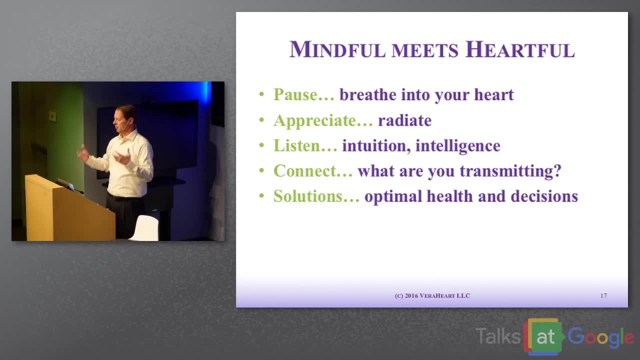 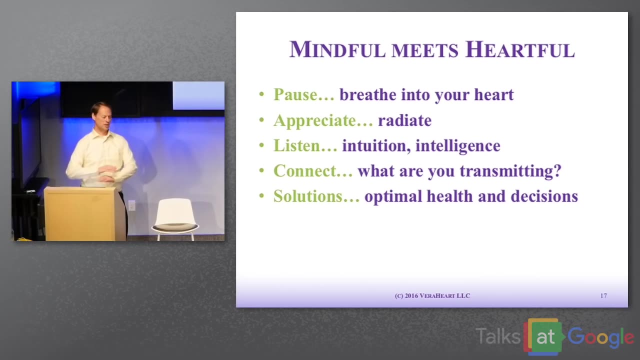 about achievement. we are in a world that respects achievement and results, and it should. we're not doing this just for you know joy and kicks. we're doing this because we've got a world that's going so fast and accelerating more. Moore's Law is not going to stop. I don't care how many people predicted over how many. 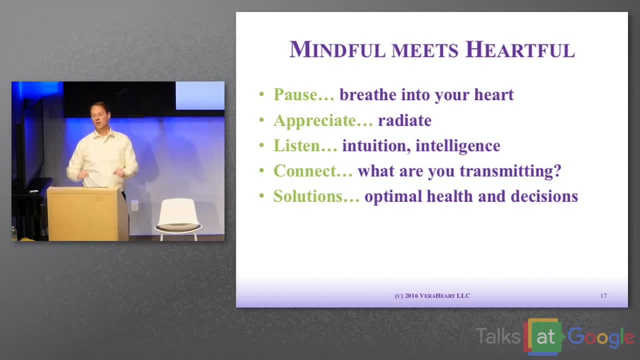 decades. it doesn't matter how many people predicted it over how many decades. it doesn't matter how many people predicted it over how many decades, it doesn't matter. stop. it won't stop, it's going to keep going. we're going to have things continue to accelerate, not just with technology and information, but in the 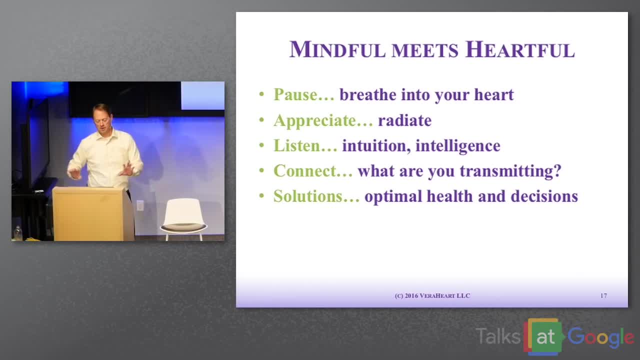 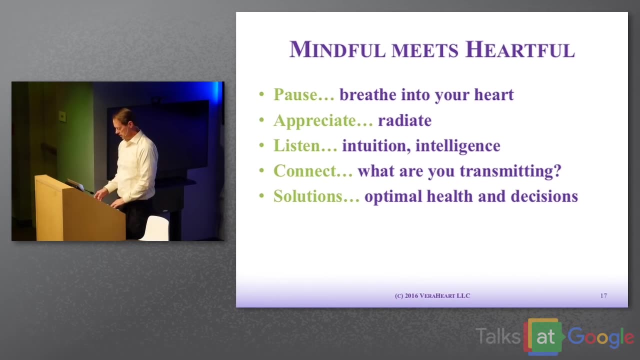 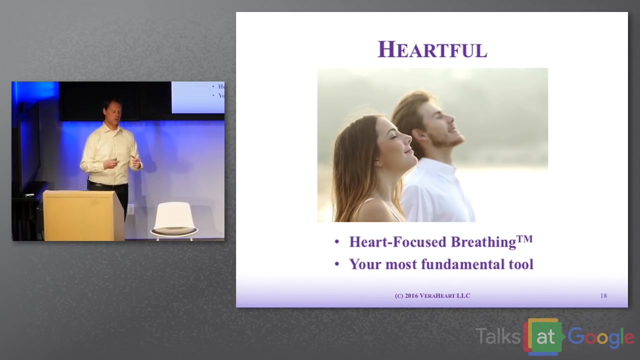 area of this new spaces, our senses, our ability to sense more, our ability to be more in touch with others through our field, and so solutions can come. and the and personal health, but also in smarter decisions and more results that get more done. so heart focused, breathing. remember that when we do training, we- that is the base. 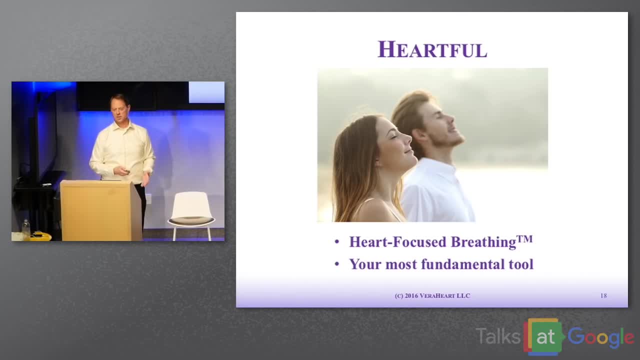 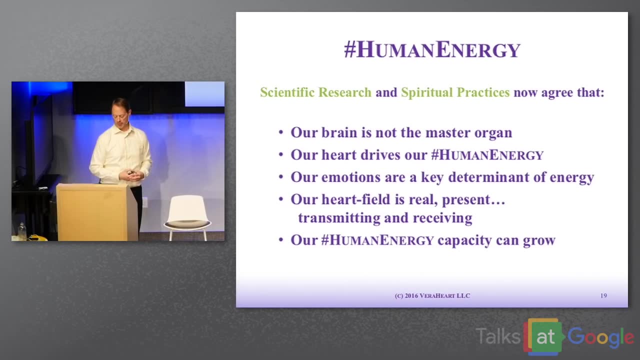 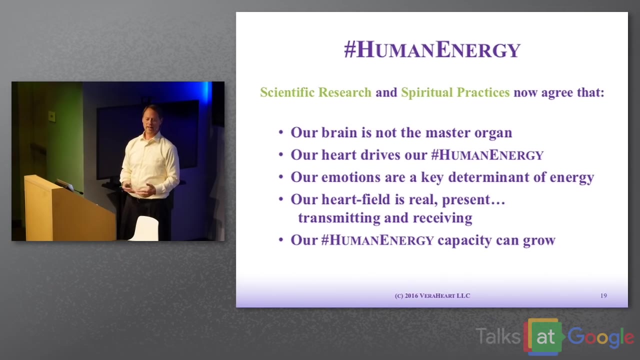 so heart focused, breathing. remember that when we do training, we. that is the base tool, the one that I shared with you. you can continue using that and expand on it. that is the most fundamental tool and it creates the pause. so recapping, I kind of like this scientific research has finally collided with, you can call it. 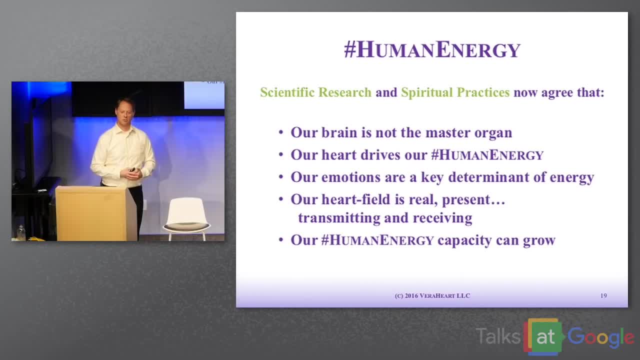 like this scientific research has finally collided with. you can call it spiritual practices. Greg Braden actually kind of created that kind of idea that we've brought these two together, and he's right. our brain was believed to be the master organ, and it's not the master organ, it's part of a system. 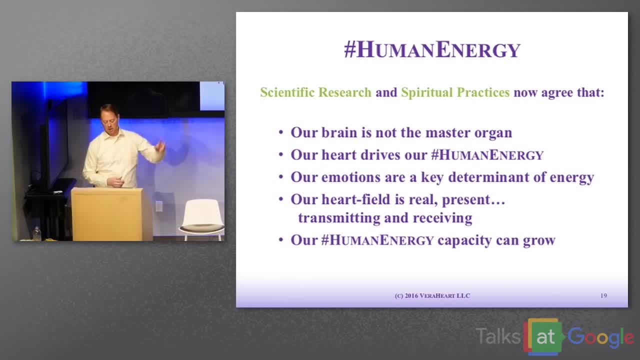 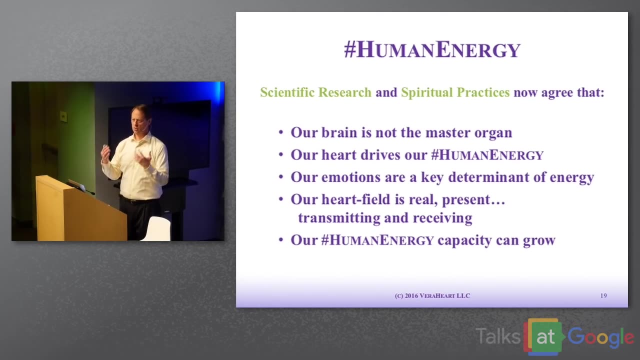 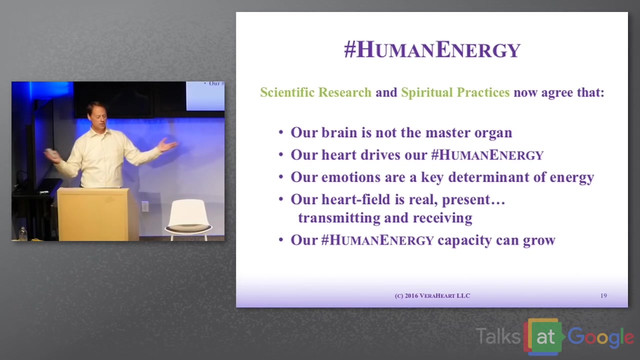 a distributed system that masters who we are. our heart drives our hashtag- human energy, and that recognition of the role of emotions is a key determinant of your energy depleting or renewing. once you have that in consciousness, you're already going to start increasing your human energy, increasing your personal energy. the heart field is present, it's real, it's measurable. 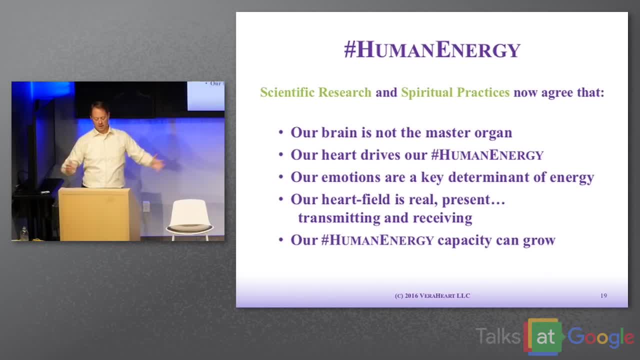 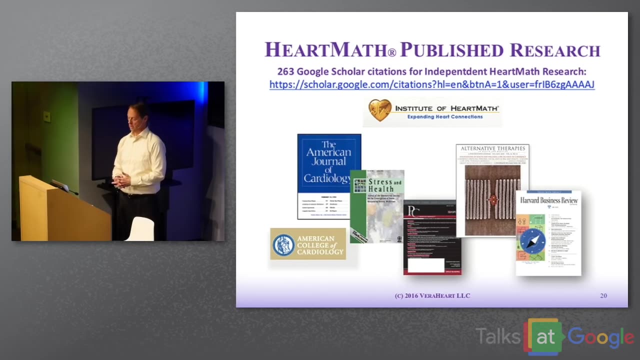 you're transmitting, receiving all day long, and our human energy capacity can grow. we can be more resilient, we can be more coherent. we are in control of being able to increase that published research. that's out there. you can. I encourage you to go look into heart math org, go to Google Scholar. look at the citations. 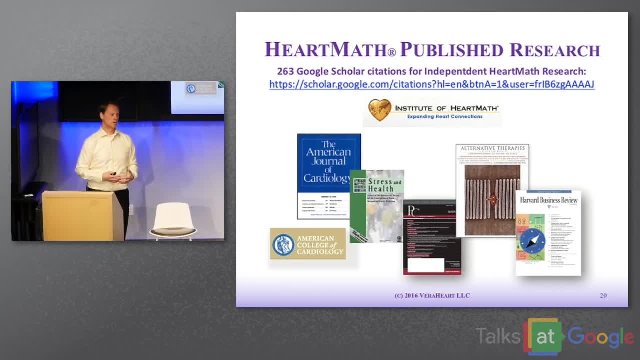 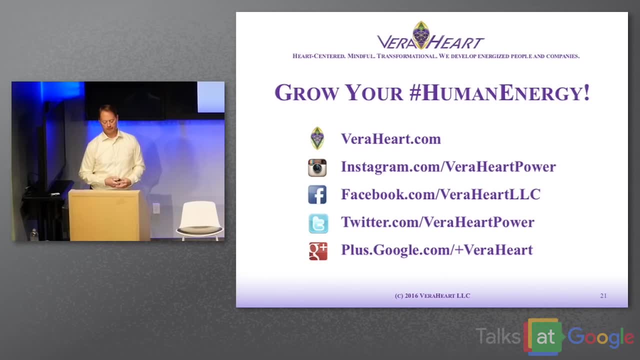 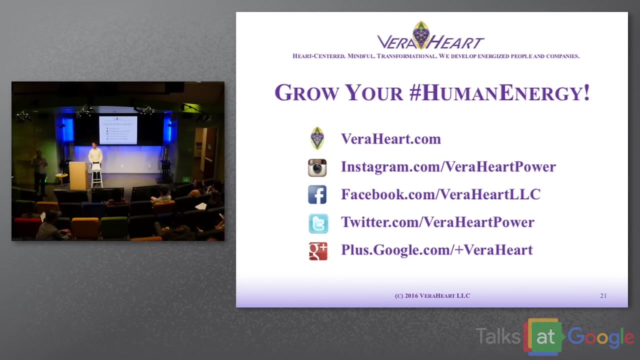 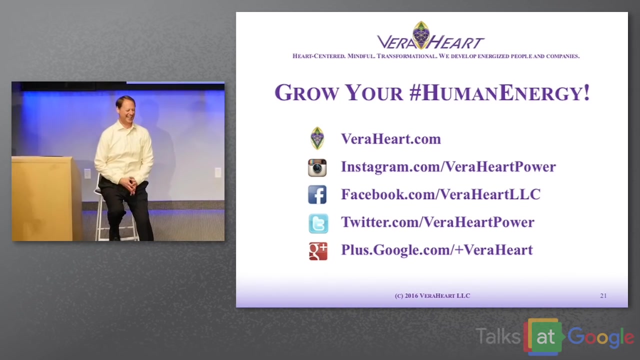 here. this, this peer-reviewed work, is fundamentally starting to take hold and launch and move forward. so thank you very much. I think we have a few minutes for questions. okay, you can make up a question. I'm curious about this heart field. I know that electric fields don't stop at a particular 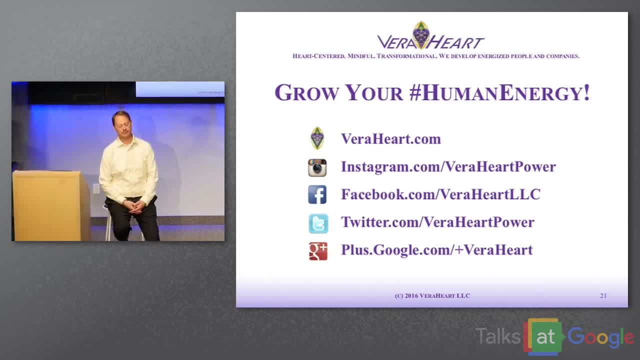 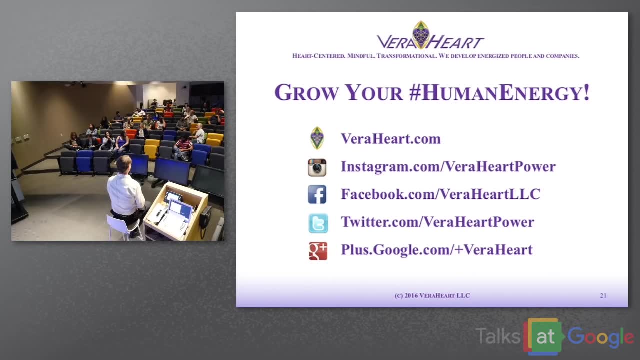 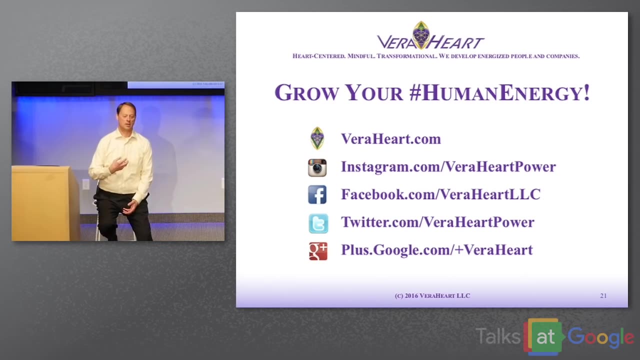 place. you talk three feet. what is what is? what is the heart field? is it a? is it the electromagnetic field coming out of the neurons? I'm sorry, what do you see when you actually measure it? I understand what you're measuring with the pulse. 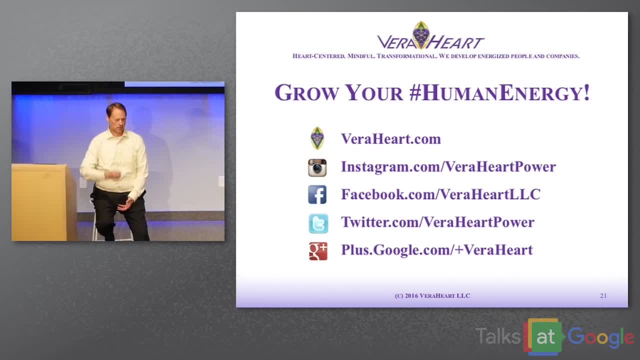 on the ear, but I don't understand what you mean by the heart field. It's a magnetometer. in this case, In hospitals I believe squibs are used, But what's happening is your heart. the way it pumps is through electrical signals: to pump and have 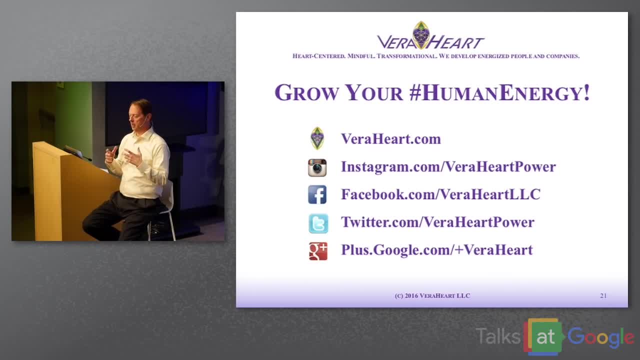 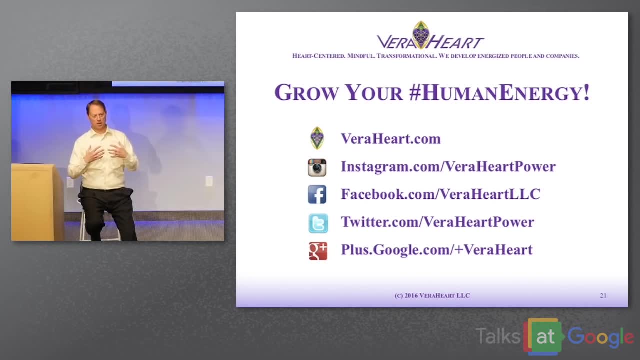 that rhythm that it's got. Anything that's electrical on and off creates a magnetic field, And so what you really are generating is the signals, for your heart are creating that magnetic field itself. Think of it. it's not really on-off, but that's the way I communicate sometimes. 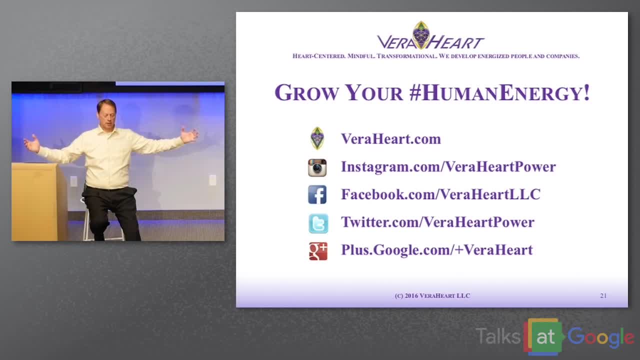 that boom boom, boom, boom, boom boom. That creates a measurable electronic field. Now the other thing that's interesting is your brain has electrical activity too. Anybody have any idea how big the electromagnetic field of the brain is? 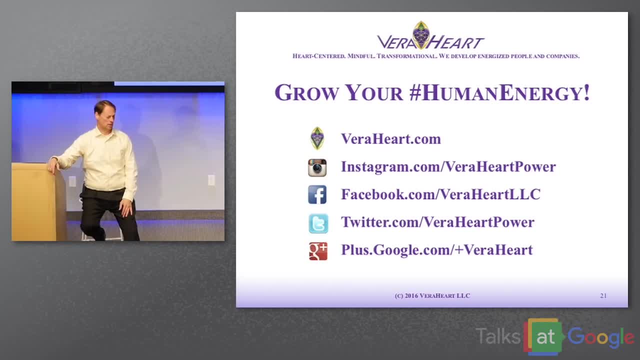 One to two inches. That's an astounding difference in power, the energy that's going on. So that is a real measurable electromagnetic field from that pulse. It's a pulse that creates your heartbeat. Okay, Did that answer your question all the way? 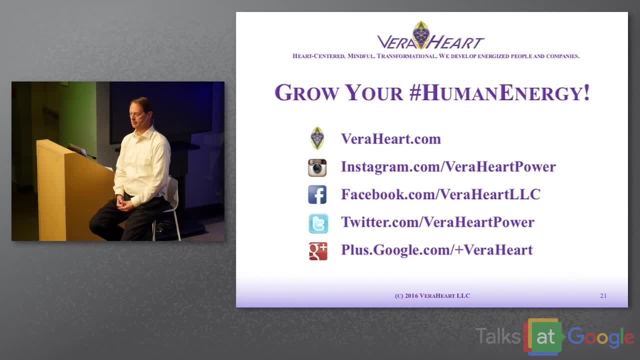 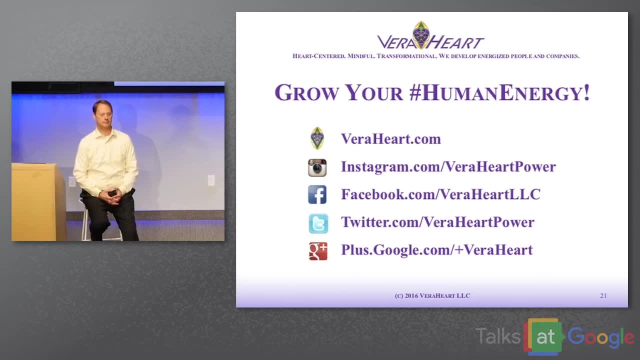 I understand how there is an electromagnetic field created whenever you have an alternated current in something, And in a previous job I worked with people who were using squid technology- superconducting something or others- to measure brain magneto-dynamics or something of the brain. 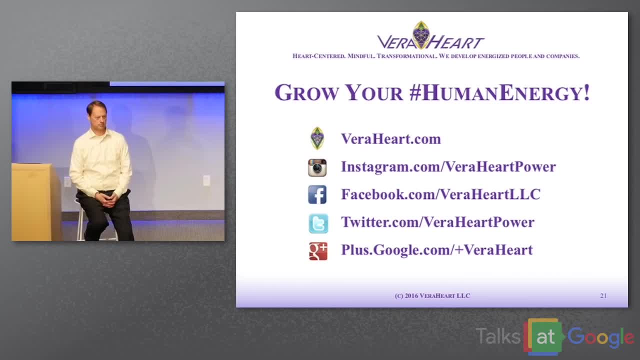 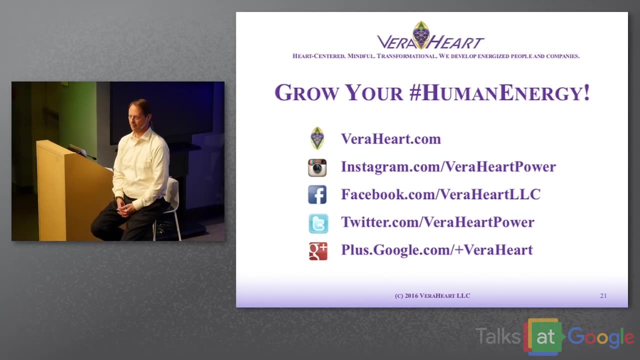 Okay. What I don't quite understand is- or another thing I'm a little uncertain about- is how you say that different people's heart fields interact. What is the receiving part of that? I understand how it's generated. What do you mean by receiving? 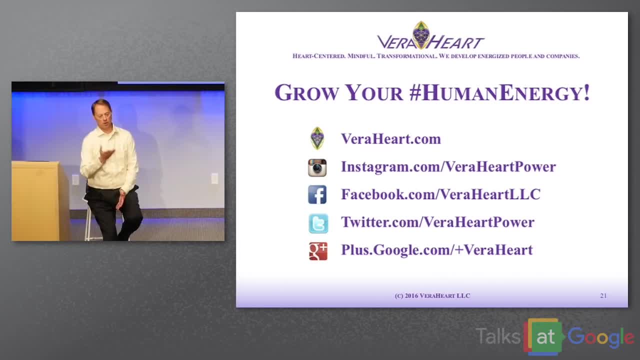 Yeah Well, the receiving side, the only way I can answer that. I'm not a neuroscience. actually I'm a neurocardiologist now who do this work. Okay, But they're measuring the receiving side of others' emotions or other fields as they interact. 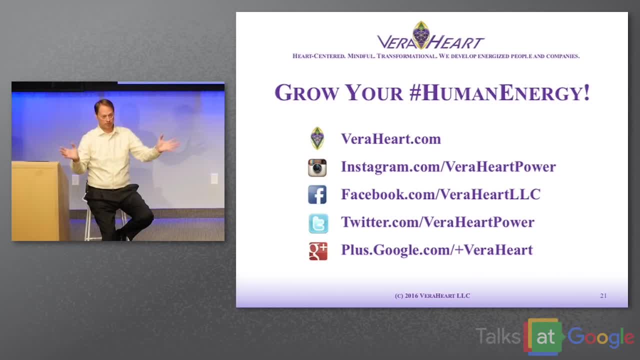 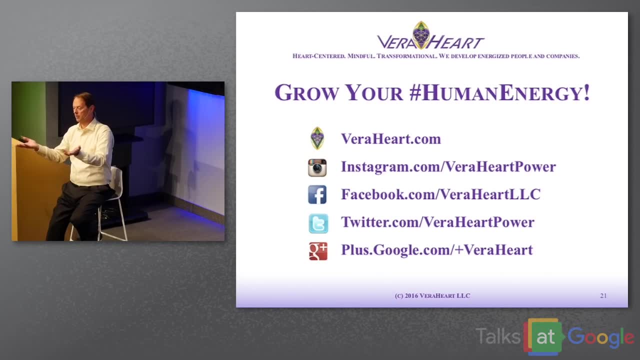 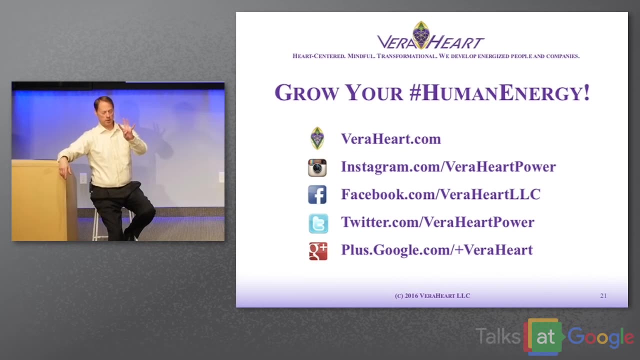 And so that can create a coherent field effect that's measurable, that there's an increase in a particular coherence of heart rhythms. So here's an example of measure: Four people, three of which do that heart-focused breathing. they've learned the technique. then they start doing it, and they start doing it to a certain degree. 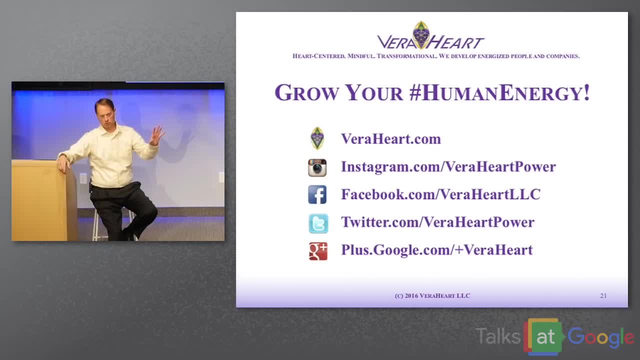 techniques to get a coherent rhythm. The fourth person: no experience, not even told. they're blind to what's going on. All get together. They're just at the table together, all four hooked up Somewhere, some number of minutes. I think it was six minutes, I don't remember exactly. 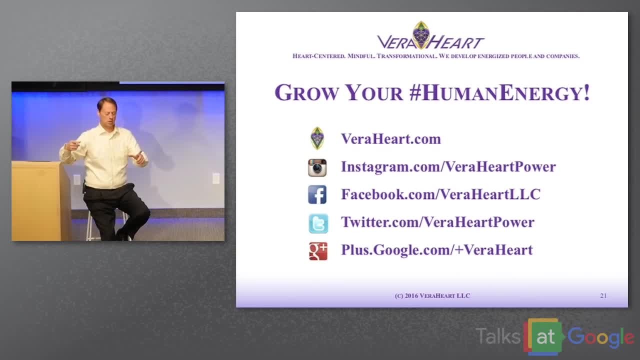 but some amount of time the data run. The three are cued to start doing heart-focused breathing- same thing you did. They establish coherent field with a very short amount, very, very short amount of time. The fourth person goes into coherence as well. They're not doing any breathing, They're 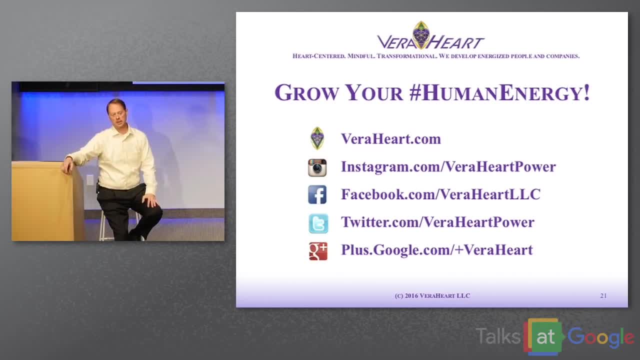 not doing any of these. They don't know the techniques, They're unconscious to it. They're receiving from the others. That's the best I can answer in terms of the science that's going on behind it. Thank you, We have time for maybe one more question. One more question. 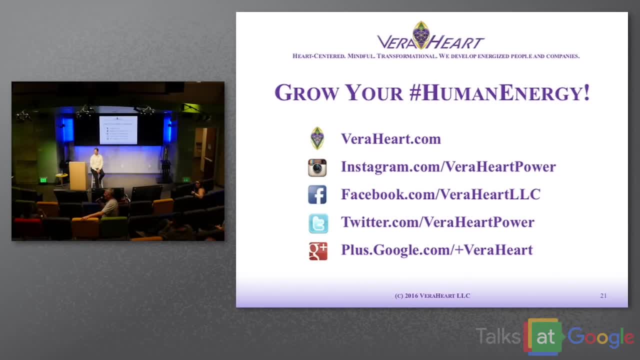 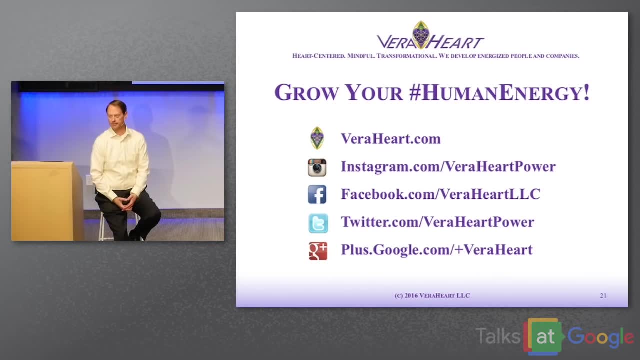 Or not? Oh, if you're, Oh one there. So I've never believed in people being able to see people's auras. but now that you've been saying that, do you think it's possible that people can see others' auras? 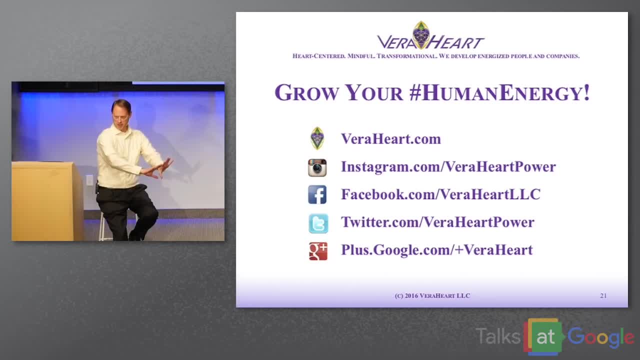 Well, that's a question completely different from what I was addressing, but the answer is yes, I do believe, and I think there's other things that are going on. There's other intuitive senses, other tools that we have that are. they're not part of what I was covering, but, yes, I do believe that. 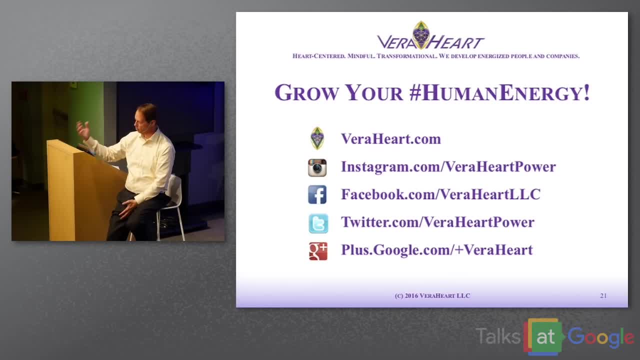 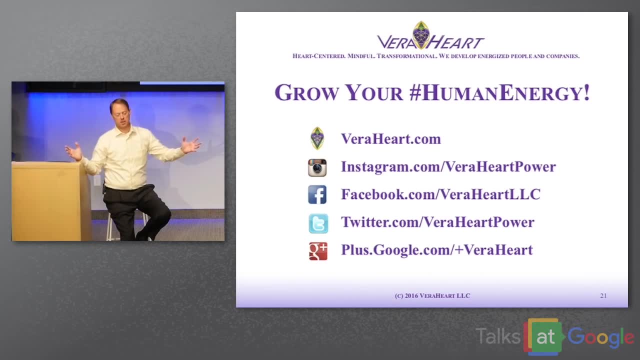 is the case, and I think that's the case. That's a whole area that's opening up more, which is just fascinating, because when we talk about the bigger topic of energy, I mean listen, we're all just energy. I mean, you know, matter is just. 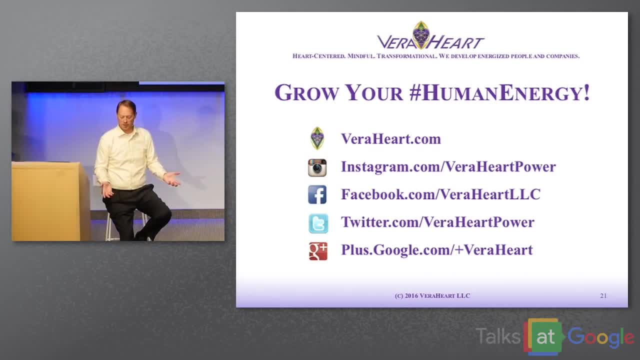 the placement of the potential of energy at any time. We know that from quantum side. So, yeah, I believe a lot more is going to be discovered. That's awesome, Thank you. Yeah, we could have a lot of good fun with that. So unfortunately we have to wrap up today's talk. 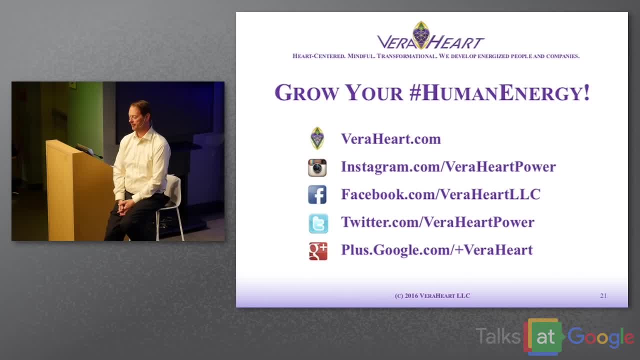 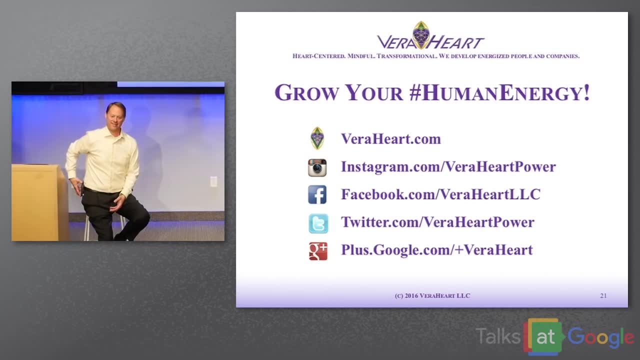 staying here for lunch. We're going to be going to Big Table, so if anyone has a question they were too shy to bring up here- they could bring it to lunch with us. So thank you for coming out, everyone, and thank you, Lane. Thank you so much.